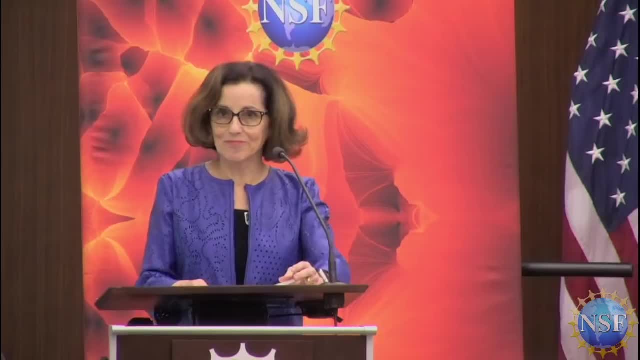 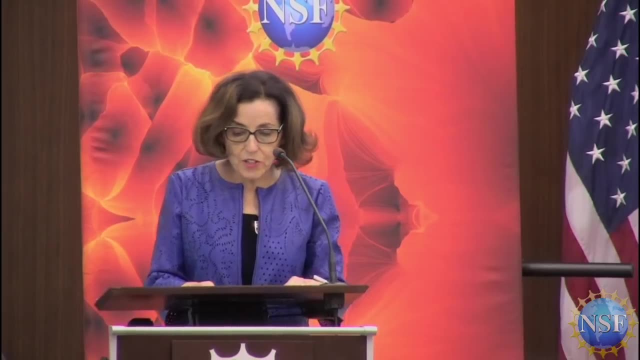 Foundation, the place where discoveries begin. In 1912, physicist Victor Hess had a problem. He was trying to find the source of a particular kind of ionizing radiation that he believed came from space, But he was just too close to the ground. So Hess did what scientists and 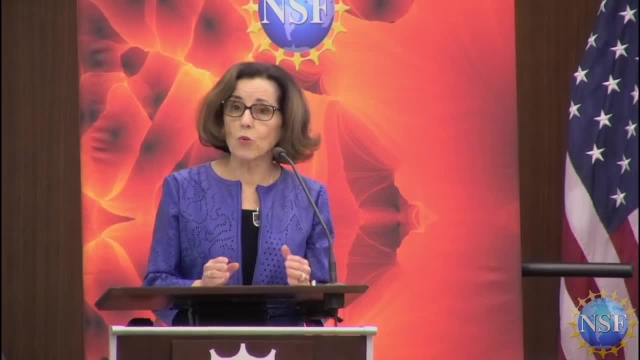 engineers have done throughout history. He devised a way to collect the information that he needed. Accompanied by what must have been some very patient friends, he began two years worth of balloon ascents, taking electroscope measurements far above the ground, Just nine years after the Wright brothers. 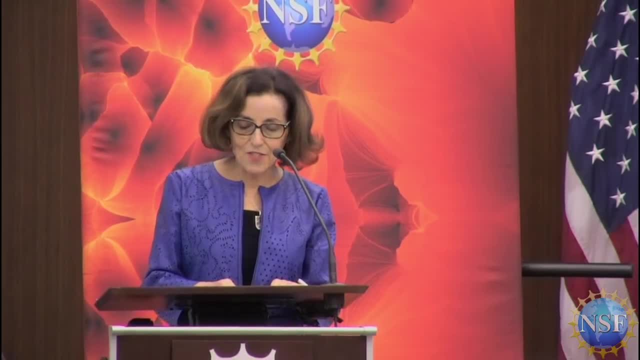 first flight in a small basket, 5,000 meters in the air, during a near total solar eclipse, Victor Hess found the first evidence of cosmic rays. For this discovery he was awarded the Nobel Prize. As so often happens in science, Hess's findings raised new questions, opening the door to a mystery that has endured. 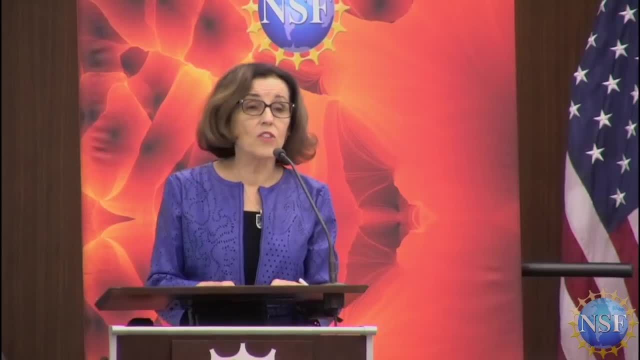 for more than a century. What are the origins of high-energy cosmic rays? In 2004, a group of researchers supported by the National Science Foundation also had a problem. They wanted to track high-energy neutrinos, elusive subatomic particles that travel the universe at almost the speed of light. High-energy neutrinos are incredibly hard to study. They have no electrical charge and are almost weightless, penetrating matter as they whiz across the cosmos. We can only see evidence of them when one happens to crash into the nucleus of an atom. If you had a detector the size of your body. 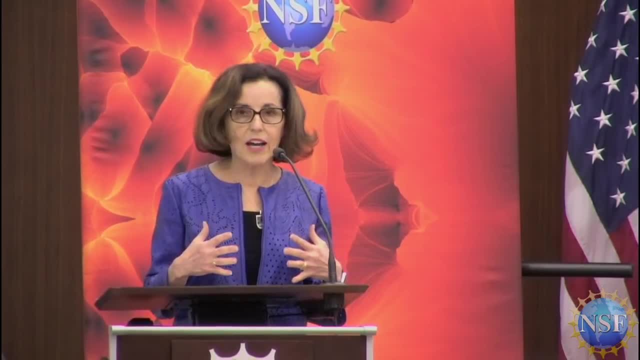 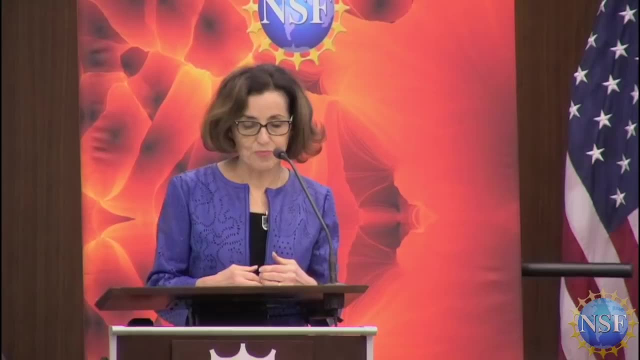 you might register a collision between a high-energy neutrino and a nucleus in your body only once every hundred thousand years. So, like Hess, these researchers devised a clever solution. They created a cutting-edge laboratory in Antarctica, one of the harshest environments on the planet and also the only. 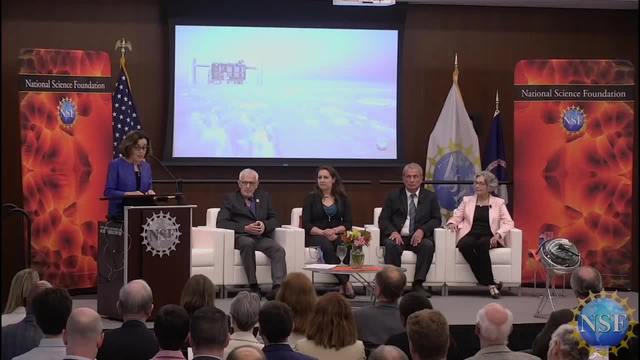 place suited to this task. They constructed, with NSF funding, the IceCube Neutrino Observatory, which sits above a cubic kilometer of clear crystal. This is the first observatory in the world to have an ice-cube neutrino observatory. This is the first observatory in the world to have an ice-cube neutrino observatory. 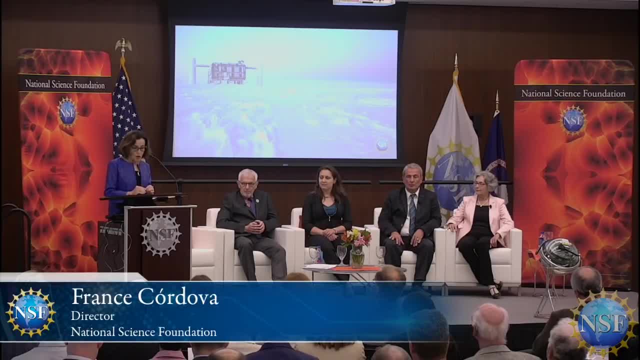 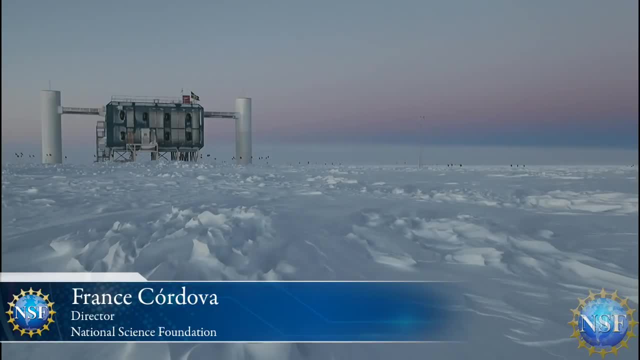 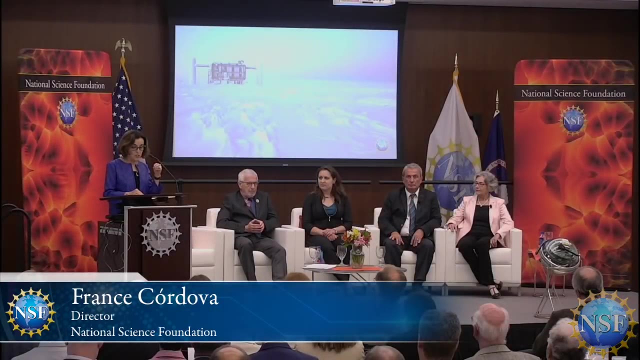 The ice-cube neutrino observatory is a crystal-clear ice that is permeated with over 80 long strings of sensitive equipment, a massive engineering undertaking. You can think of these strings like strings of pearls, in which every pearl is a digital optical monitor like the one on this stage, and there are over five thousand of them in. 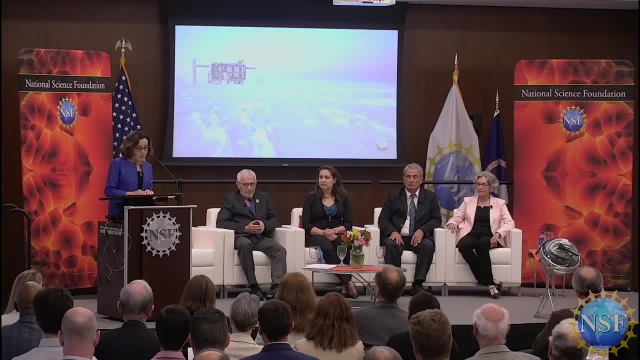 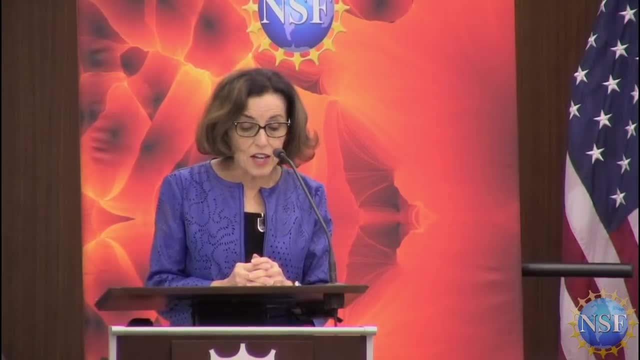 this cubic kilometer of ice, 3.5 billion cubits of ice. Today, I am proud to announce that, using data gathered by NSF's IceCube, an international coalition of scientists has taken a major step toward solving the high-energy cosmic ray mystery, echoing Hesse's spirit of innovation. 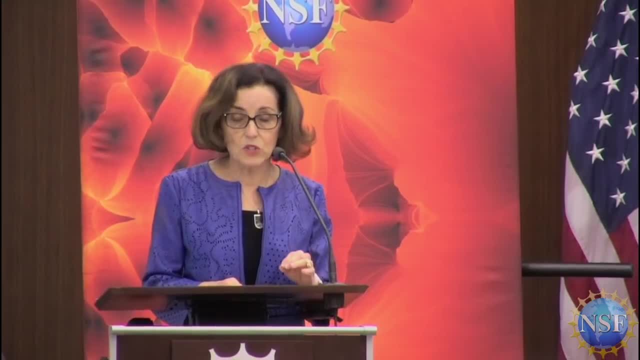 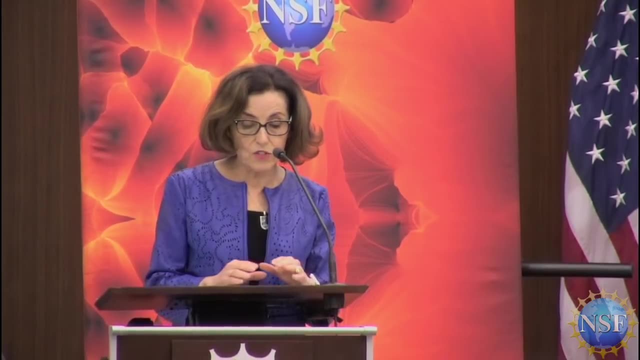 They believe they may have identified at least one source: another galaxy, billions of light-years away, with an especially active nucleus known as a blazar. Blazars are powered by supermassive black holes and spew immense jets of mass and energy that can be the size of a visible galaxy. 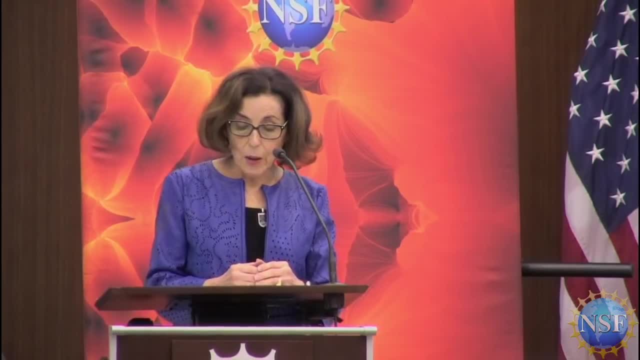 These jets accelerate cosmic rays and contain particle collisions that result in high-energy neutrinos And in all blazars. one of those jets points directly at us. This discovery will enhance our understanding about how the universe is built and behaves. We will better understand the nature. 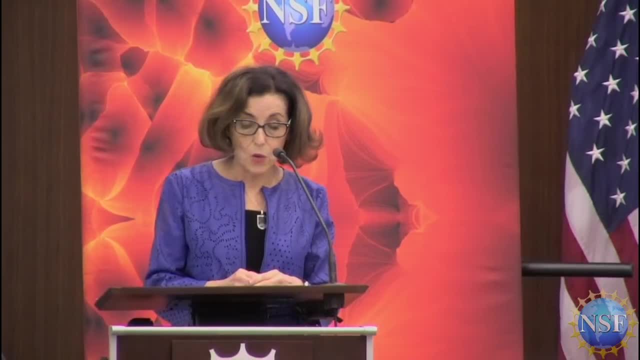 of the universe's immense cosmic accelerators, which are far larger and more powerful than anything we could build on Earth. Despite all the progress we've made with particle accelerators like the giant ones at CERN and Fermilab, we still can't produce anything with nearly the energy. 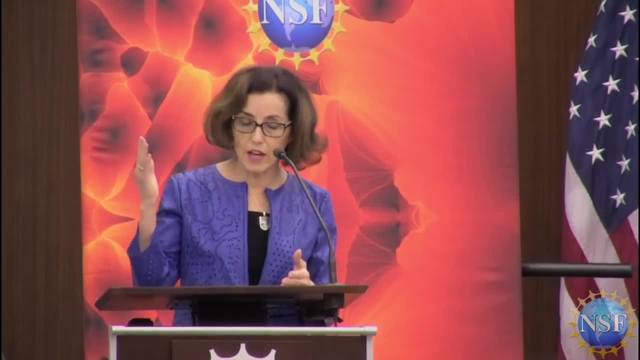 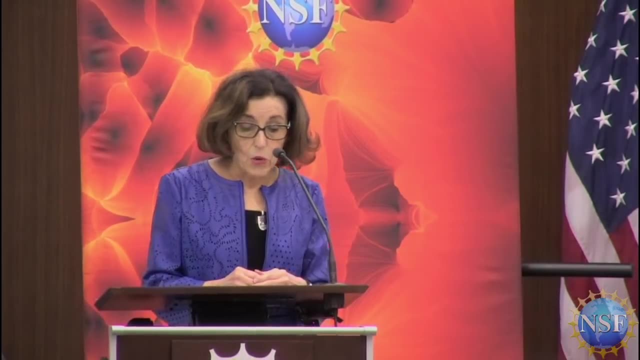 of these cosmic particles. So we have to turn to the heavens to deepen our understanding of the highest energy processes. Creating NSF's IceCube was a difficult process, but the rewards have justified the investment and again demonstrate the importance of building entire ecosystems of basic research. 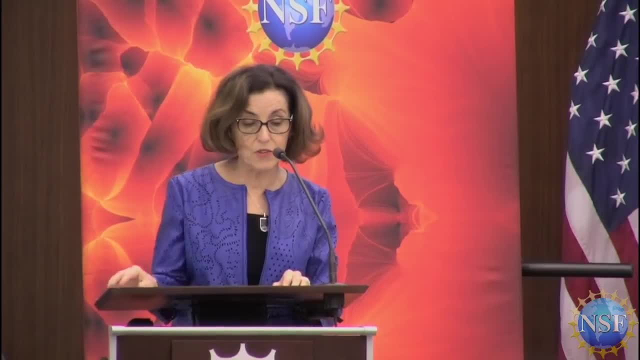 This work would not be possible without the foundational discoveries made by neutrino physics pioneers, including Nobel laureates Melvin Schwartz, Frederick Rynas and Raymond Davis, all NSF supported. Discoveries like this build on advances that result from years of painstaking investigation. 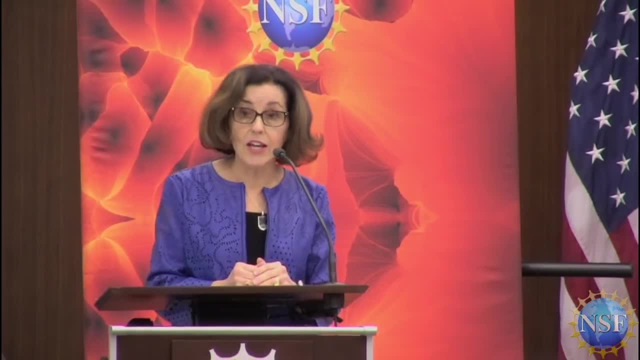 The federal government has a unique, unique role in these discoveries as the only supporter with the resources and mission to ensure that high risk, high reward, long-term research continues. Like the recent detections of gravitational waves by the NSF-funded LIGO facilities, this work shows that consistent investment. 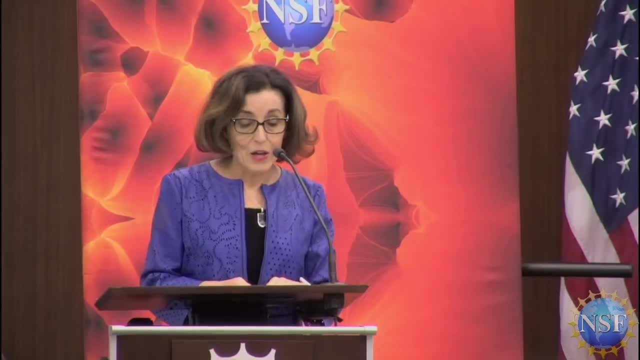 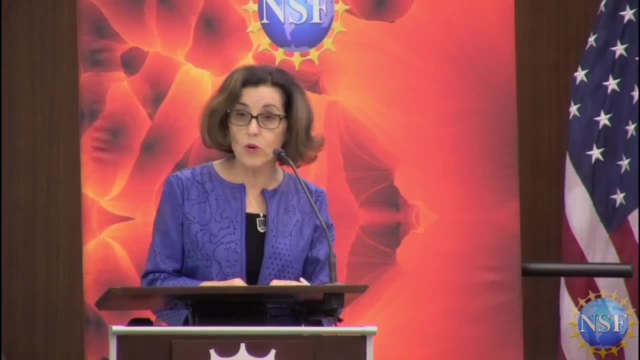 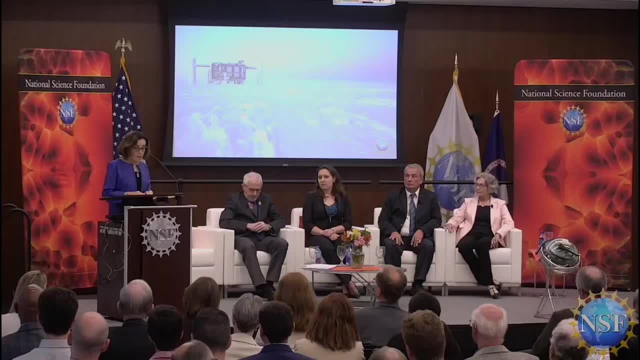 I want to commend the researchers for how they've presented this to the world. The experimenters take care to quantify the statistical significance of the spatial and temporal coincidence of the high energy neutrino detected by IceCube and a blazor flaring in gamma rays. 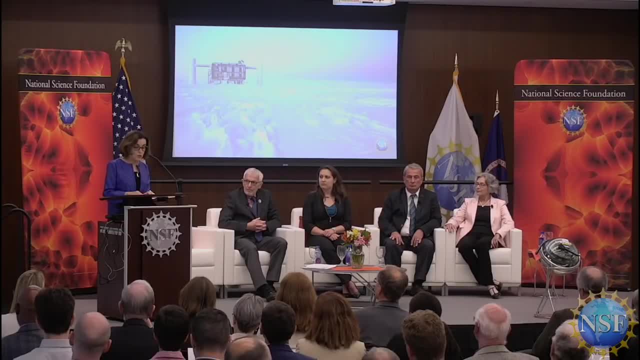 Like Hesse's discovery of cosmic rays, these first results will raise new questions and open doors for new research. As in all good science, this is only the beginning, and that's exciting. Now let's hear about the new updates from today's presenters. I'd like to 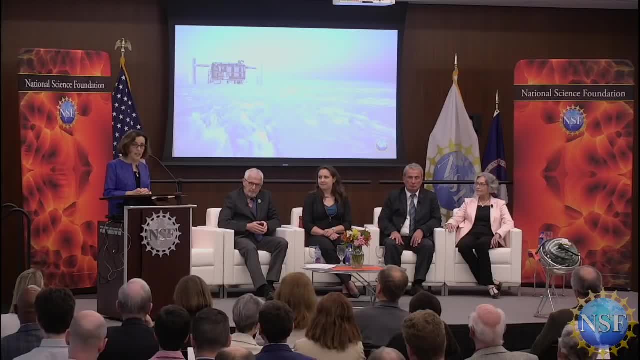 welcome. Frances Halzen, Principal Investigator of the IceCube Observatory at the South Pole. Regina Caputo, Research Astrophysicist at NASA's Goddard Space Flight Center in Maryland. Razmik Mirzoyan, Senior Astrophysicist at the. 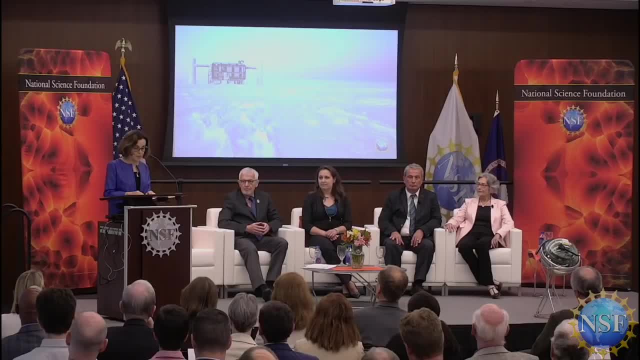 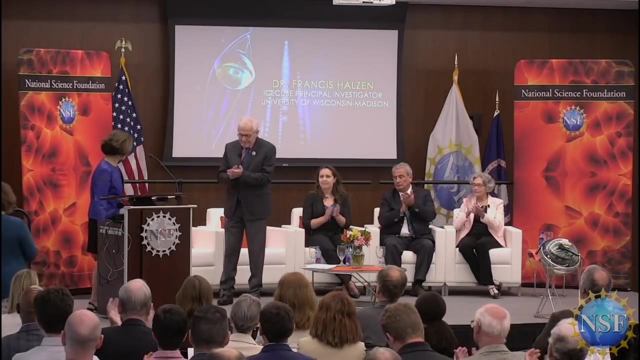 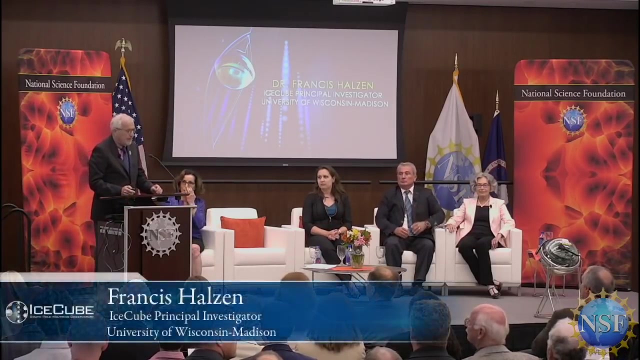 Max Planck Institute for Physics in Munich, Germany, and Olga Botner, Professor of Experimental Particle Physics at Uppsala University in Sweden. First, Dr Halzen After the director's introduction, I think I should show a picture of Victor Hess. 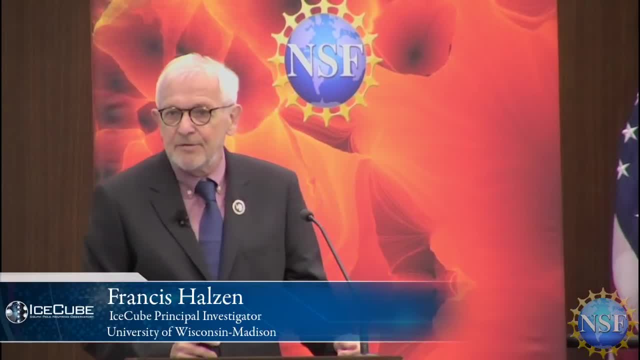 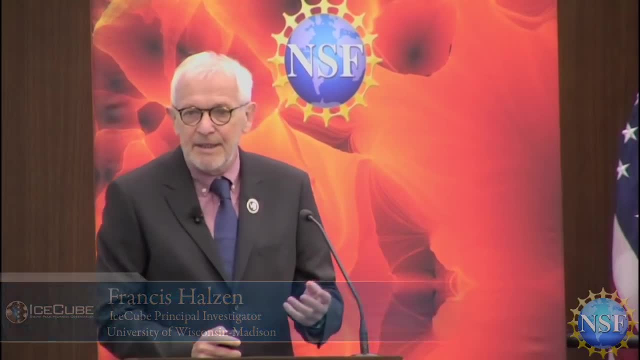 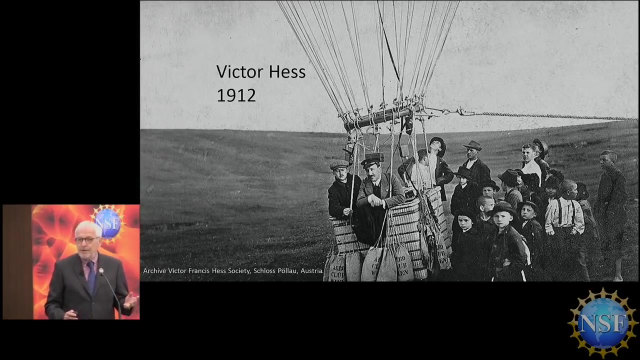 who just ascended to 17,000 feet without oxygen. He discovered cosmic rays which are not rays, they are nuclei, mostly protons, and and we don't know where they come from. We have been seeing neutrinos since 2013 and 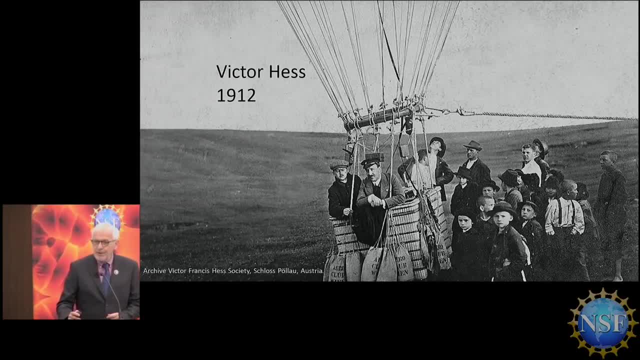 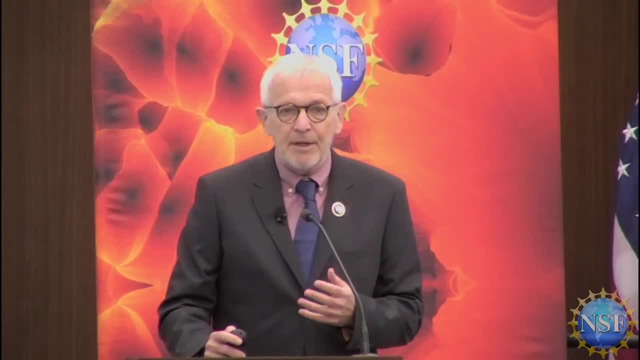 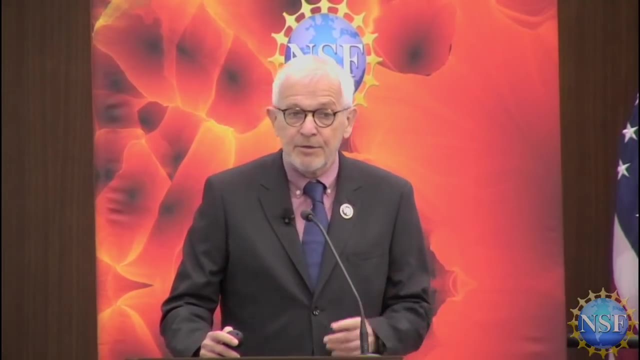 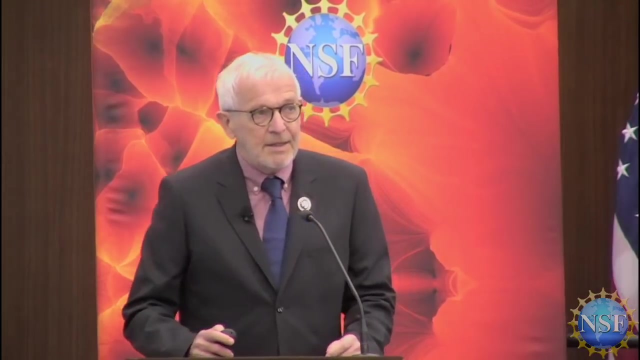 we still didn't know where they came from. It's one of the oldest open questions in astronomy and of course, the issue fascinates particle physicists, because cosmic ray accelerators routinely accelerate particles to 10 million times the energy of the light. That's similar to the technology aroundété and quantum câlidos. about Ishara's? 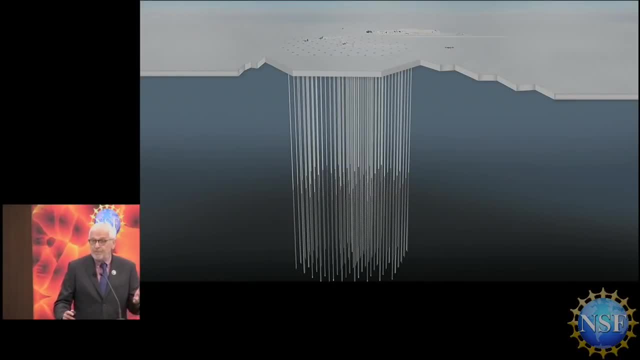 mal-Haramoon问题, So it is obviously a very successful project. We don't need logarithmic unst toplary arrassing, so we put a large hardware andhalider beam in Geneva So to track cosmic accelerators. those was actually deflawed. all was meant to be. the flagship mission of ice cube. we transformed a kilometer cube of ice, a mile deep under the Geographic South Pole, under the schema science foundation station, into a neutrino detector and it's very simple: you feel a kilometercube체. grináá Tasca. 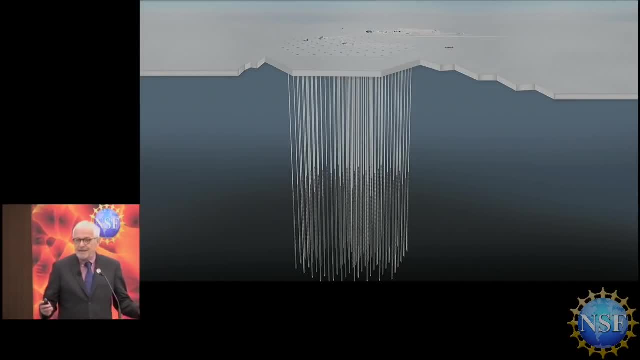 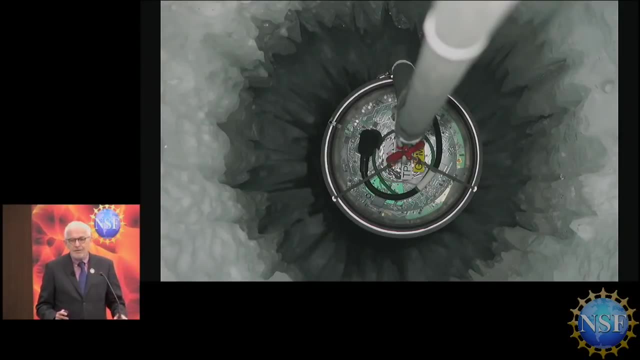 of ice with 5,160 light sensors and you detect neutrinos. So this is a neutrino, an optical module, an optical sensor starting a trip probably 2,400 meters deep, And that's the last time you see it. 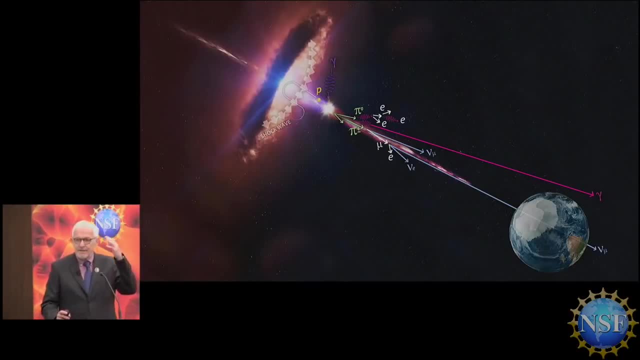 So why neutrinos? This is like a theorist image of a cosmic accelerator, a black hole of some kind, And it managed to transform some of its gravitational energy into accelerating particles. So there are accelerated protons because it's a cosmic ray source. 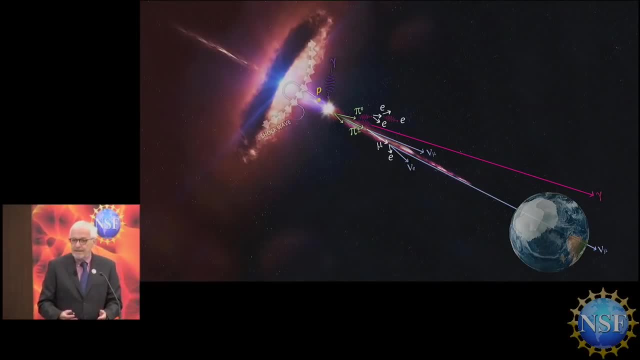 And they will interact with the light in the galaxy and with the hydrogen and produce neutrinos. So The goal is to track cosmic ray sources by looking for neutrinos, And so they will point back. They're neutral particles. They will point back at the source. 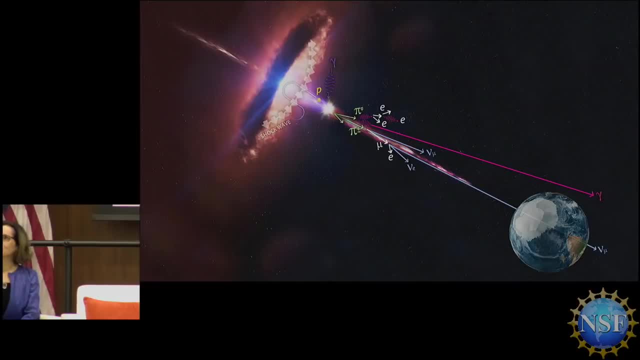 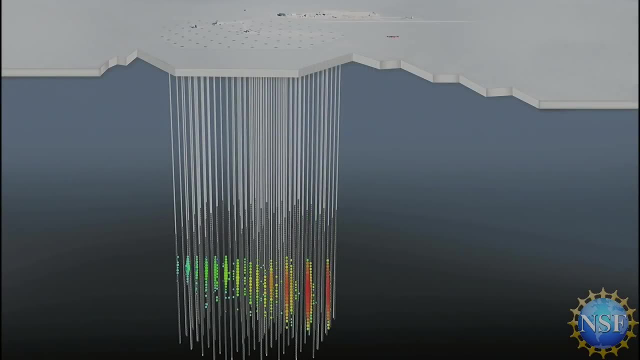 And on September 22 of last year, that's exactly what one neutrino did, And you can see it coming through the ice, lighting up the sensors. In fact, you don't see neutrinos. What you see here is a muon, which is a particle. 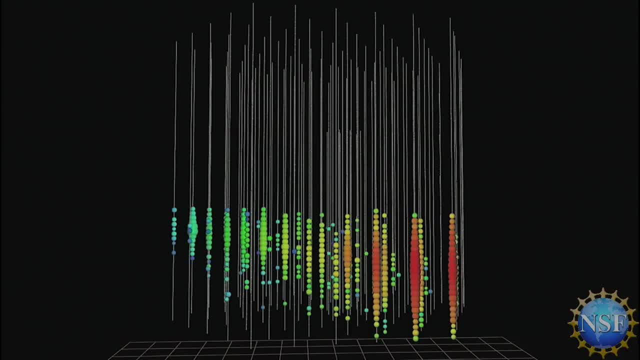 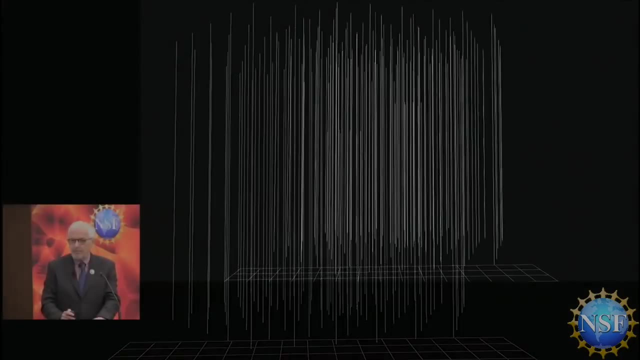 particle that was made by a neutrino somewhere to the right of the detector and that streaks at the speed of light through the ice, lighting up the sensors by the blue light that it emits. So within 43 seconds the computers at the South Pole captured these signals, reconstructed. 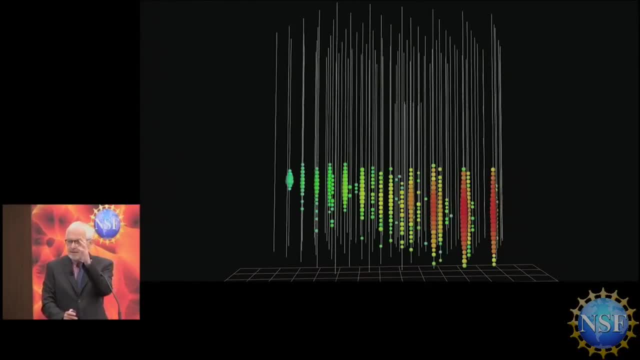 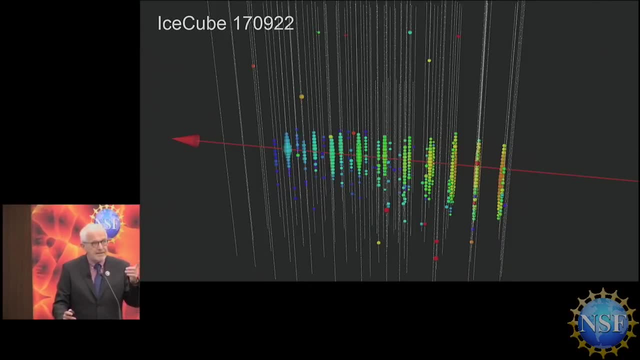 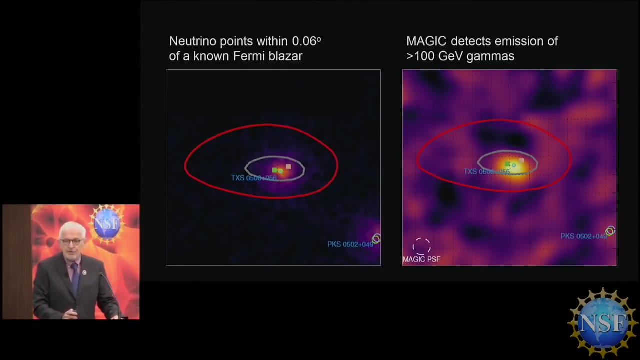 the energy and the direction of the track and sent it for any telescope in the world that would be interested in it. This is the event, And so what we find out is that sometime later- if you look at the picture on the left within, 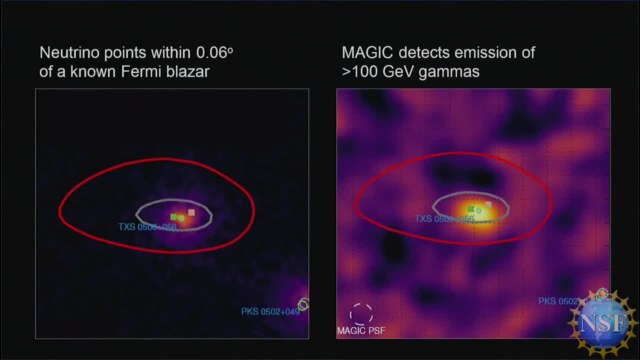 0.06 degrees. Fermi was aware of a source, an active galaxy that actually was flaring It in the last few months increased its output, its power, by a factor of more than six. So this is the event. 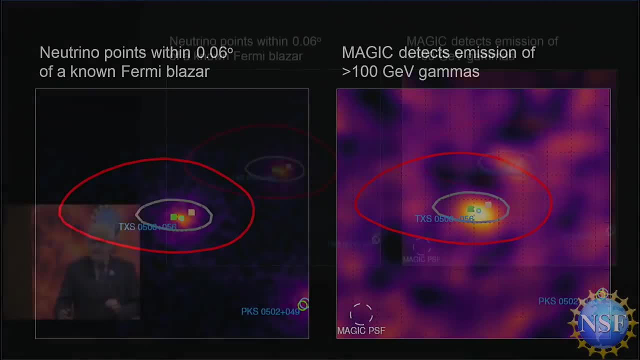 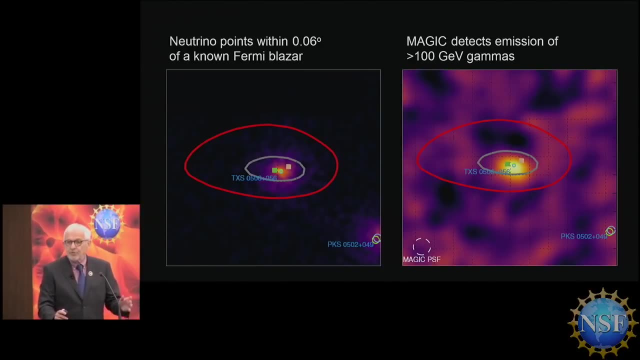 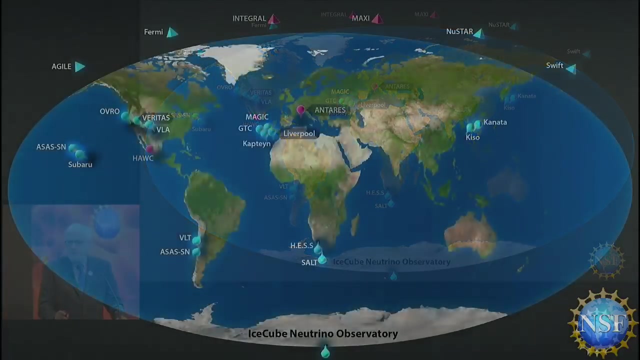 Subsequently, the magic telescope that detects the highest energy form of gamma rays that we detect in astronomy detects that the source emits TV gamma rays. This is a very unlikely event, So by then- this was interesting and more than 20 telescopes which are shown on this. 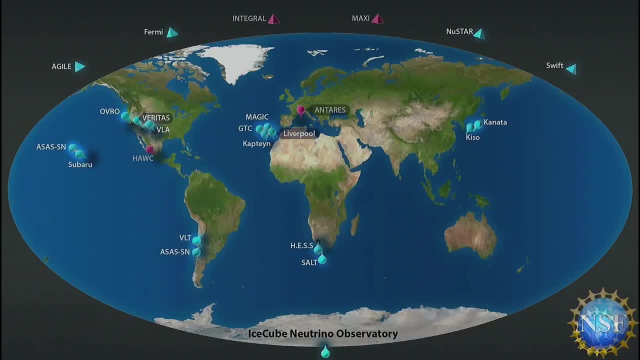 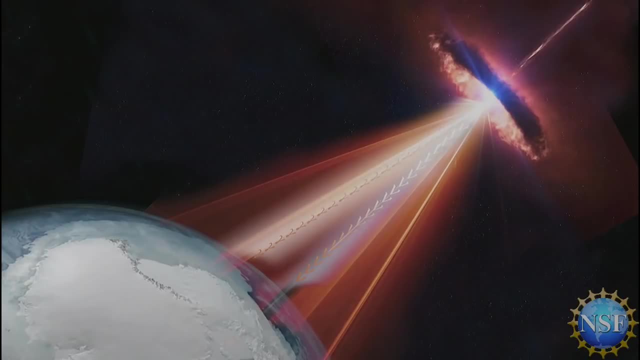 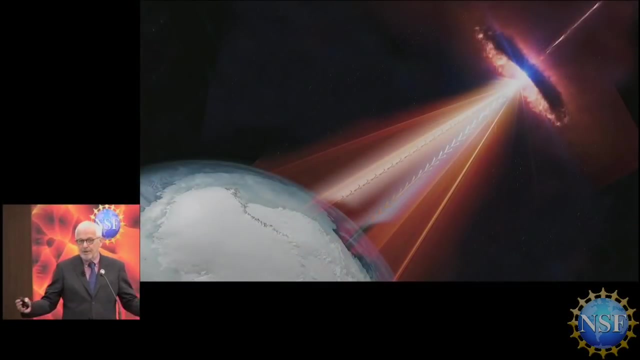 slide, looked at the direction of gamma rays. So that's the entire timeline of this event. So that's, however, only the beginning, because now we knew of an interesting place in the sky, both Fermilab collaboration and the IceCube collaboration. 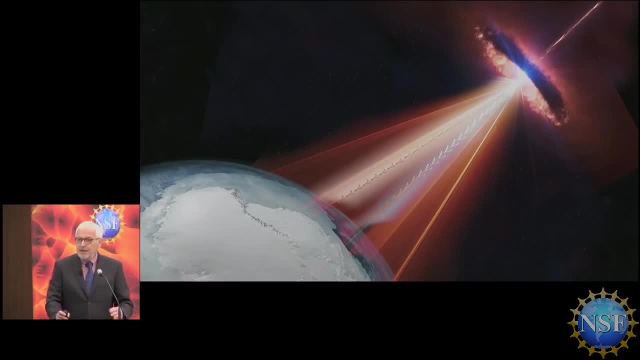 We've stored some 10 years of data on tapes and now- And we can look back in this direction, And that's what we did about- was dominated by essentially one: 290 TV neutrino. when we look back in our data, we found that in 2014, there was a flare in neutrinos- more than 12 that. 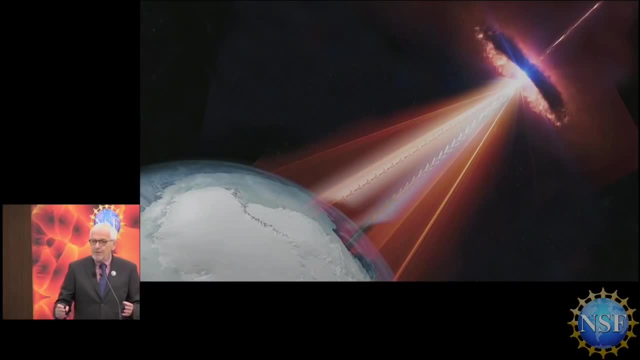 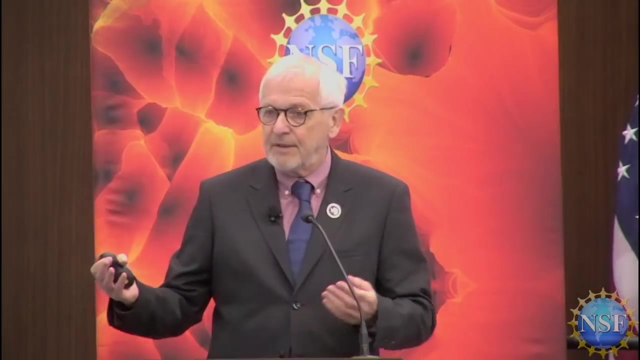 came in 150 days when we measured the energy distribution. the energy pattern of the neutrinos is exactly that what we expect from cosmic accelerators. in fact, that's the same, if true, for the gamma rays in 2017 and 2014. so what did we? 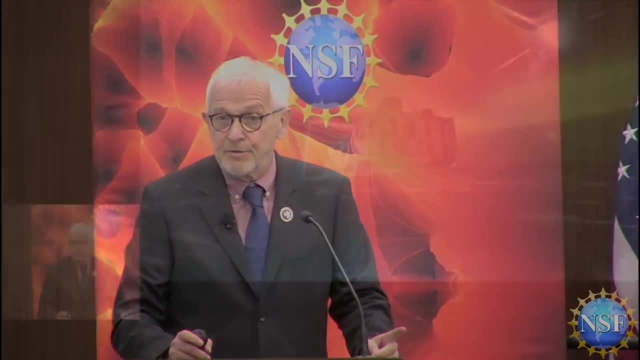 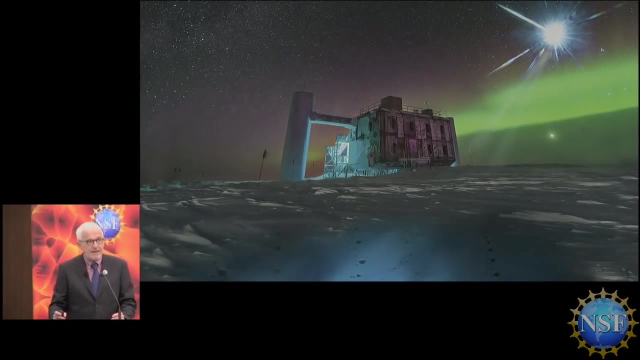 discover. well, we finally discover one source of cosmic rays. it's a super massive black hole that is powers the accelerator and produces the neutrinos and the gamma rays subsequently detected. this is all the beginning, but through this campaign we have collected an incredible amount of data on this source and, most important, we know it accelerate protons. 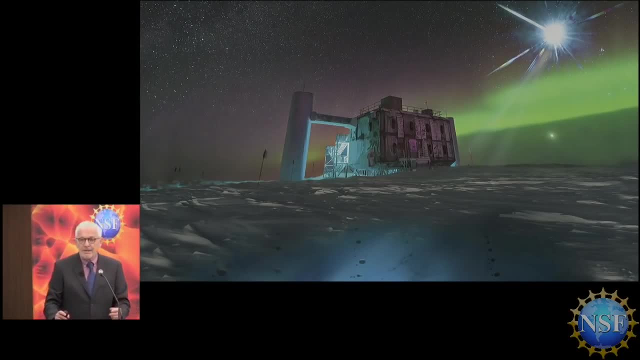 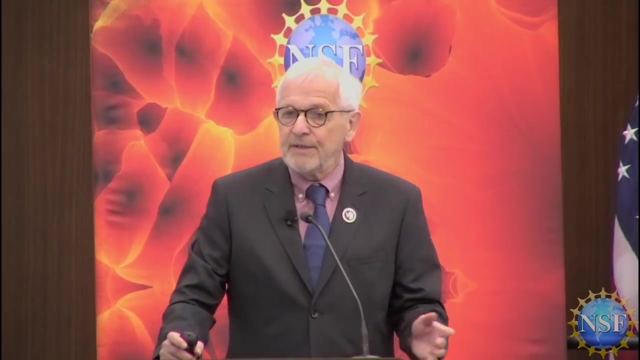 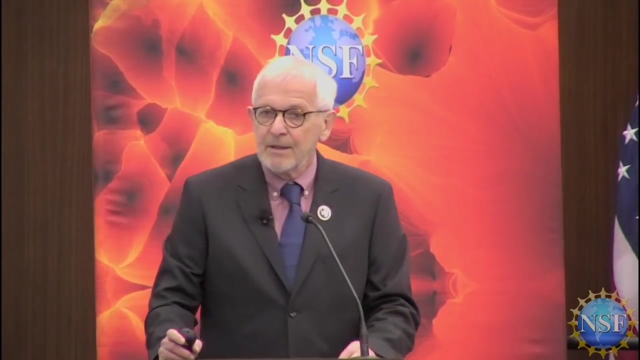 and not just electrons. so this is actually not the first time multi messenger neutrino event occurred. it occurred in 1987, when a supernova exploded in our local neighborhood. but who could have guessed that we would stand here 30 years later and report a similar event with neutrinos that are 10 million? 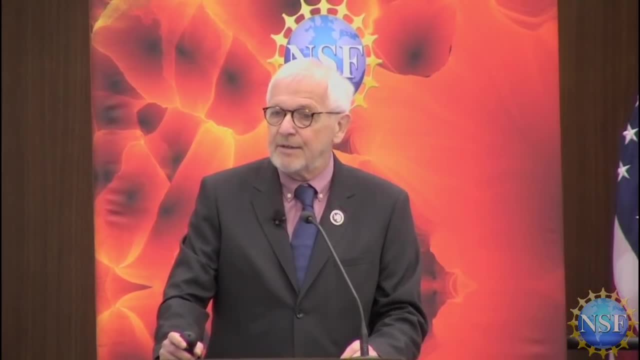 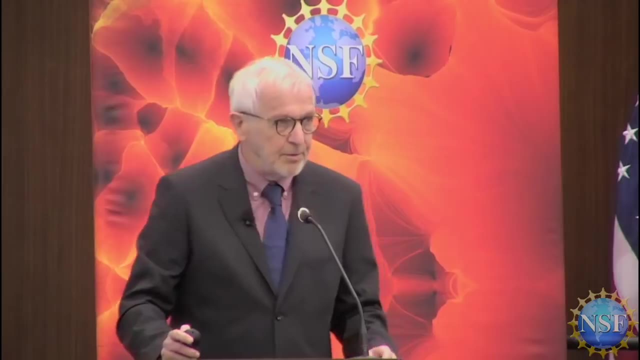 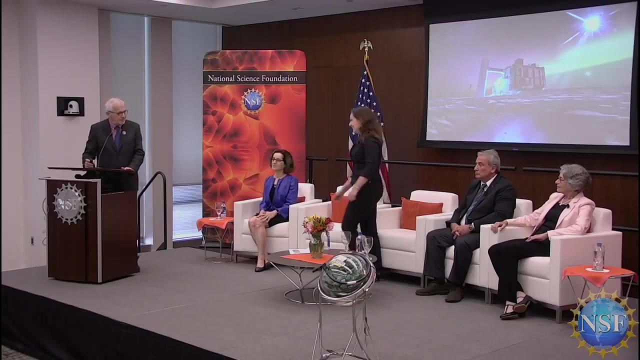 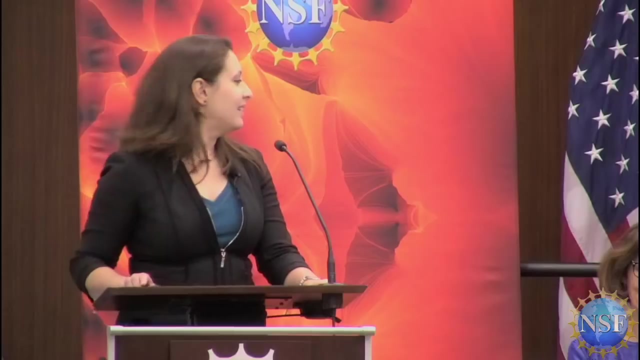 times higher energy from a source that's a hundred thousand times further away in the universe. so to tell you the rest of this story, I like to introduce Regina Caputo, who is the analysis coordinator of the Fermilab collaboration lab, and I'd just like to thank her for the opportunity to come here to talk to us. 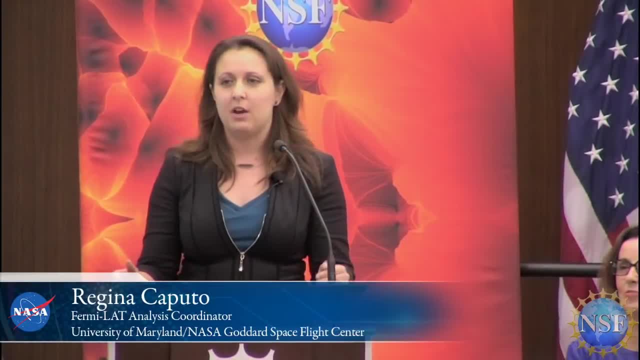 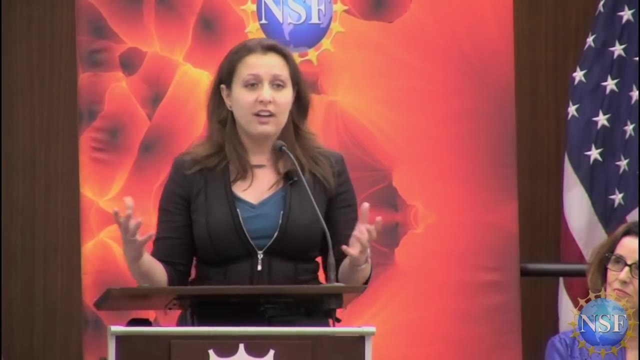 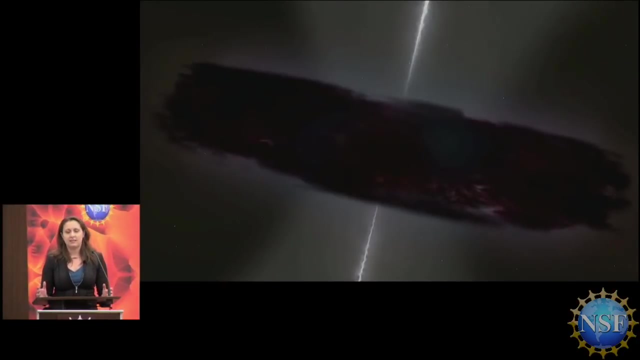 today. Thank you, Frances. it's a privilege to be here today speaking on behalf of the fermi large-area telescope collaboration, a collaboration of over 400 scientists from around the world who are constantly monitoring the gamma-ray sky. so the object that we're talking about today, as you've heard a few times already, is a 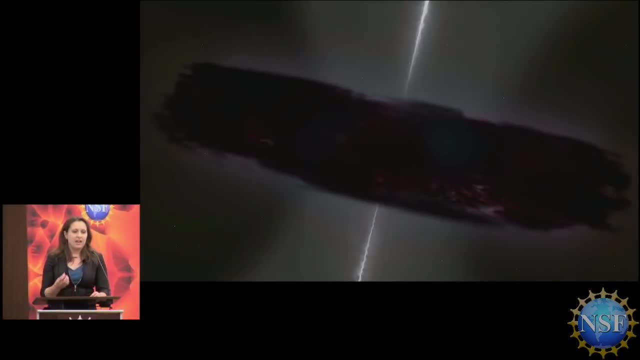 has a very dense core at the center, and at that core is a supermassive black hole. that's millions to billions- the times of the mass of the Sun. Now it's surrounded by gas, and what you're looking at in this visualization is this central core of a galaxy. 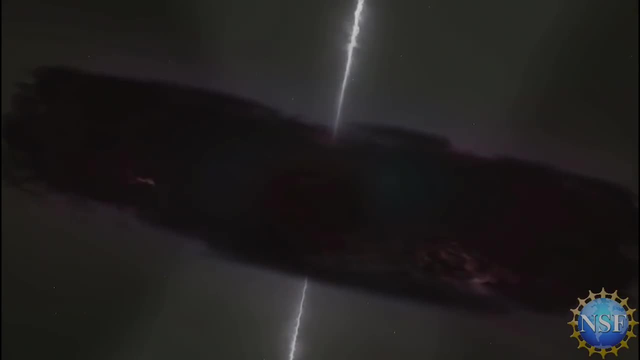 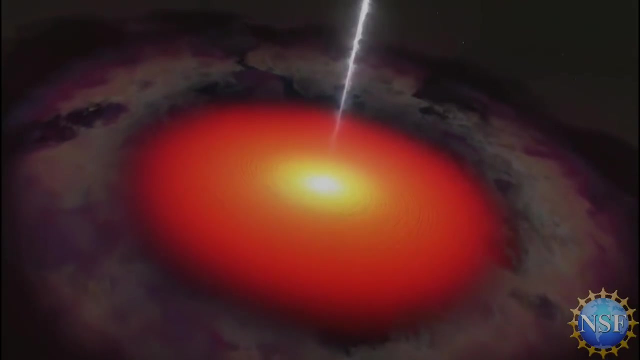 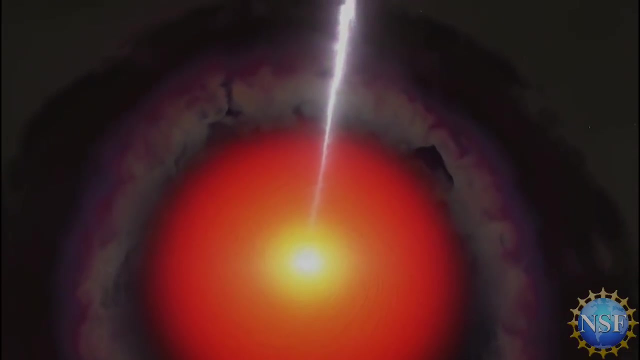 As we go in, you'll see this gas that gets gravitationally compressed into a disk and gets accelerated and swirled around this central black hole. Now, sometimes these particular galaxies shoot out jets of particles. These blazar jets are true cosmic accelerators and they accelerate. 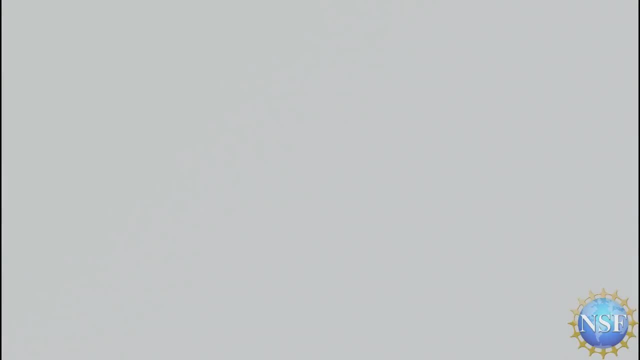 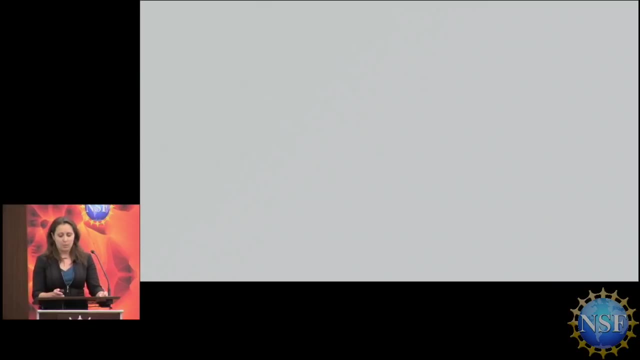 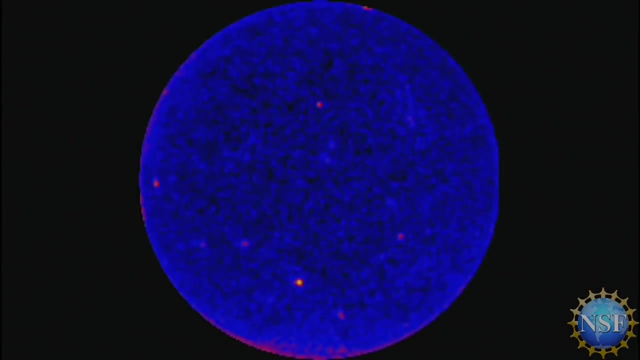 particles to the highest energies, higher than we can see on Earth. Now, when that jet is pointed at us, that's what we call a blazar. Now the Fermi Large Area Telescope, or the LAT, observes the full sky and the scientists who analyze Fermi data are 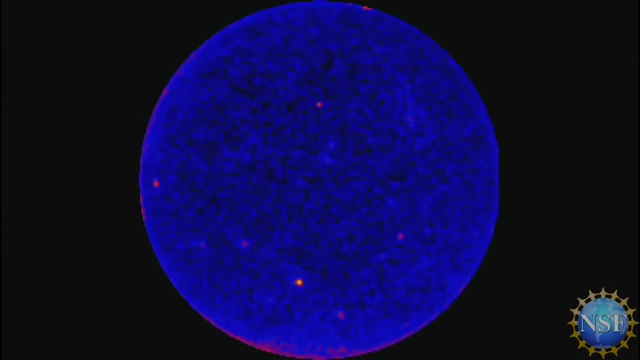 constantly checking for objects, variability and changes in that gamma-ray sky, And so what you're looking at here is an image of the northern hemisphere of the galaxy in gamma-ray data, and you'll see a time-lapse image over about eight months of these flaring objects. 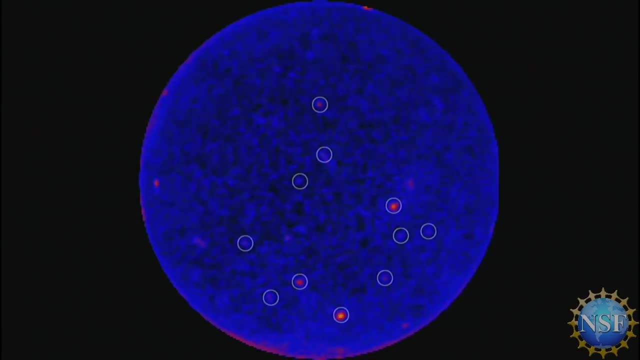 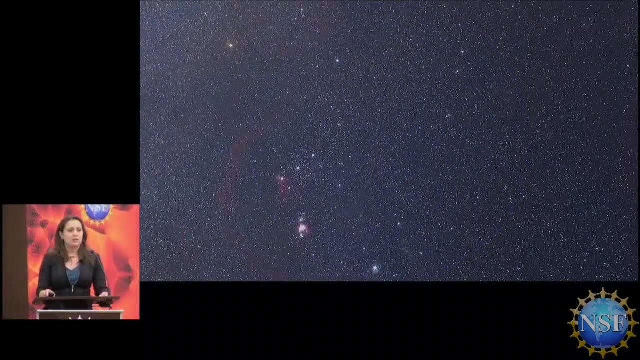 So you see, they change, the flux, changes and flares and increases And what are circled are the 11 most energetic blazars that we observe. We actually observe over 2,000 blazars in the gamma-ray sky. So this particular blazar, called TXS 0506, is 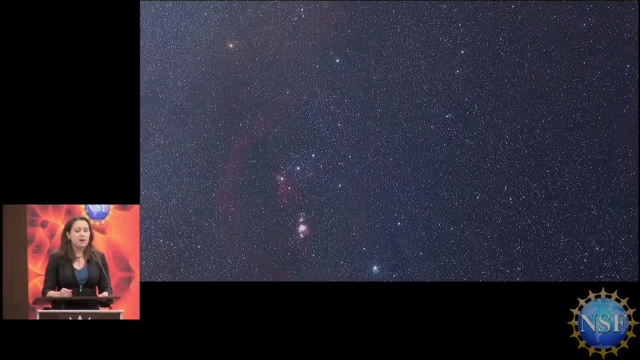 located in the Orion constellation, But it's about four billion light years from Earth. Now, if you are looking at this, it's a little bit more than the original TXS looking at the sky at Orion. this is about what you would see with your eyes. 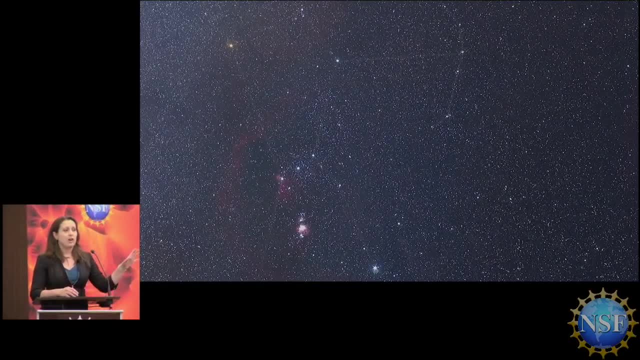 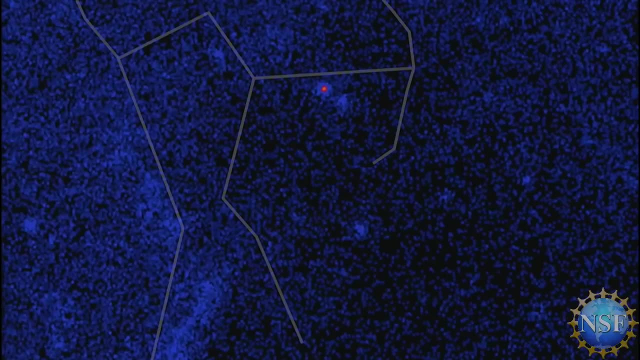 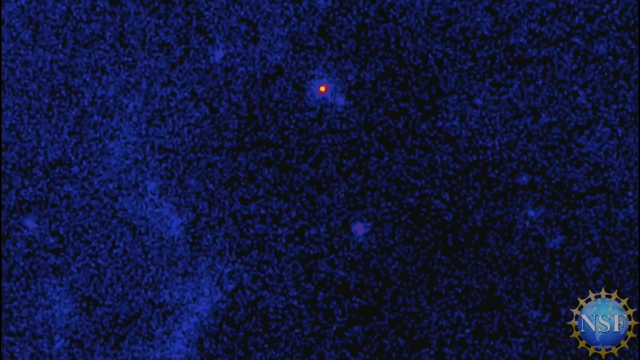 But the way that we see it in gamma rays, and we'll go ahead and outline Orion as a reference. you see, it's the source right there under Orion's arm. Now, this particular source is a bright Fermi source. We've seen it for 10 years And, starting in April, it experienced one of the 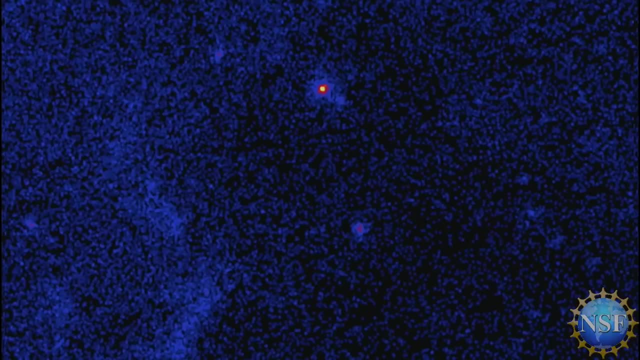 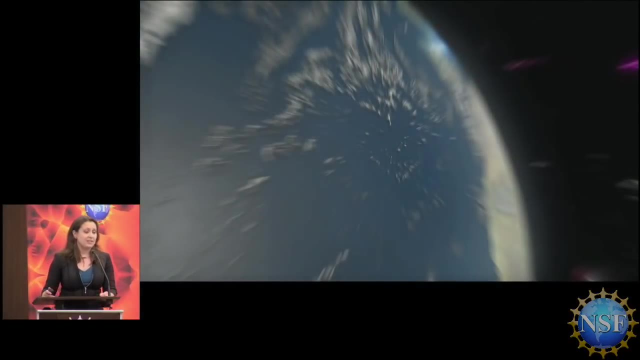 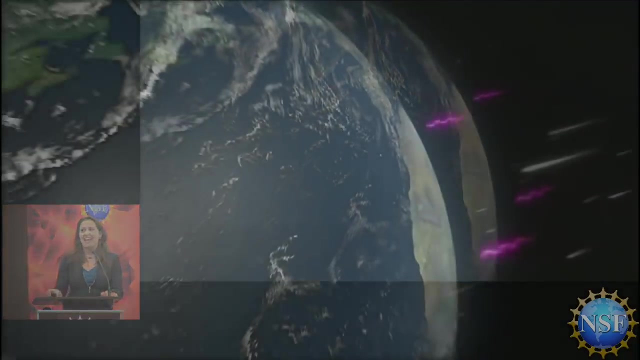 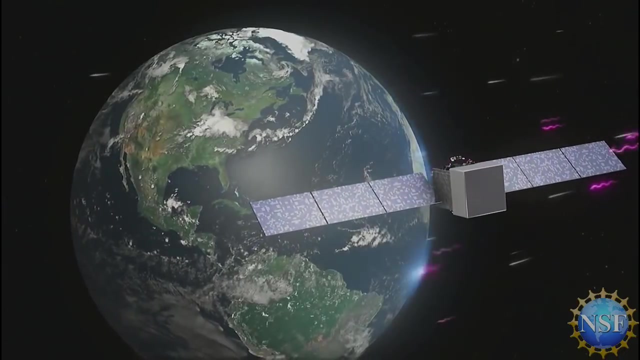 largest flares that we had- well, the largest flare that we had ever seen from this particular source. Now Fermi is on orbit in space, which is probably the only place that's more inhabitable than the South Pole, And what you see is gamma rays coming in, the magenta squiggles formed in the same place. 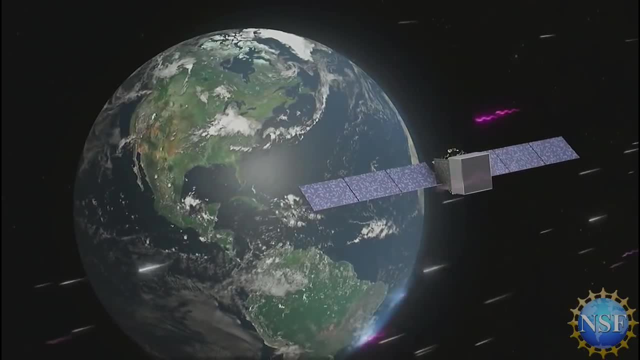 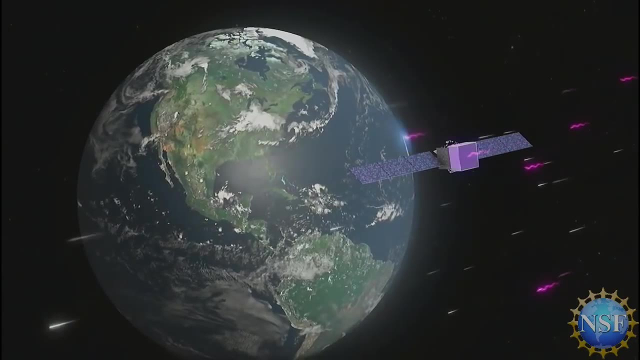 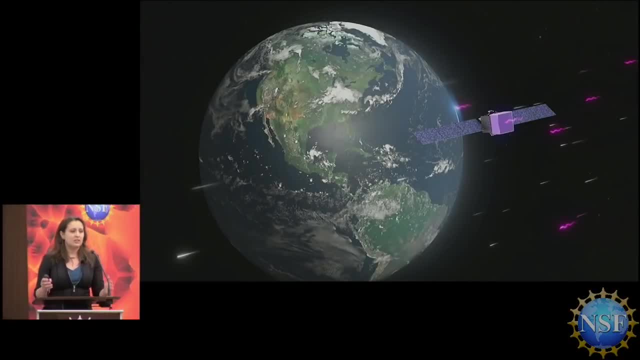 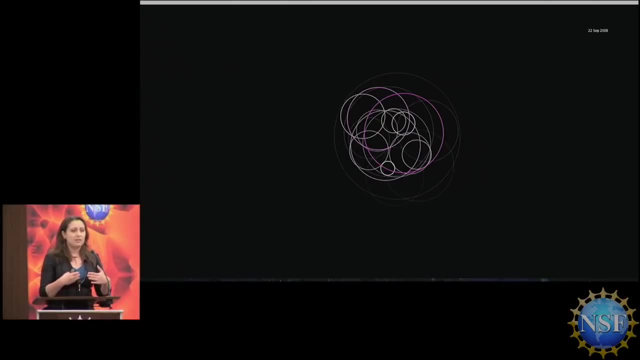 straight through the Earth. Now, just to give you an idea of what this source looked like for the first 10 years, we have a time-lapse video showing the gamma ray data as represented by these circles, where the size and color of the circle is representative of the energy of the. 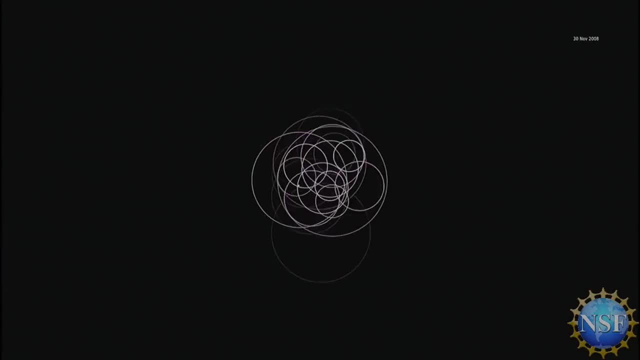 gamma ray that entered And so you could see. we see lots of gamma rays from this source. It's an active source, It's bright, And this is what a typical emission state looked like Then, because we're able to monitor the sky. 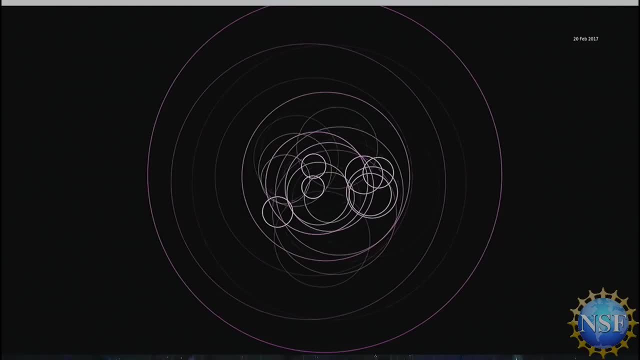 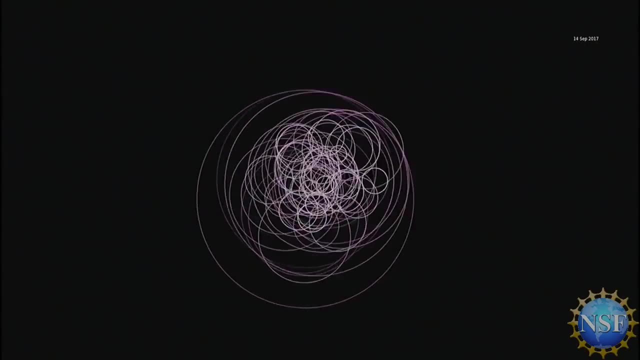 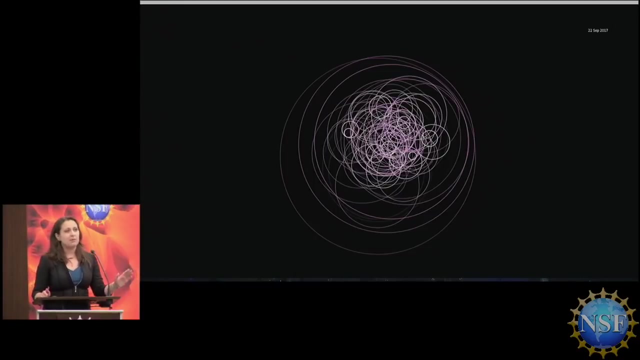 all the time. we were able to notice that during April, which starts right now, that the number of gamma rays from this source increased by a factor of more than six. So it was very, very crazy emission from this source And I've stopped it on September 22nd 2017.. And you'll see just how much. 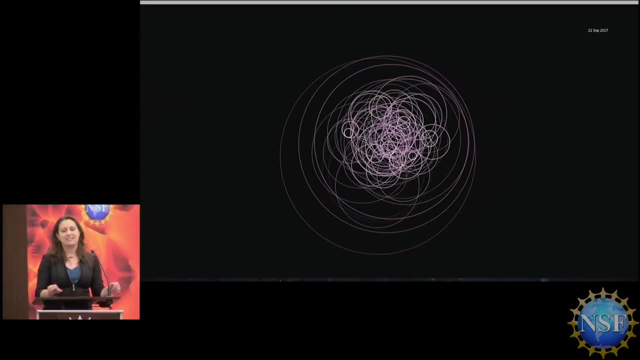 this is, And you'll see just how bright this source was in gamma rays as represented by these circles. And so it was really, really exciting when we got the notification from IceCube, because, as I've mentioned, blazars flare, But the fact that we could tie together the gamma rays and the 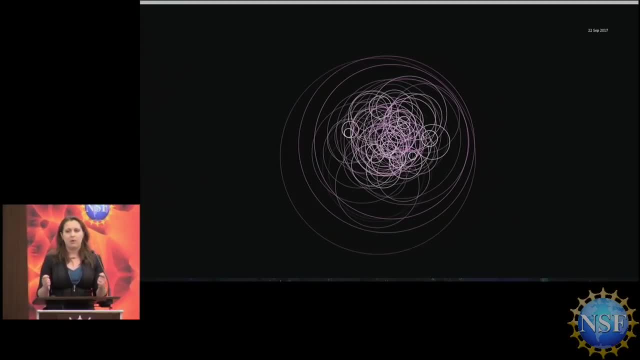 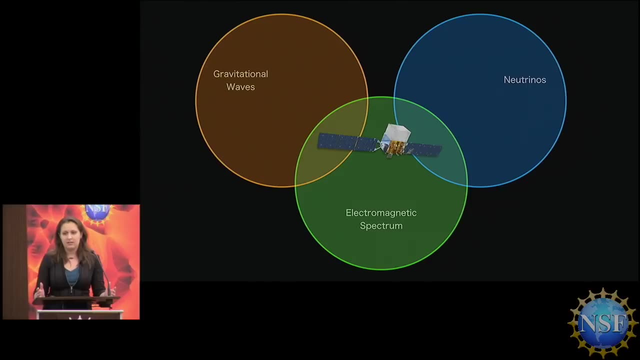 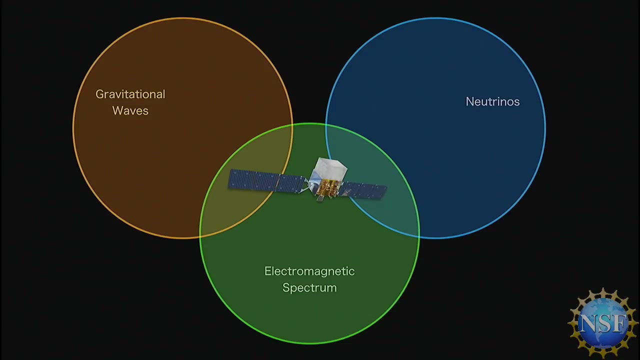 neutrinos tells us something very exciting about the particle jet and the particles that are being accelerated. So we've now entered a new era, Starting last year with the joint discovery of gravitational waves with gamma rays from Fermi. we were able to view a cosmic explosion when two 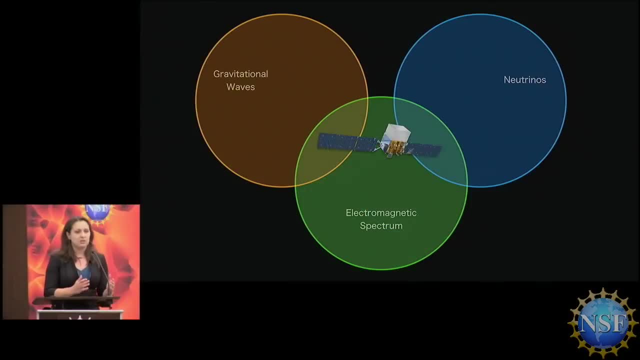 neutron stars merged And we were able to detect it in these multi-messengers. Today we're really excited to report. now we know something about cosmic accelerators in the joint detection of neutrinos and gamma rays, And so to give you more information about the cosmic accelerators, we're going to go ahead and 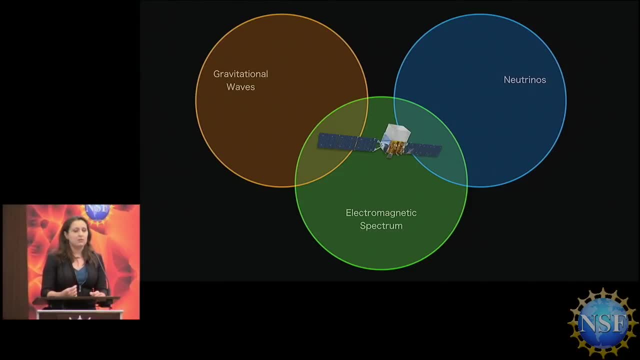 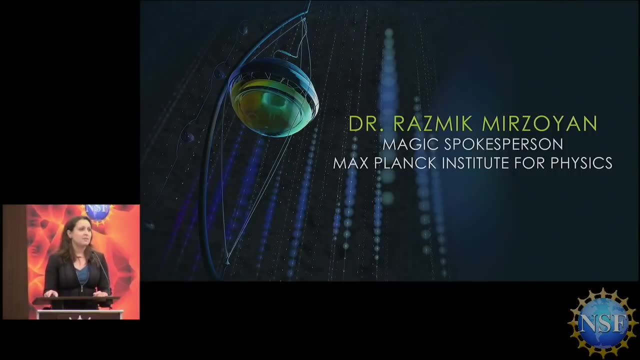 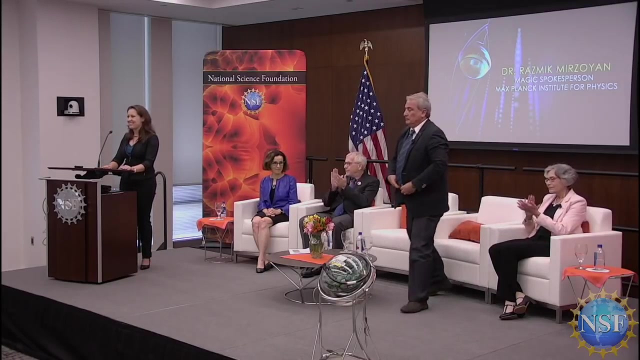 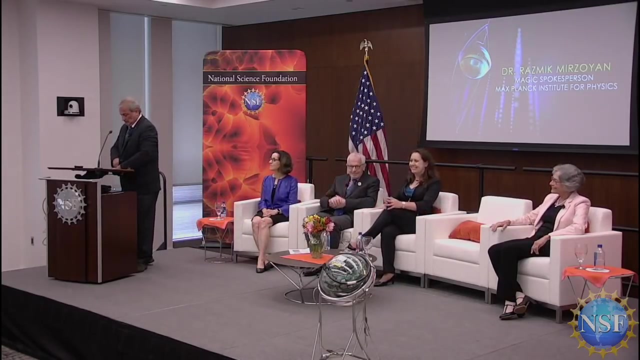 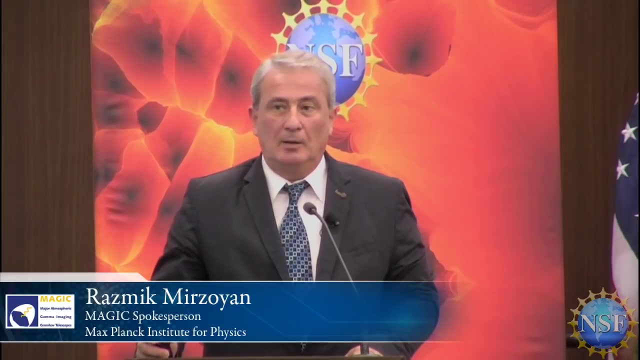 talk about the 20 observatories that followed up this very exciting notification. I'd like to introduce Dr Razmik Mirzoyan from the MAGIC Collaboration, who's the MAGIC spokesperson. Thank you, Good morning, ladies and gentlemen. I feel privileged to be today here and to talk from the name of the MAGIC Collaboration and to talk about 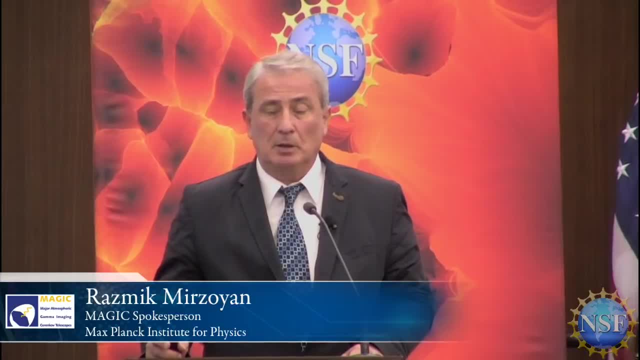 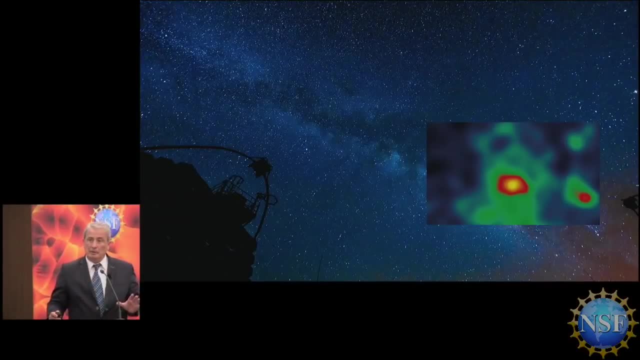 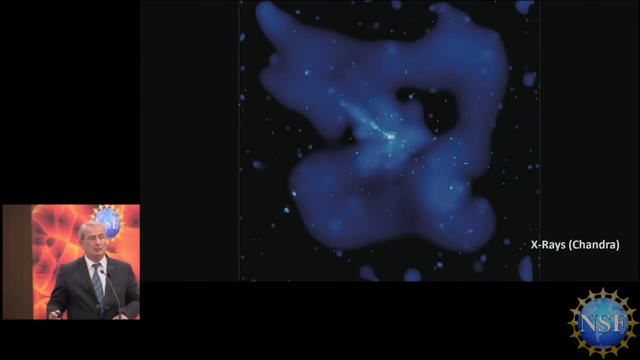 measurements done by MAGIC in this big event, in this multi-messenger detection. In astronomy, we are observing objects in different wavelengths. You can see, just as an example here I show you a Senn-8, the source observed in X-rays or in optical wavelengths. This is the Senn-8, the source observed in X-rays or in. 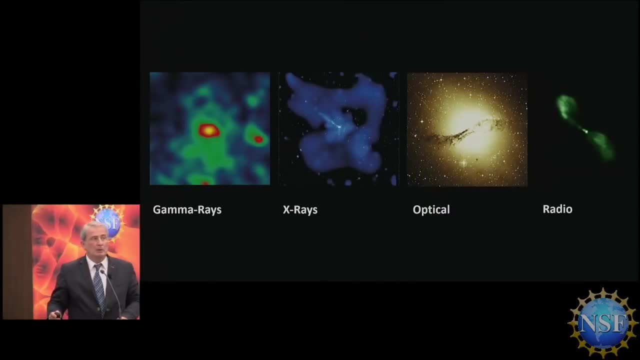 optical wavelengths. This is the Senn-8, the source observed in X-rays or in optical wavelengths. This is the thinks of a consortium of radio continuum, and then you can see that the source is looking very different depending on at which wavelength it's observed. and then this multitude contains a lot of information which allows us to understand the source nature. 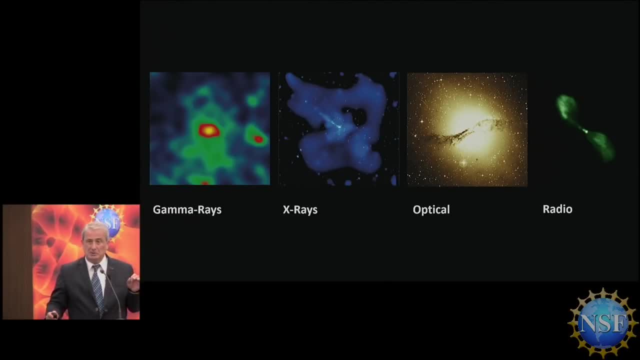 And now imagine that there is a multi- messenger detection and neutrino is coming into the game. and I should tell that I can remember something like 25 hav Greene high years ago, many discussions with my colleagues, with my friends, and they were saying: sometime in future, maybe it will become possible to measure sources, not 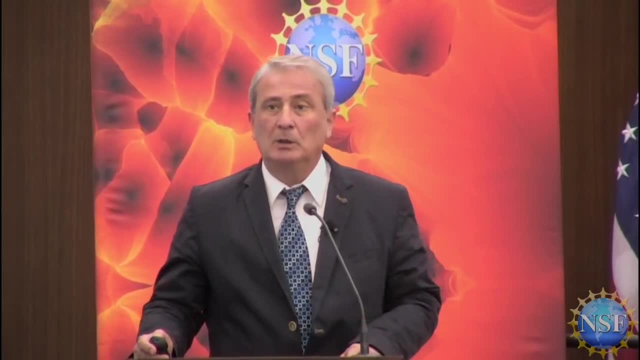 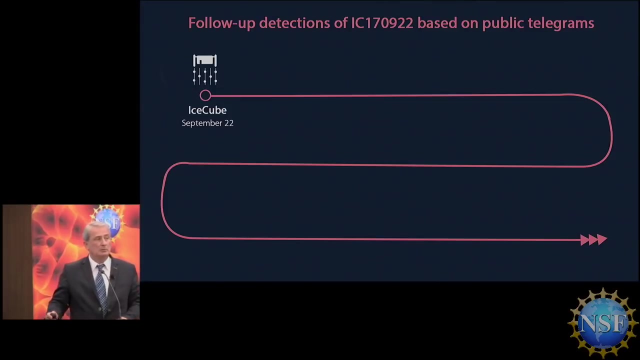 only across the electromagnetic spectrum, but also maybe one can measure with ground-based instruments neutrinos, and I'm very happy because today is becoming reality. On 22nd of September 2017, IceCube set an alert for an extremely high energy neutrino and a few days later, Fermi collaboration measured the 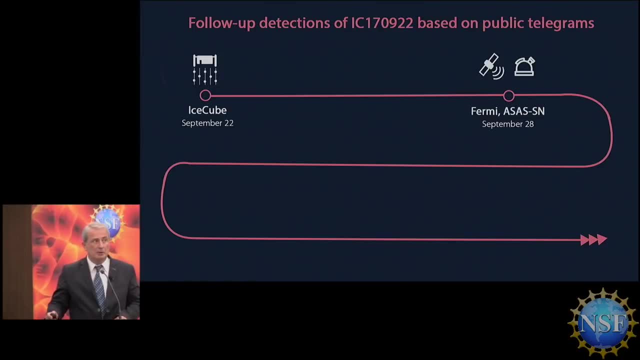 signal from a particular direction, practically coinciding with the direction indicated by IceCube, from an object with the name TXS 0.0506, and the signal was shown to be 0.0506.. And then that was followed with other measurements. magic telescopes measured. 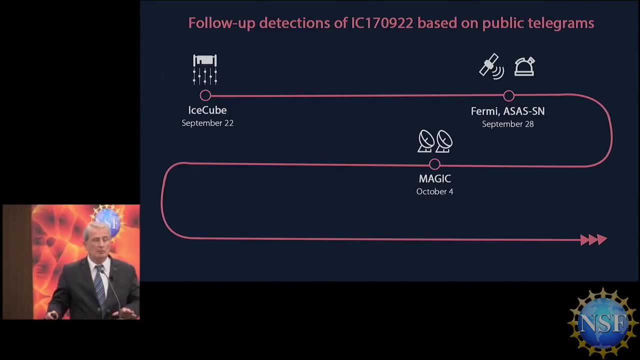 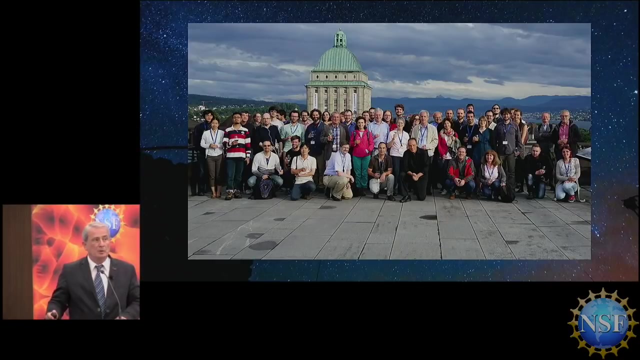 on during 12 hours a strong signal from from the same direction, like Fermi has indicated, and this was followed by an avalanche of other detectors, almost two dozens of instruments across the electromagnetic spectrum worldwide measured signals. So this is the magic collaboration. it's a middle-sized 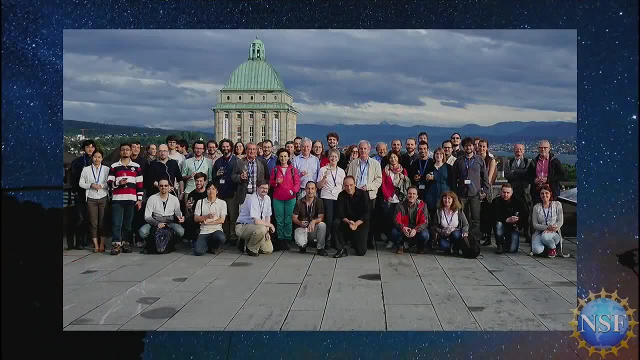 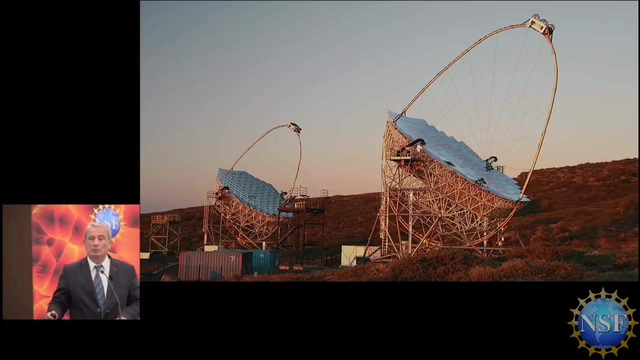 collaboration consisting of about 100 instruments. We have a total of 275 astrophysicists and two weeks ago we were celebrating 15 years of anniversary of operating our instrument on the Canary Island of La Palma. So these are the two magic telescopes which are located on the Canary Island of La Palma at an altitude of 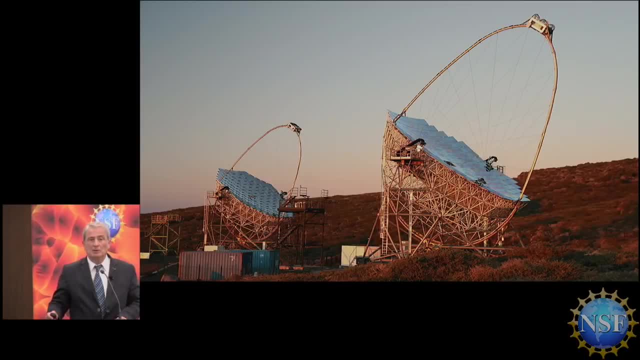 2,200 meters above sea level, and this is very different from what Regina has described and Francis has described. We have nothing to do with the ice in the South Pole or high up satellite mission. I think this is. La Palma is well known as a resort. 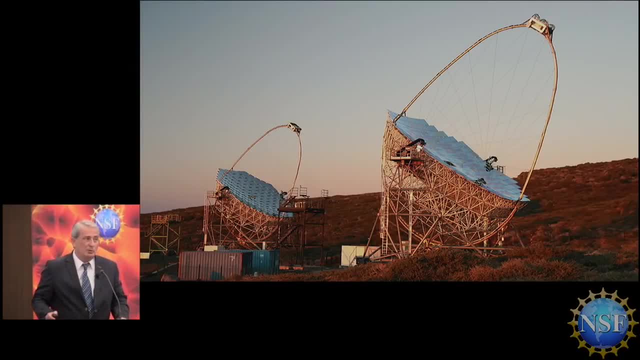 place for a place for doing vacations. So we are enjoying having vacations and doing science together and we try to do it very efficiently. These two telescopes: they have a 17 meter diameter each, they have a focal length of 17 meter and they are separated on 85 meter distance from each other. and these are 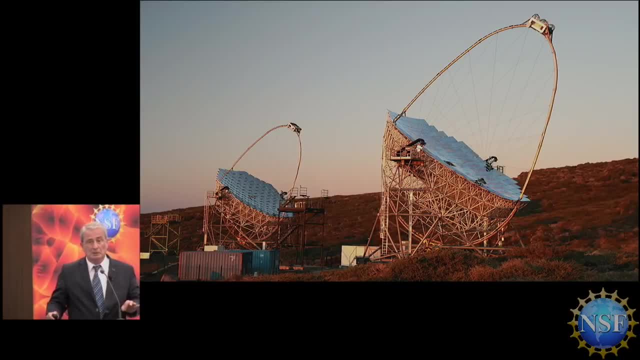 really high-tech telescopes. They introduced a lot of new techniques and methods into the field, and one of the distinguishing features of these telescopes is we can rotate them very fast. Within 20 seconds, we can go to any direction in the sky, and this is 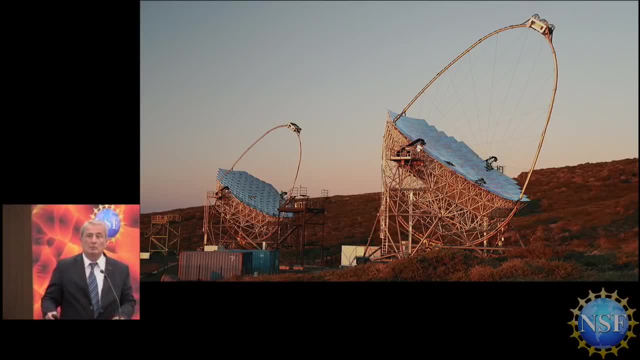 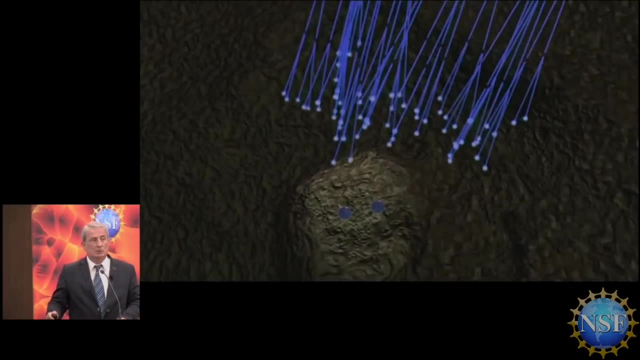 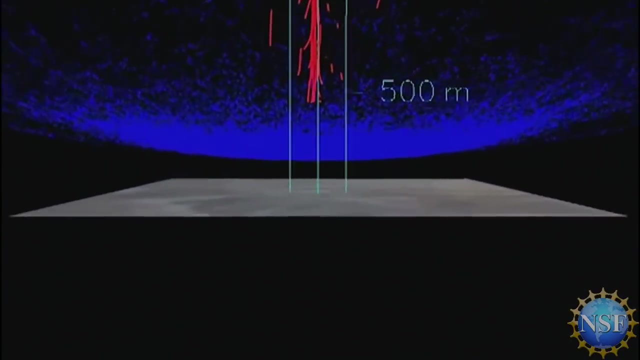 very crucial when a fast alert is coming, like the one from iSkoop. So this, in this cartoon, I would like to give an impression what we are measuring with these telescopes, because the telescopes are somewhat different from usual optical astronomy. Our Earth's atmosphere is not transparent to gamma-rays. they 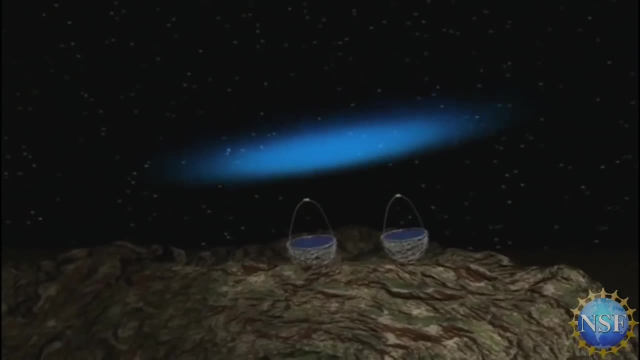 will be absorbed very fast. We can actually see the atmosphere of our Earth's atmosphere. It's not transparent to gamma-rays. they will be absorbed very fast. So we have the possibility: somewhere on 25 kilometer height cameras get absorbed, but then they produce secondary. 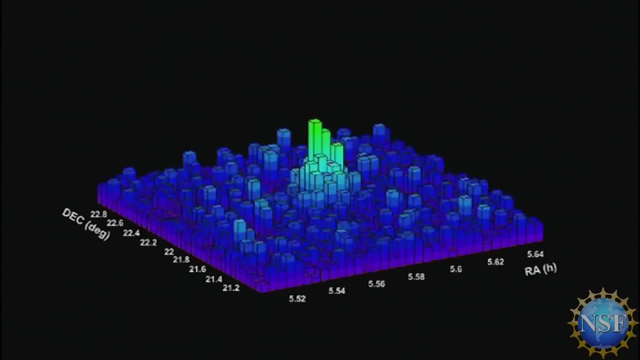 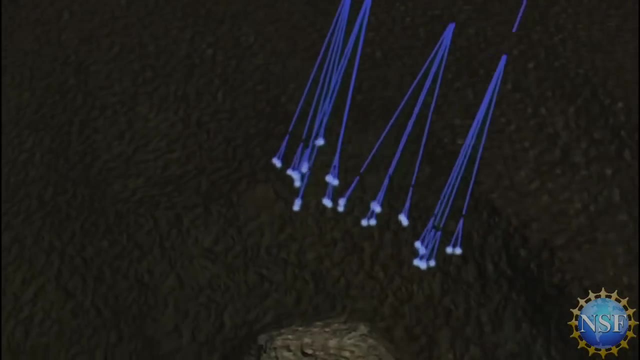 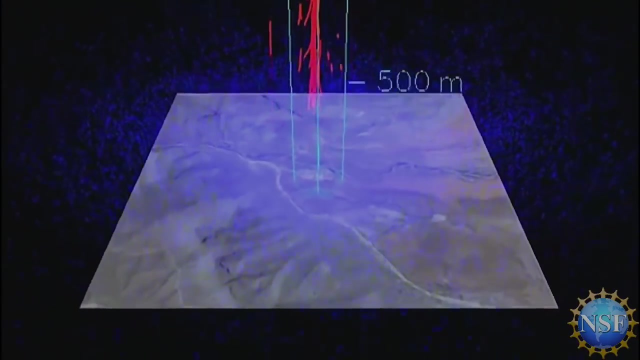 particles and the secondary particles, mostly electrons and positrons. they move at a speed higher than the speed of light in the air and they emit this bluish light, this blue color light. So these telescopes are measuring this, collecting this blue light and then focusing it into 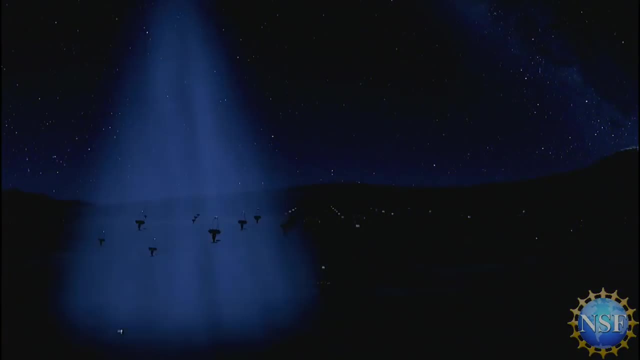 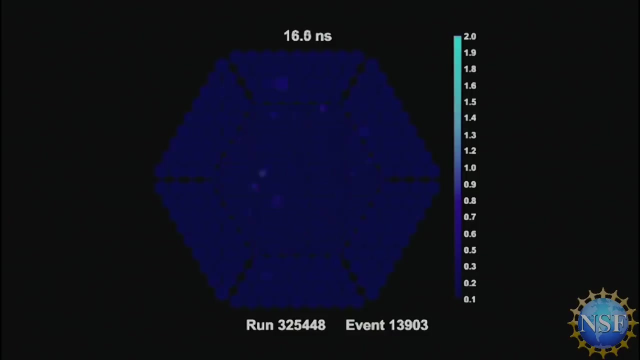 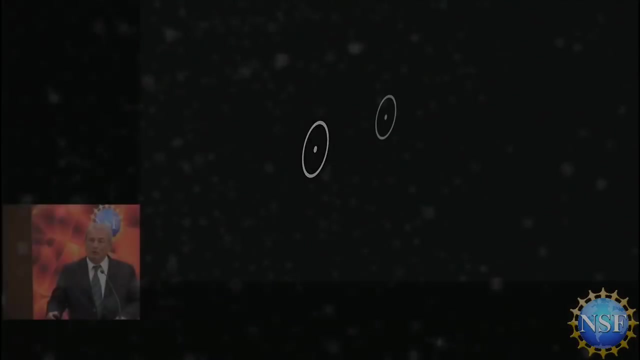 the focal plane, where an imaging camera will measure the shape of an air shower in the atmosphere And then, based on this shape, we can measure the energy and then most parameters of these gamma rays. This is how these telescopes are working. I would like to show to your attention a cartoon. 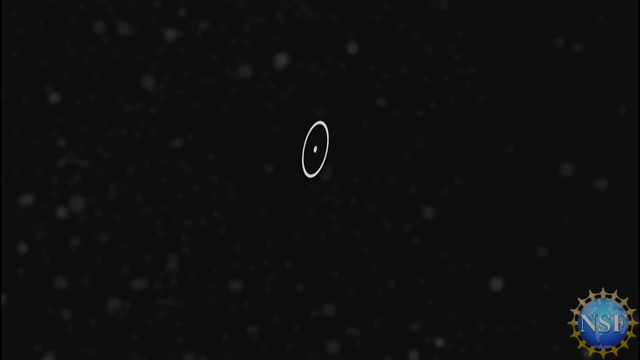 This cartoon is about an attempt to understand how these multi-messenger detections happen in space In total, to have a big picture. So, for understanding this picture, I would like to tell you that to date, there will be published seven papers devoted to this event, and I'm expecting that an avalanche. 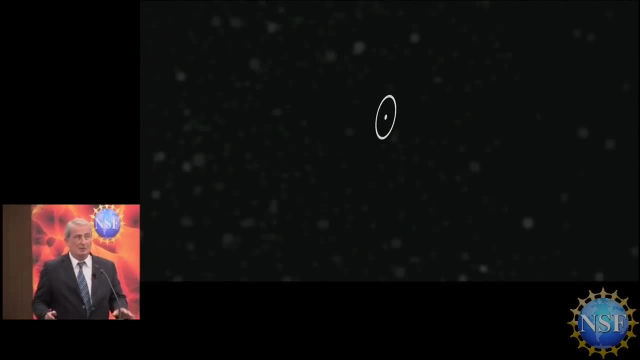 of papers will follow in the next times, but from these seven papers two will be published in the Science Magazine. There are five more papers, So it is an attempt of accompanying paper from a magic collaboration where we try to talk about the blazer, you see the jets of the blazer and then you can see zoomed in. 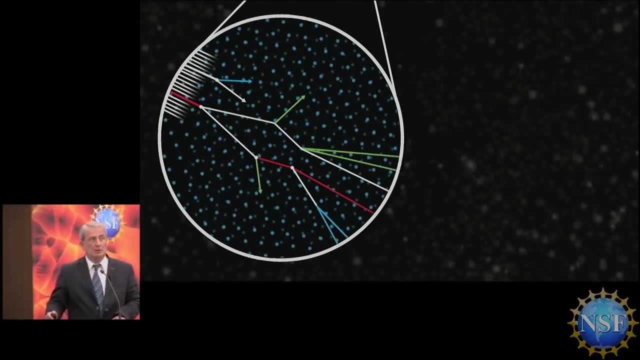 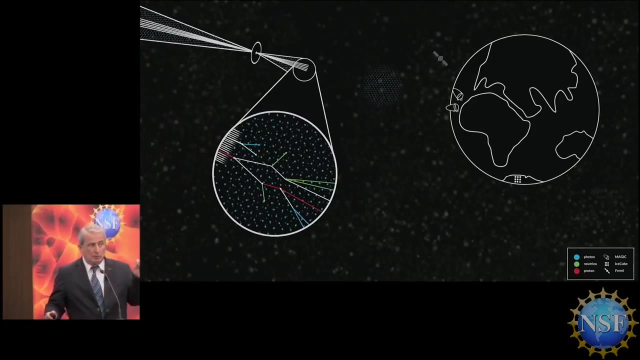 a jet And then, under special conditions, I think, you can have relatively low energy photons and these photons can interact with electrons and then, due to this interaction, so-called via inverse quantum mechanism, you can get gamma rays. but also protons are there and 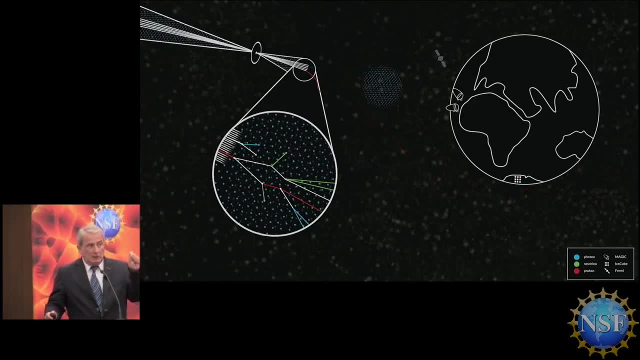 these protons can interact with these photons And then they can create via quantum production. they can create pions which will later indicate to neutrons. So you look to the picture. you see the red color as the protons and because of the charge, 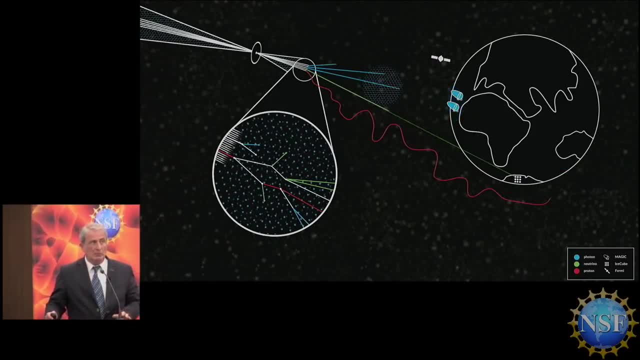 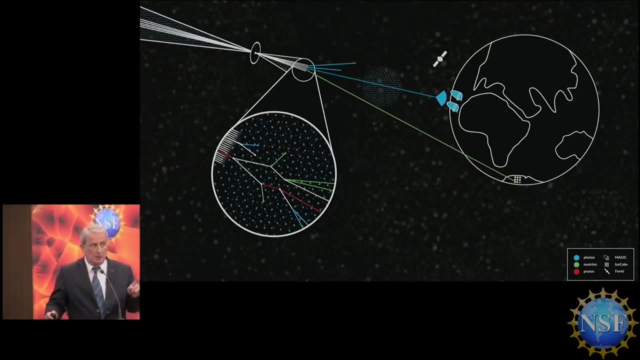 they move in a zigzag line so they're deflecting the magnetic, different magnetic fields. So when we measure protons we cannot say the incoming direction. but you pay attention to the green line. These are neutrinos which are detected by ice cover the South Pole and you pay attention. 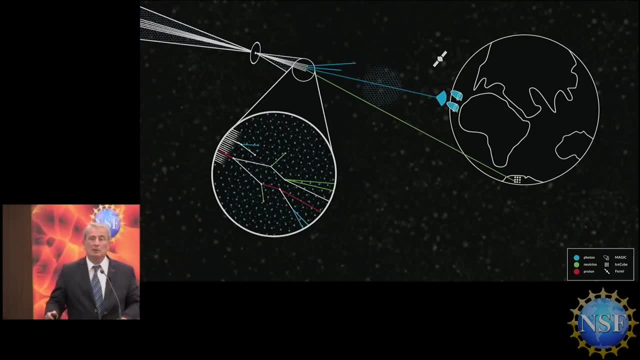 to the blue lines. These are measured by Fermi satellite and then magic telescopes. These are gamma rays. So I think we try to get a consistent picture and in this picture I think we can explain very well how it comes that we can measure simultaneously neutrinos and gamma rays in 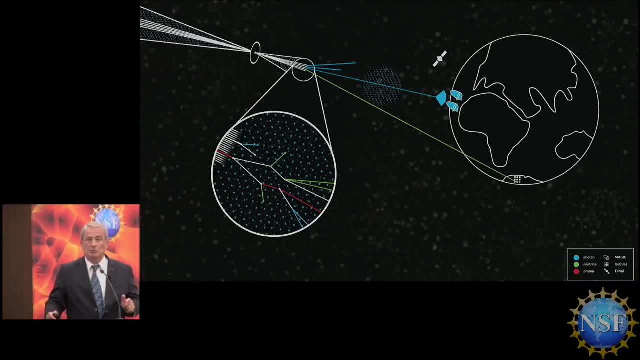 different energy ranges. And then, when you measure neutrino, neutrino is a smoking gun for a parent proton. And then, when you measure neutrinos, neutrinos is a smoking gun for a parent proton. And then, when you measure neutrinos, neutrinos is a smoking gun for a parent proton. 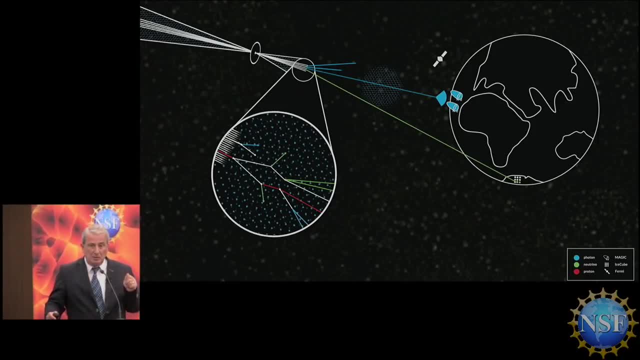 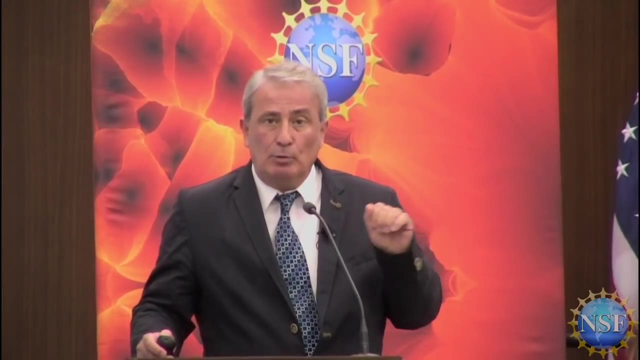 So if you measure about 300 TV neutrinos, it means that there is at least order of magnitude high energy proton. So these protons are in the jets of blazers and this seems to be the first time that we can say something serious about the longstanding question where the protons are accelerated. 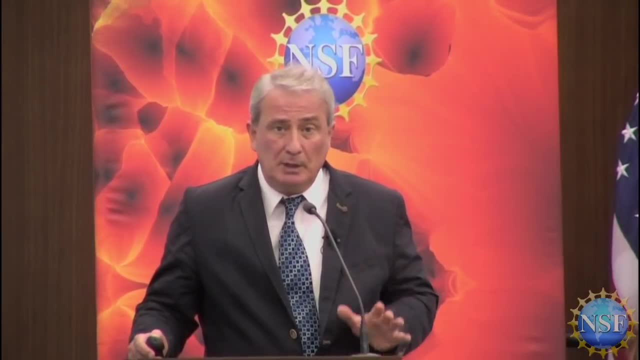 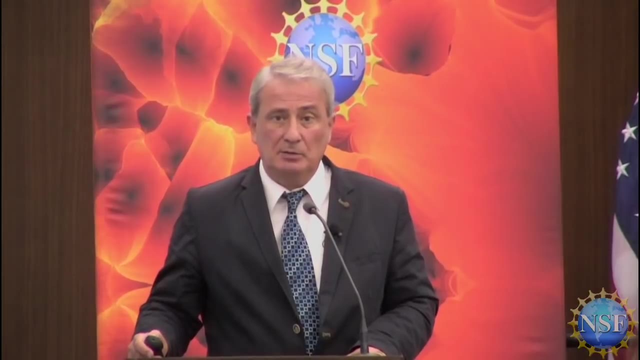 and protons are nothing else other than cosmic rays. So it means that the blazers can contribute cosmic rays at extremely high energy. So this is a very strong message And with this message I would like to give the word to my colleague, to Olga Boettner. 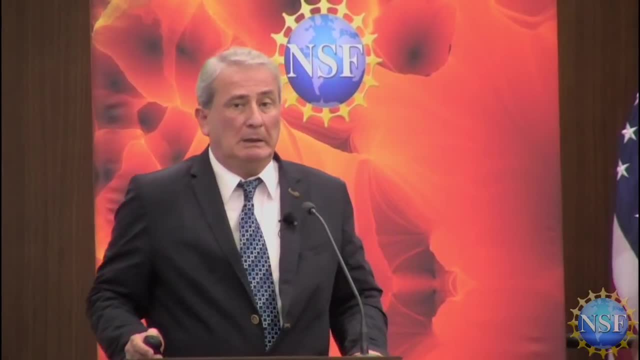 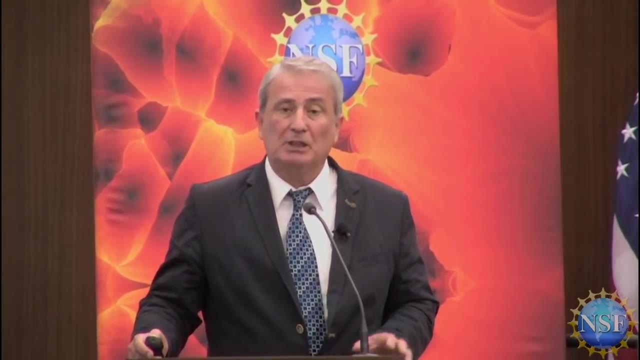 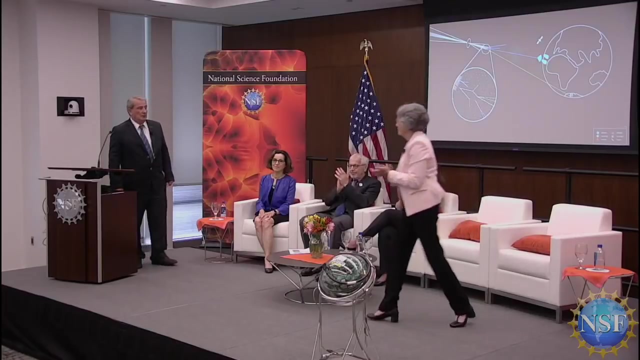 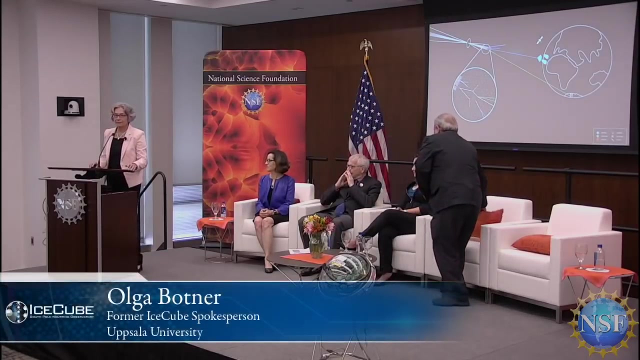 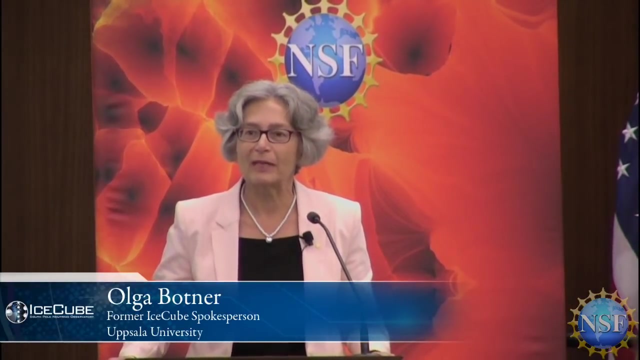 former spokesperson of IceCube Collaboration And she's going to present details of the accompanying paper of IceCube Collaboration, second paper in the Science magazine. Thank you very much for attention, So it's a great pleasure for me to stand here in front of you on behalf of the IceCube. 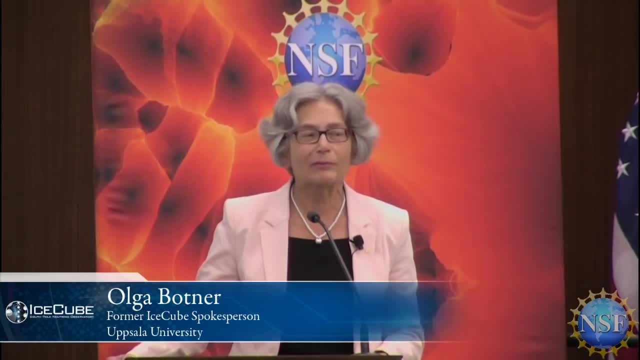 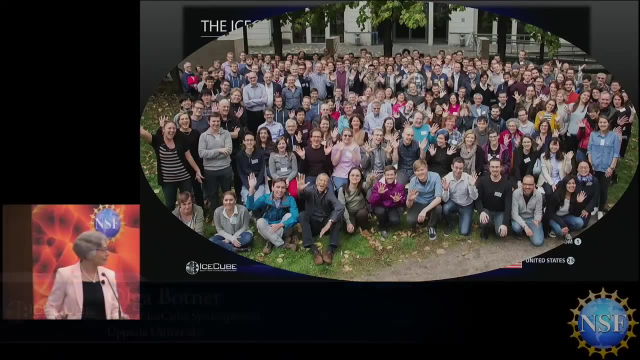 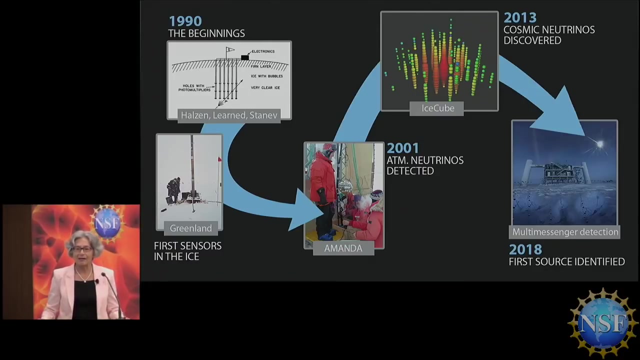 collaboration. 300 scientists from 12 countries around the world, on four continents, and most of them young and not gray-haired like Francis and myself. 300 sounds like a lot, but the number underscores the tremendous effort which has kept the dream of neutrino astronomy alive for the past. 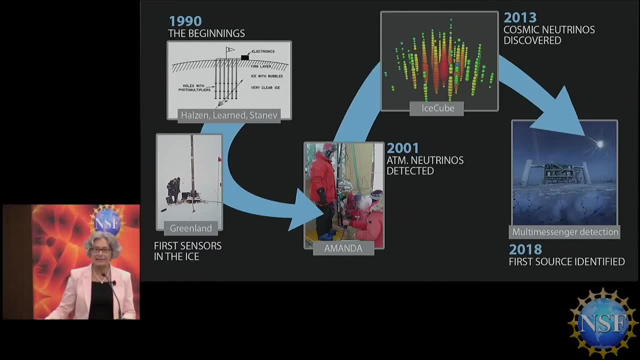 three decades, From the tentative beginnings around 1990, to the proof of concept with the prototype array at the South Pole in 2001,. to the breakthrough discovery of highly energetic cosmic neutrinos with IceCube in 2013,. to today's exciting news: the first evidence for a source of such neutrinos. 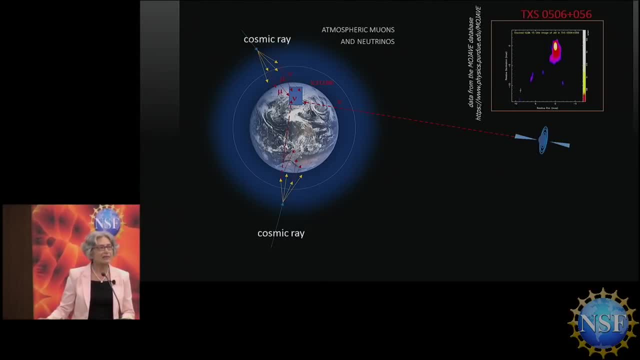 As you've heard several times today already, IceCube's September 2017 alert, in association with gamma-ray observations, pinpointed an astrophysical object named TXS 0506, and sometimes nicknamed the Texas Source, as the most likely source of these neutrinos. 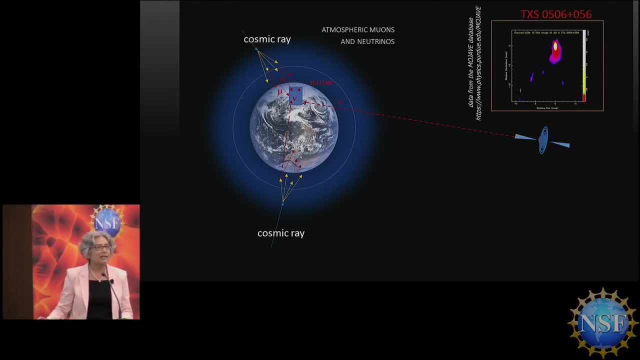 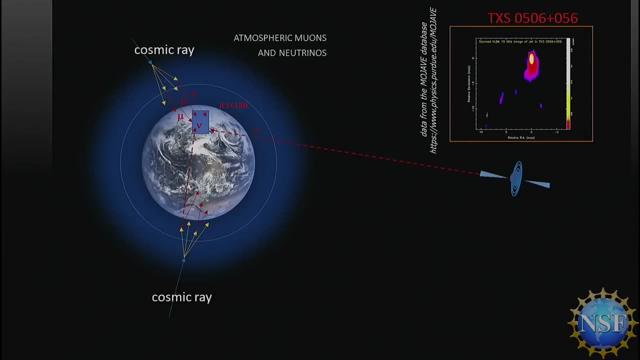 And what you are looking at on your right-hand side is a picture of the sky at radio frequencies, at the position of the blazer, And you are, as it were, looking directly along the barrel of one of the blazer jets. That's the bright white spot at the centre of the red blob. 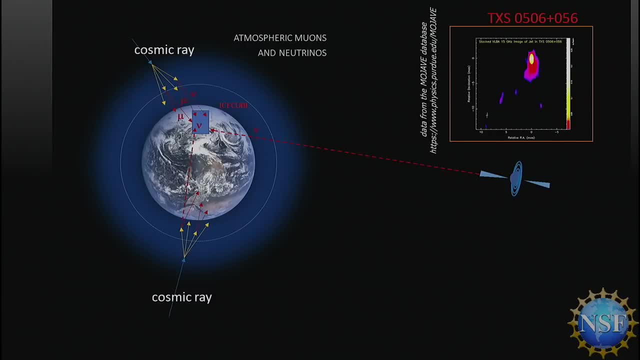 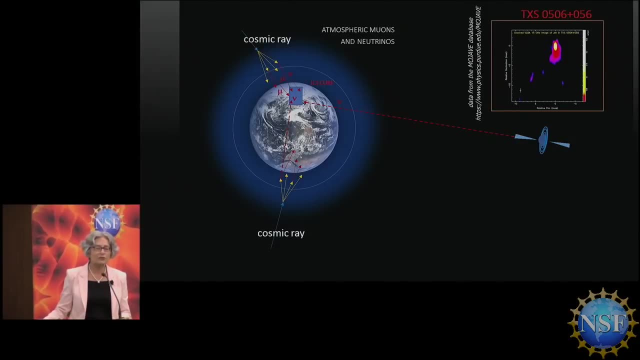 Now, intrigued by this revelation, we have determined to approach an eineuronic probe at the emailedinnue of the red blob. Now, intrigued by this association, we decided to look in our archival data to see if we could identify any more neutrinos coming at us from the position of this source. 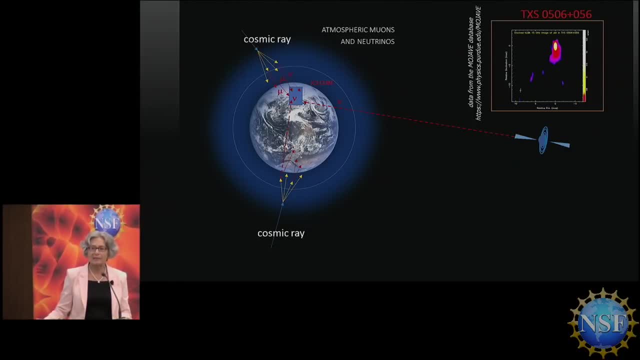 As you may know, iSKIP was completed in 2010,, but we had been taking data in partial configurations already for several years before that date, and so we had about 10 years of data to scrutinize And, amazingly, we discovered a neutrino flare centered on December 2014.. 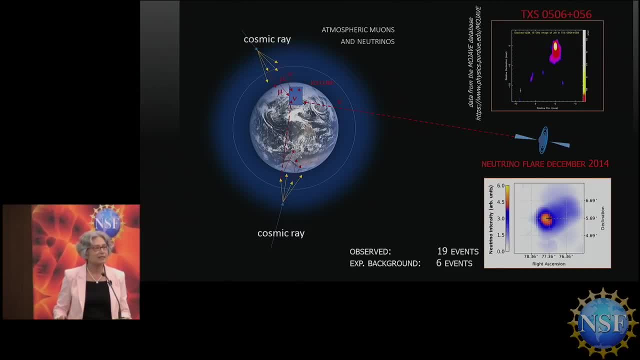 During a period of five months, we observed 19 events, where we expected about six events from cosmic-ray interactions in the atmosphere. This is an additional bit of evidence indicating that the blazar is indeed a source of high-energy neutrinos. Thank you, 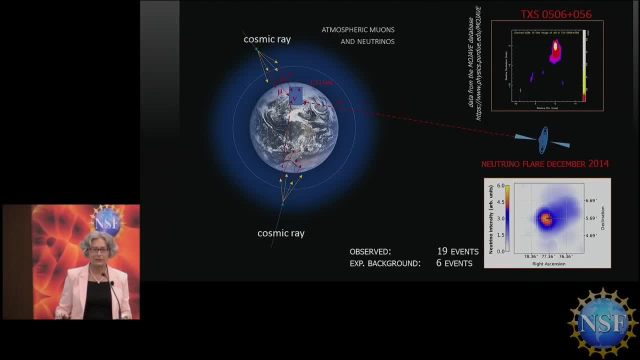 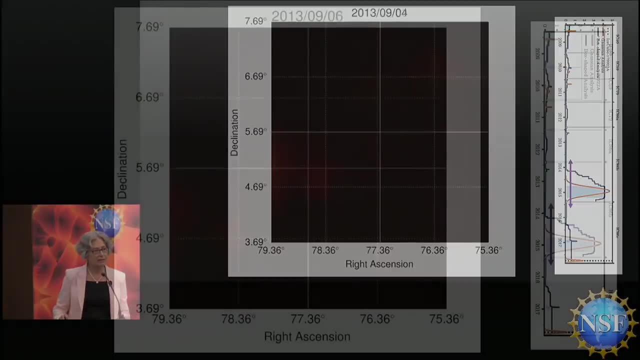 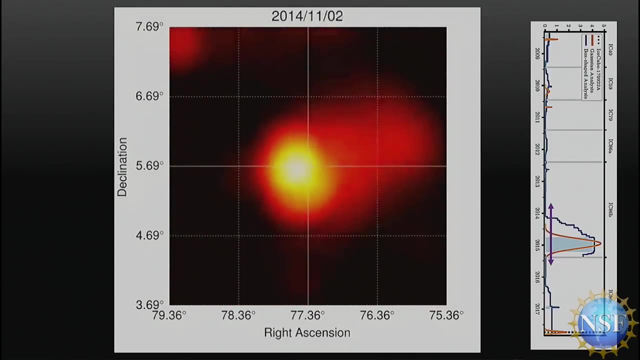 What I'd like to do now is to play a movie for you, a movie showing how the neutrino signal accumulates over the five months. So here it goes from nothing to a peak and disappearing again, And on your right-hand side you see a timeline with the neutrino intensity as a curve, and 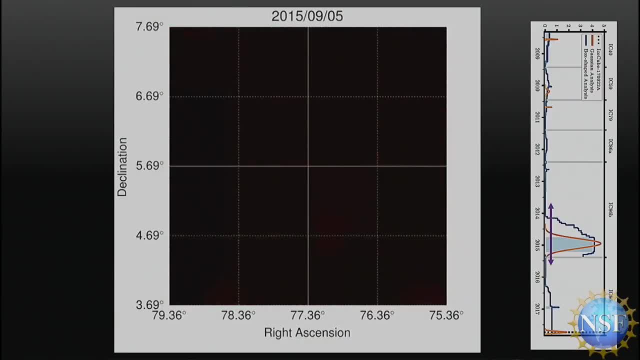 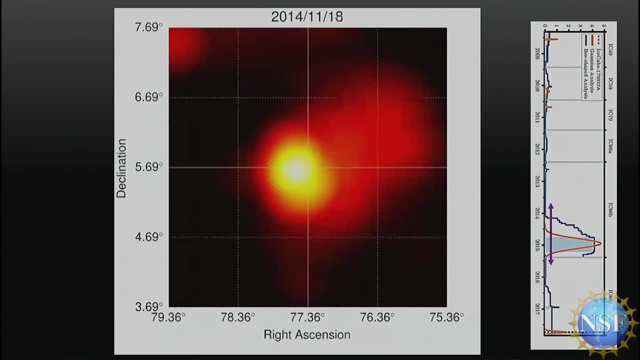 the arrow indicating the time interval of this movie. I want to just show you the intensity at the peak of the flare Again. so this white spot, the bright spot in the center of this sky map, at the position of the TXS, is the neutrino flare. 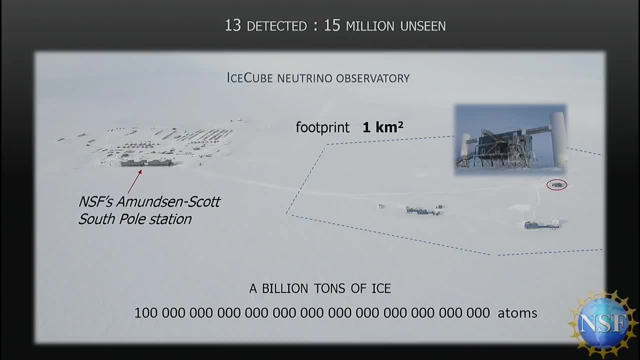 So, as I've just told you, we detected 13 neutrinos which we believe are signal from the direction of the Texas source in the 2014-15 flare. During these five months, 15 million neutrinos were detected. That's a lot. 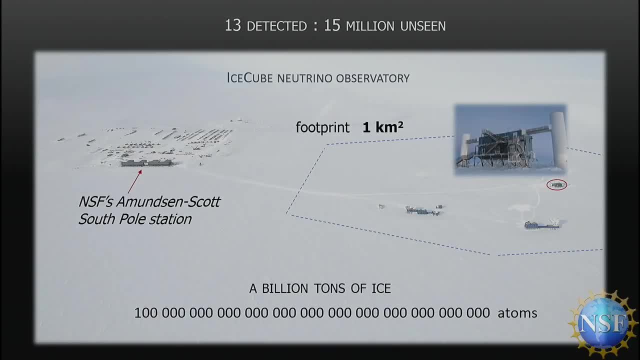 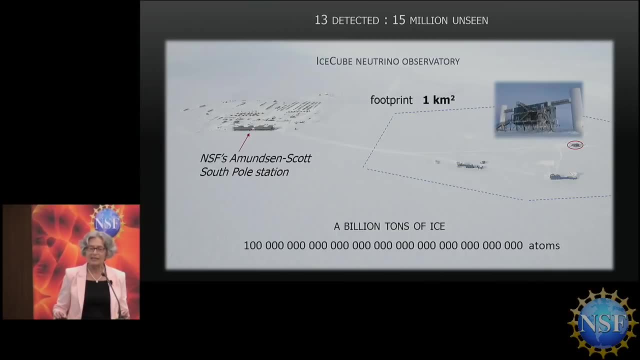 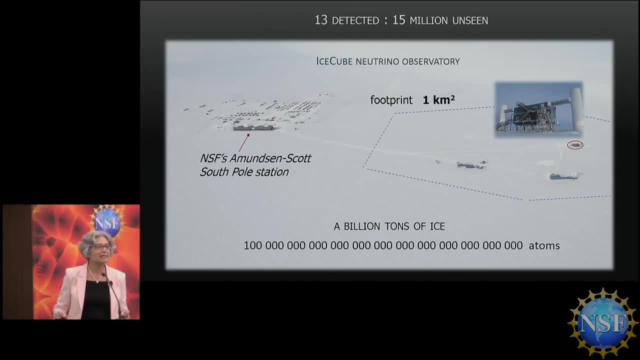 A neutrino is invisible unless it collides with an atom, And this happens very rarely, And so you need to monitor tremendous lot of atoms to stand a chance to catch a neutrino. IceCube at NSF. Amundsen–Scott is close. 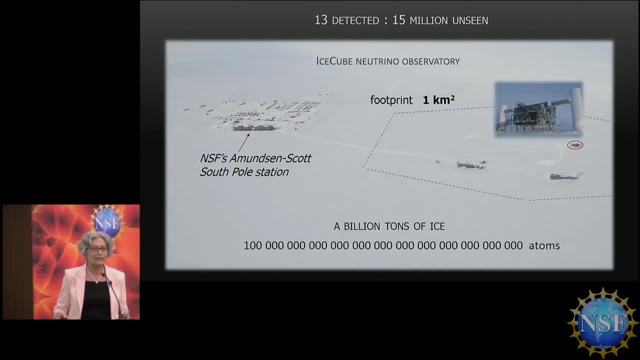 South Pole Station instruments: a volume of one cubic kilometer of the clearest glacier ice. This is a billion of tons of ice. 10 to the power, 38 atoms- This is a one, followed by 38 zeros. On the left-hand side, you see how the ice cube. 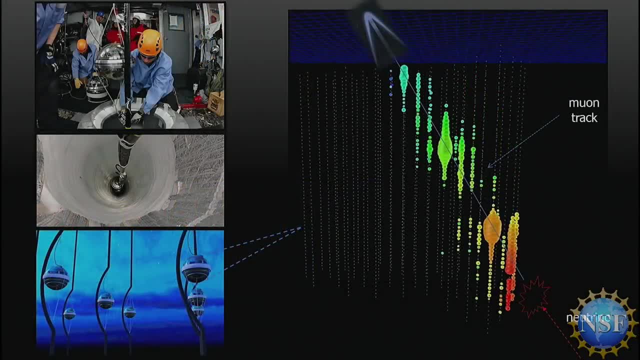 sensors like the one which is standing in front of you on the podium, attach to cables deployed into vertical holes drilled by means of hot water and left to freeze in in the ice. On your right hand side, you see a neutrino coming from the bottom right colliding with an atom, producing a charged. 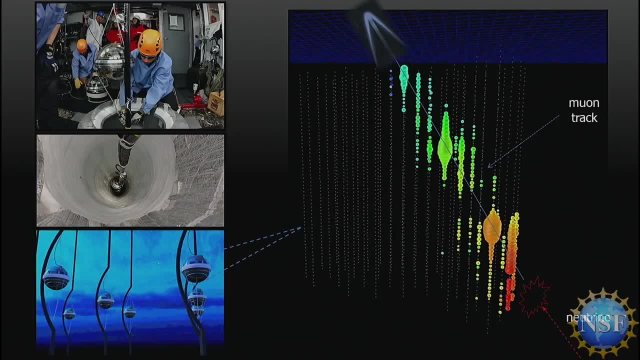 particle, which is called a muon, which then moves through the entire depth of the detector, trailing a cone of blueish light, And it's this light that our sensors detect. Now, the colors you see in this picture are the light that's being donated to our sensors, and the colors that are 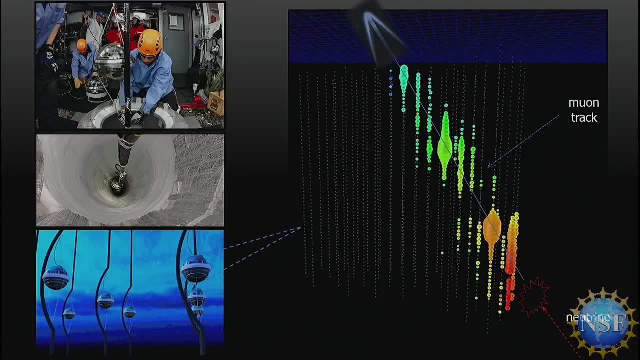 not the colors of the light, but they illustrate the time sequence of the signals we observed, with the reds and oranges being early and the greens and blues late. So, as you can see for yourselves from the time sequence, we can reconstruct the direction of the muon and hence the direction of the neutrinos. 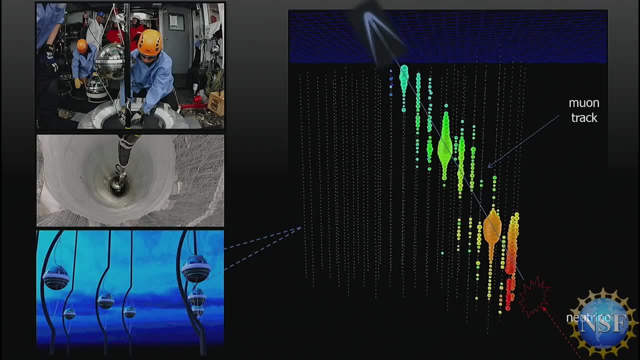 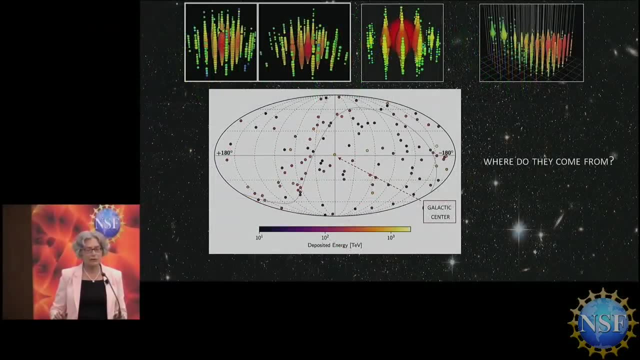 So this is how we know that the neutrinos we observe come from the TXS source. In 2013,, IceCube made a breakthrough discovery of a diffuse flux of highly energetic astrophysical neutrinos. Since then, we have observed a couple of hundred such events and what you see in the upper panels on this: 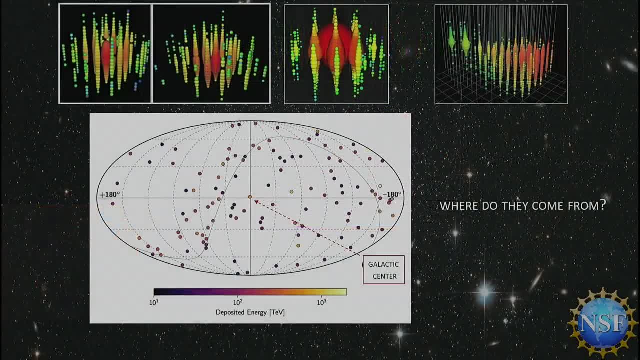 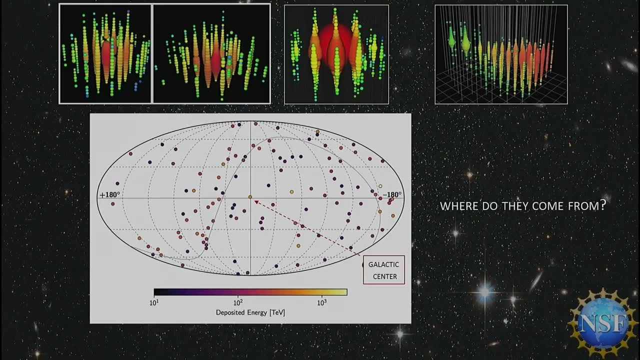 slide are the four highest energy neutrino events ever observed on Earth. What you are seeing is not the neutrinos themselves, but the light images as they are recorded by IceCube, and to give you some kind of feeling for the dimension, think in terms. 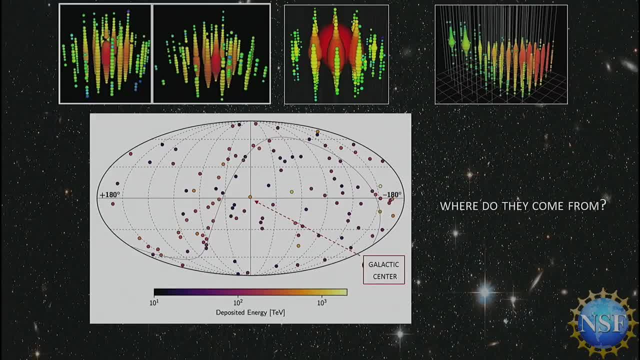 of hundreds of meters or kilometers. On the picture below you see the directions of these high-energy neutrinos distributed over the sky and, as you can see for yourselves, there is no obvious accumulation of directions. So the million-dollar question has since then been: 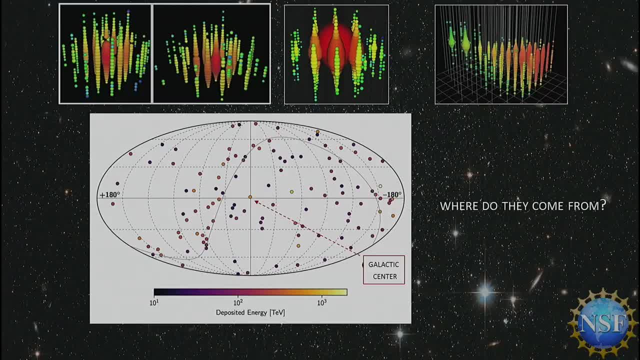 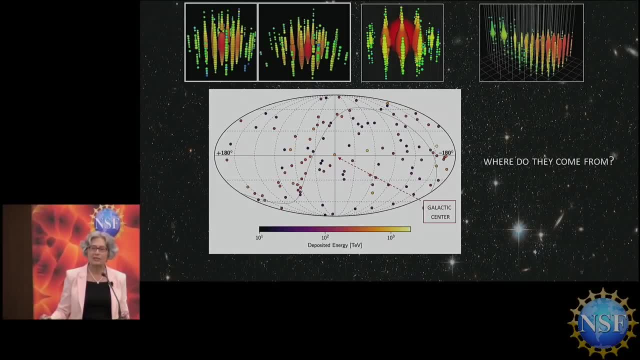 where do these neutrinos come from? And for the neutrinos we're reporting on today, we know the answer. We needed electromagnetic observations to assess the association of the September 2017 alert with an astrophysical object. The neutrino burst in 2014-15 strengthens this association, and so the bits of the 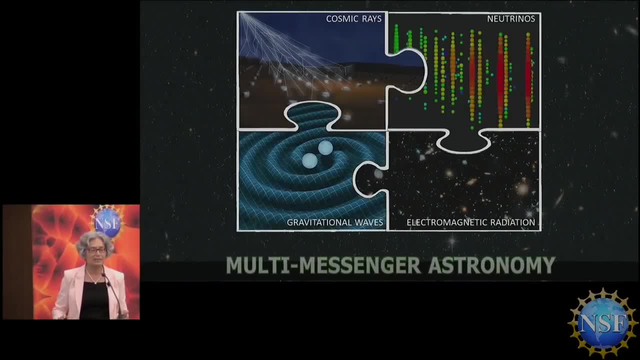 puzzle are starting to fall into place. For the first time, we have been able to associate high-energy neutrino emission with a high-energy gamma-ray source. This is what we've been waiting for. This is the first evidence for high-energy cosmic accelerator, a pivotal moment for multi-messenger astronomy. 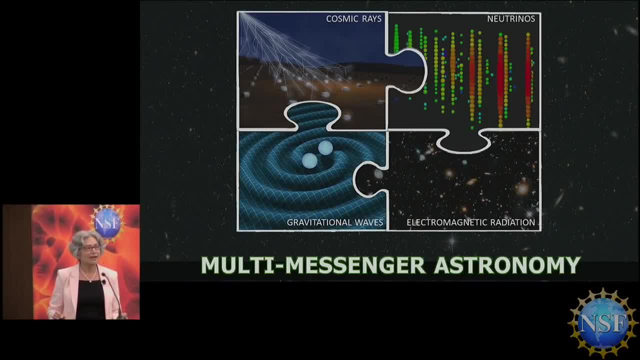 Now, as you see in this graph on your left-hand side, in the bottom corner, I show also the gravitational waves And, as most of you know, we have not identified neutrinos in connection with gravitational wave events yet, But we believe that this is. 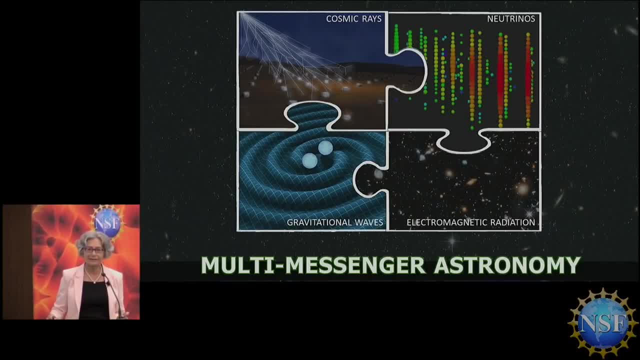 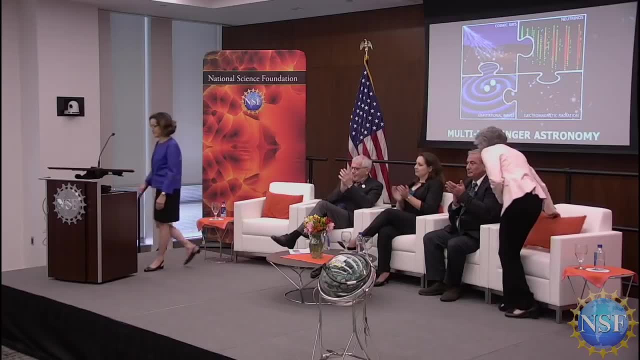 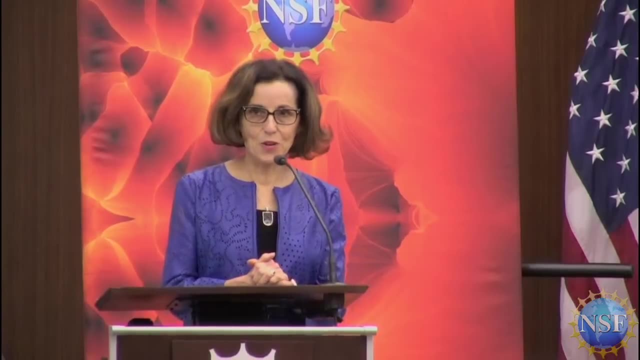 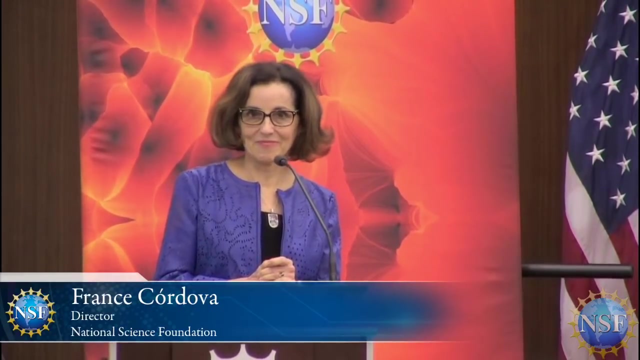 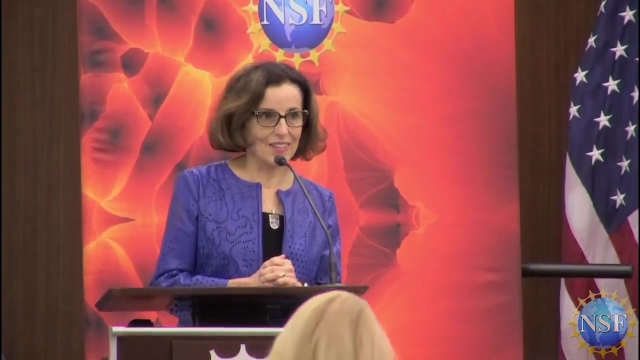 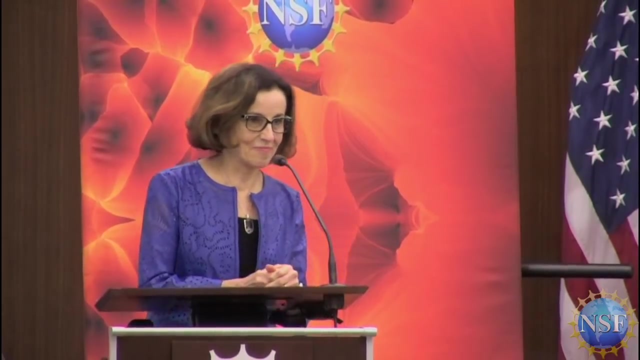 the discovery waiting for us just around the corner. Thank you. Well, there you have it, So now we're open to questions. Hi, This is Emily Conover from Science News. I wonder if you could talk. you know you've. got one neutrino now that's associated with the high-energy space and that's associated with the high-energy world. That's a big thing, And so the question is, what is the relationship between the two? And you know, the first thing that I'm going to ask is: how can we? 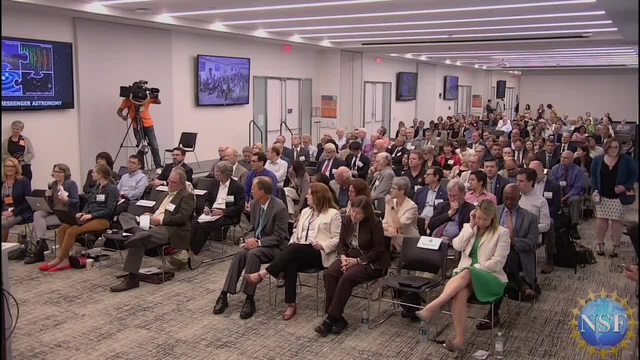 get the distribution of the two. And then the second thing that I'm going to ask is: how can we get the distribution of the two? And so we have a very interesting question and I'm going to ask with this Blazar, what's sort of the future? 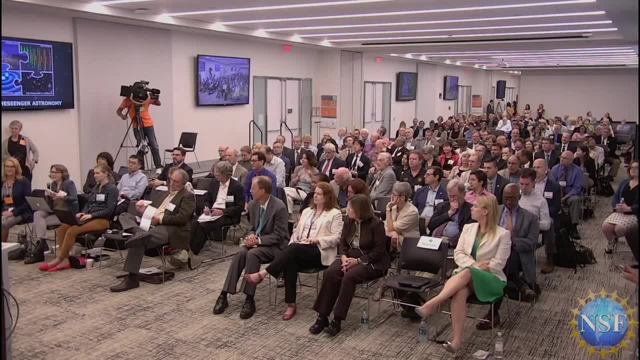 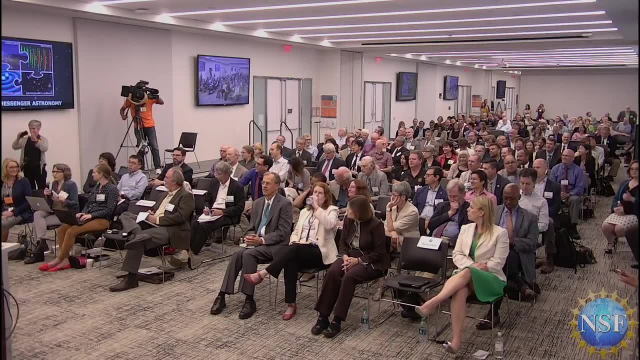 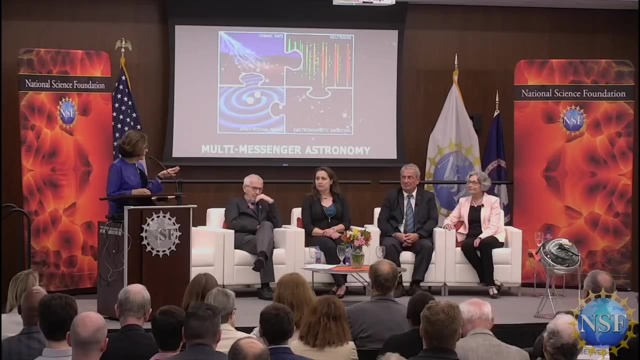 of this kind of work, How soon can we expect another one? I mean, obviously that's hard to predict, But are there any plans for future upgrades that might increase the rate, things like that? OK, well, first I'll have Olga. just clarify that there's. 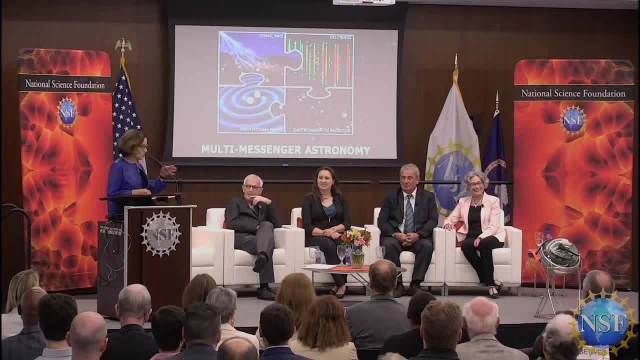 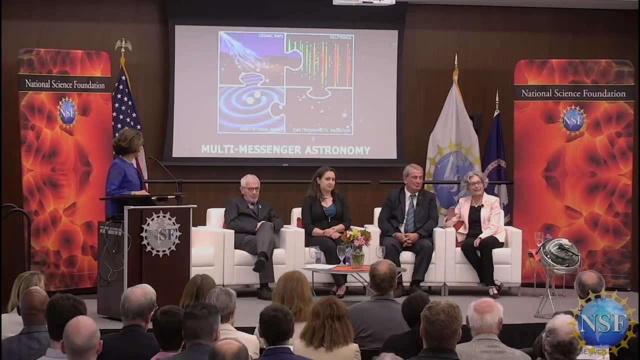 actually more than one, And then ask Frances to address your question. Yeah, so just to make it quite clear, there is two papers published in Science. One is the paper about the 2017 alert And this is one high-energy neutrino pointing. 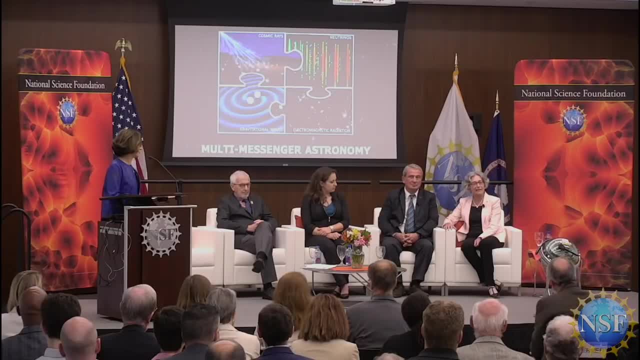 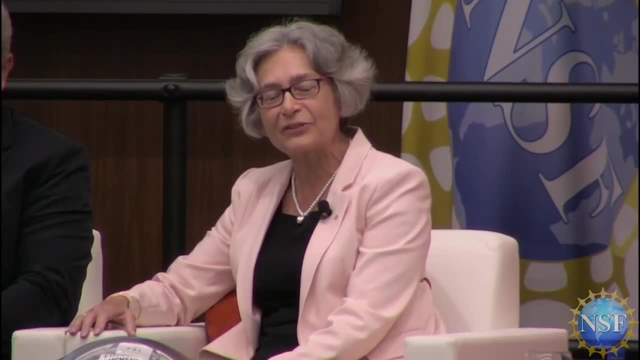 at the spot in the sky, But then in our archival data we have more than a dozen neutrinos coming at us from the same direction. So we have actually a handful of neutrinos from this object, And this is why we are confident that this. 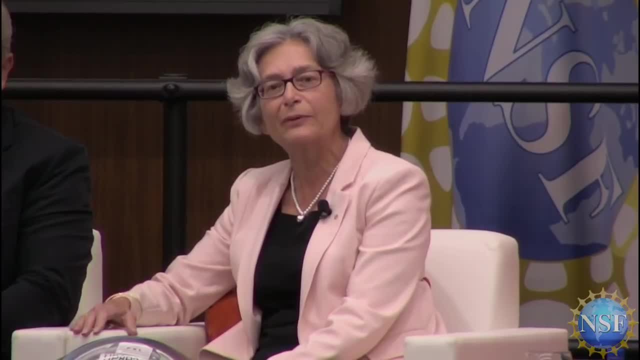 is a source of neutrinos And a probable accelerator of high-energy cosmic rays. Now about what we would wish for the future. this is, of course, a good question, And I've tried to explain that neutrinos are very, very. 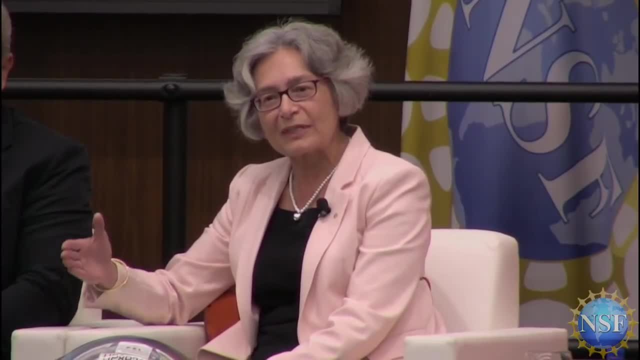 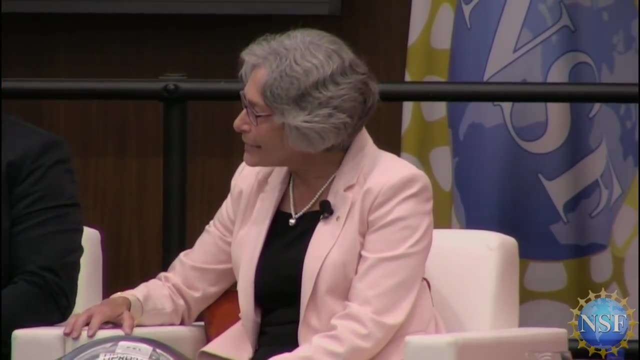 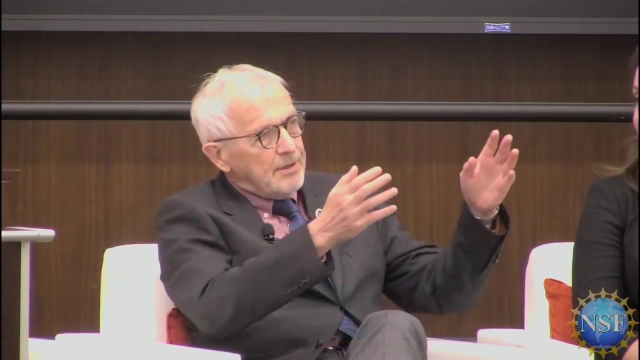 difficult to catch. So to get more, you need a bigger detector, And I let Frances continue on that. Well, the short, direct answer to your question is: you saw it actually on one of Olga's plots. In the last nine and a half years we saw two birds. 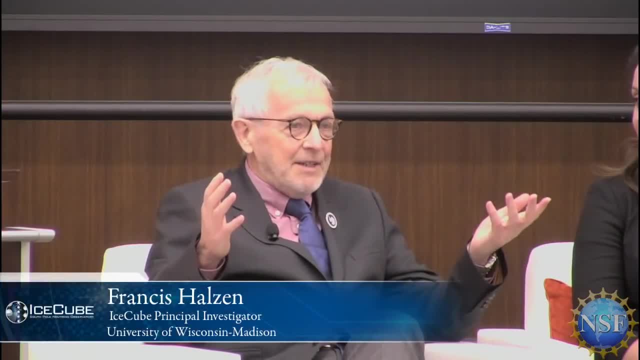 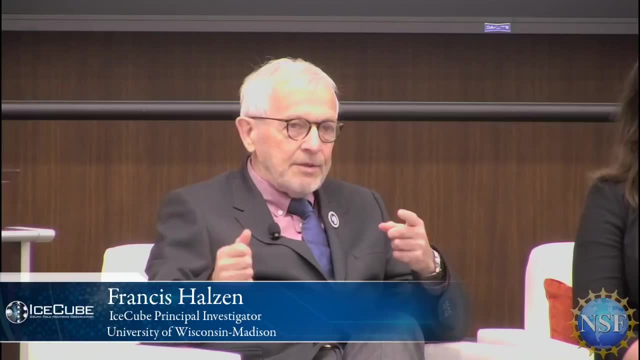 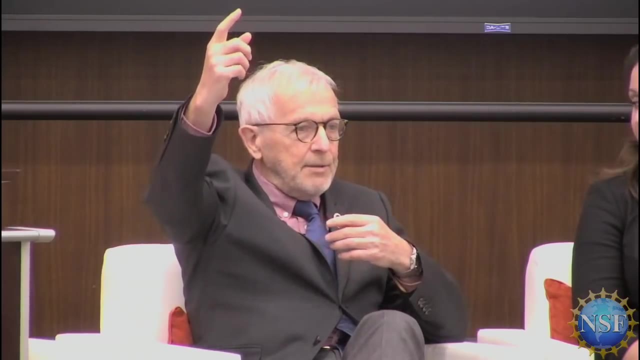 And that's the only information we have right now to predict when we'll see the next one. The key, I think, is this source is very special, Because why do we detect the first source 10 times further away when there are very nearby sources? 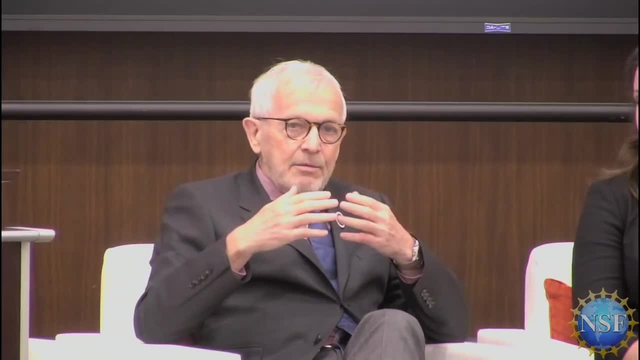 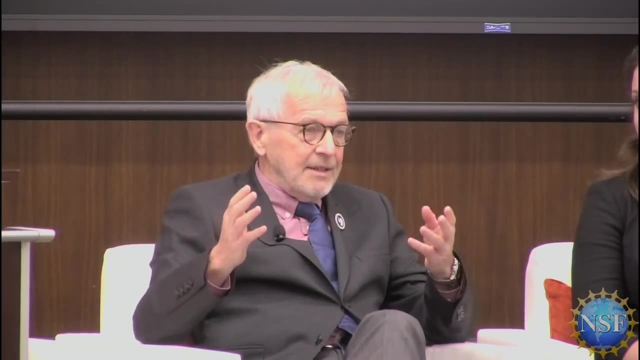 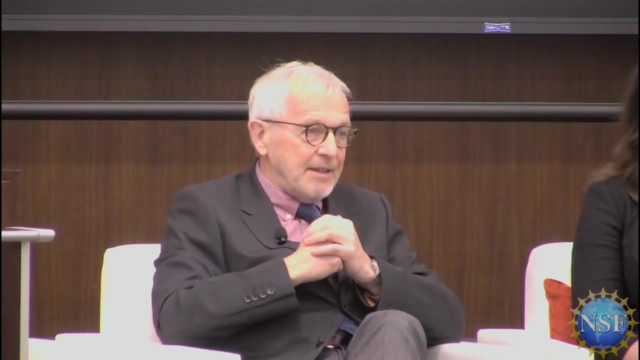 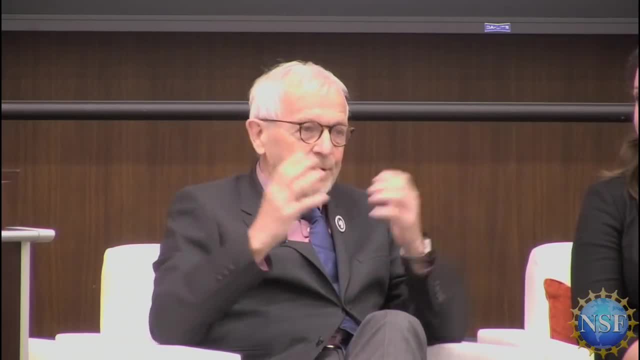 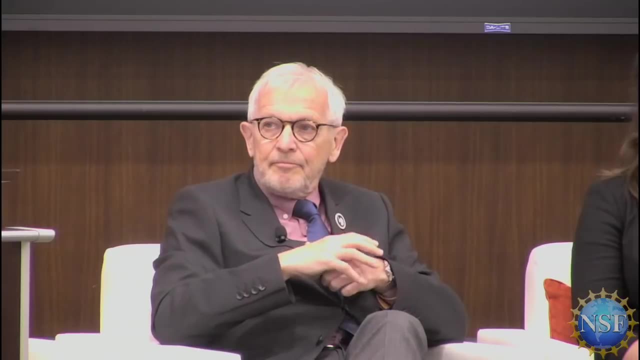 But, as usual, the work has just begun. Frances, are there plans, just following on that question, are there plans to make the IceCube observatory bigger? Of course That's the answer she wants, And I'll just add to that: you also? 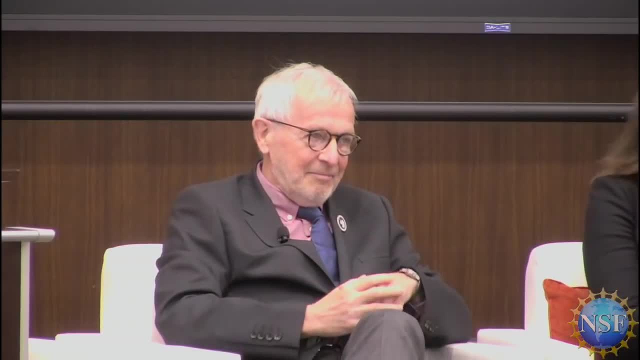 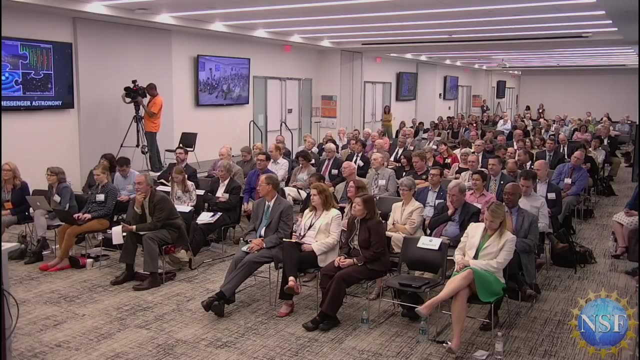 want to keep continuing to monitor other high energy particles like gamma rays, to have these joint detections, Because that's so. you want to continue to monitor the gamma ray sky as well? Great, And once LIGO is up and running again. 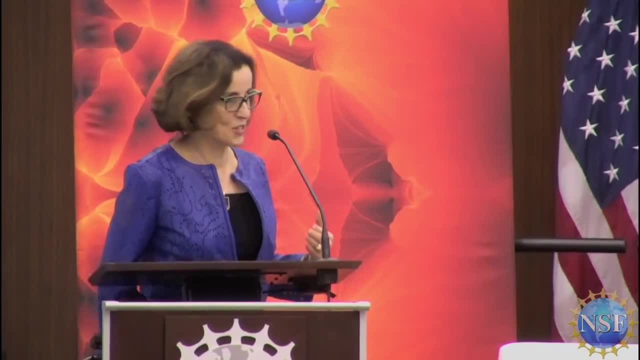 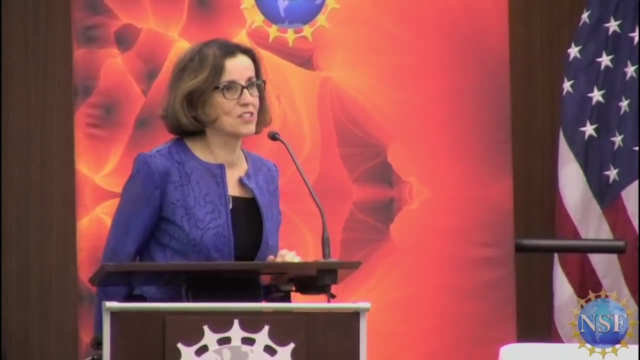 right now it's being refurbished to have higher sensitivity, which is really important in these things. Then we can see, as Olga said, there's going to be, as I said, the last piece of that puzzle falling into place in multi-messenger astronomy. 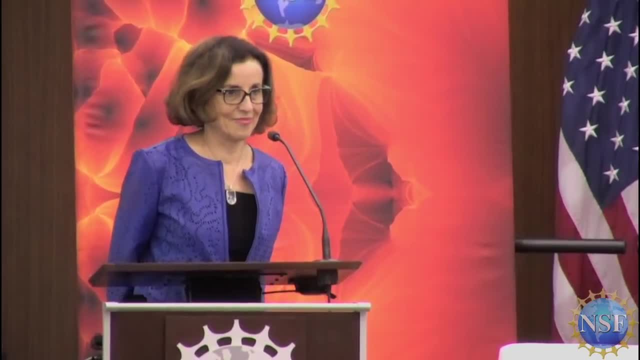 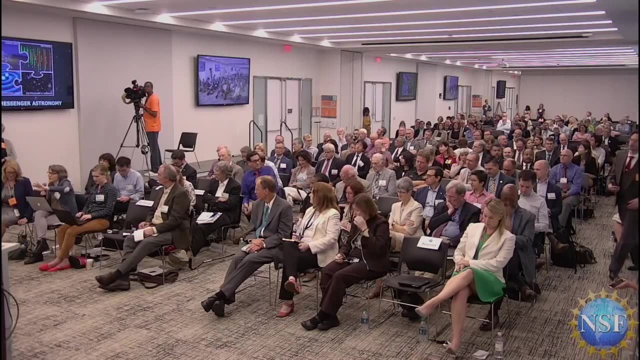 Another question, please. We have a follow up. Sorry, So I just wanted to ask about the. so when you look back in the data and you see the neutrinos, this handful of neutrinos, is there any evidence of a gamma ray? 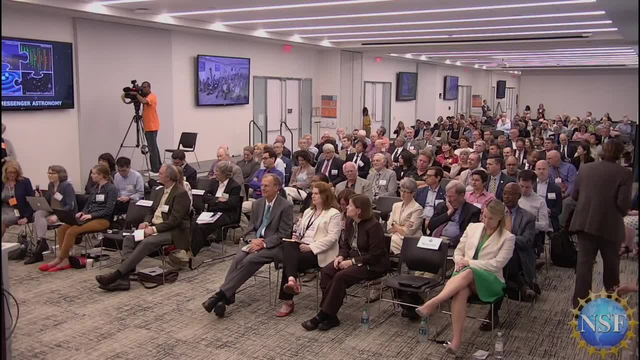 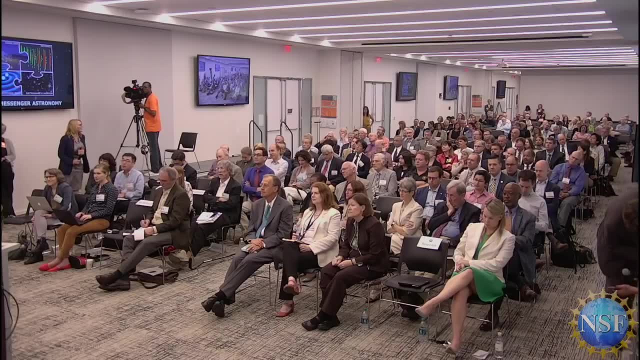 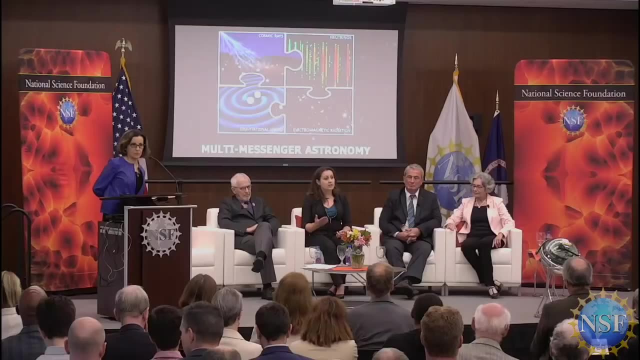 flare at the same time, or anything like that. So there's two things you basically have to look for: The number of gamma rays and the energy of the gamma rays, And so at the time of the neutrino flare, we didn't see an increased number of gamma rays. 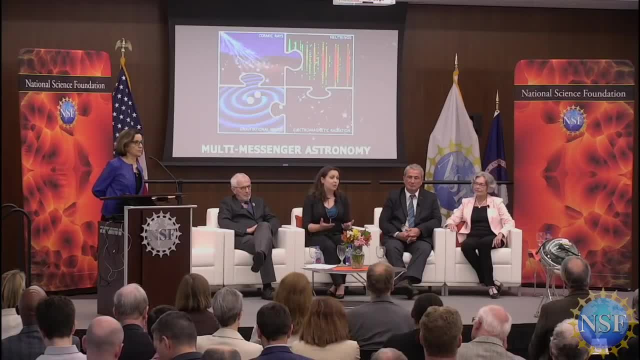 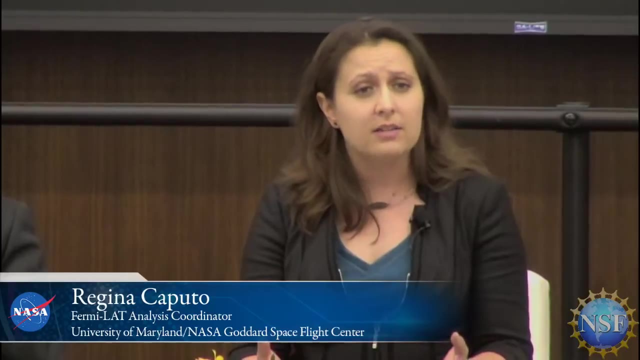 But there is some evidence to indicate that we saw an increased energy in the gamma rays Because they're produced at the same time. the same process that produces neutrinos also produces gamma rays. That's why the energy is also important. So we didn't see an increase in the flux, which is why 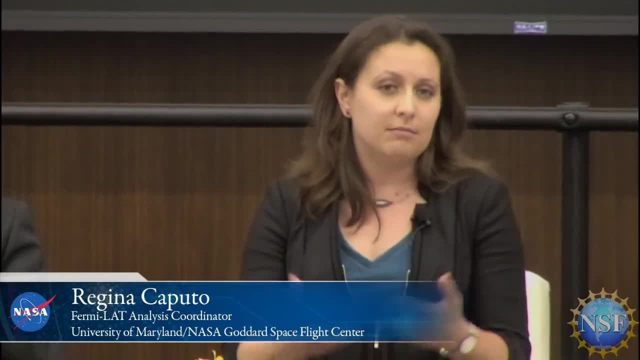 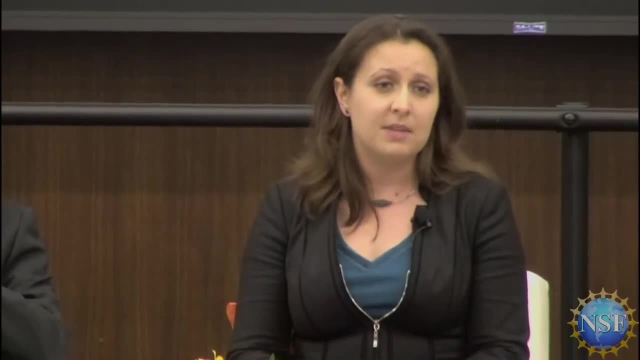 and we didn't have an alert. We didn't have an alert from IceCube, But also Fermi. all of the data is archived, So we can go back and look at the data and see what was happening at the same time. 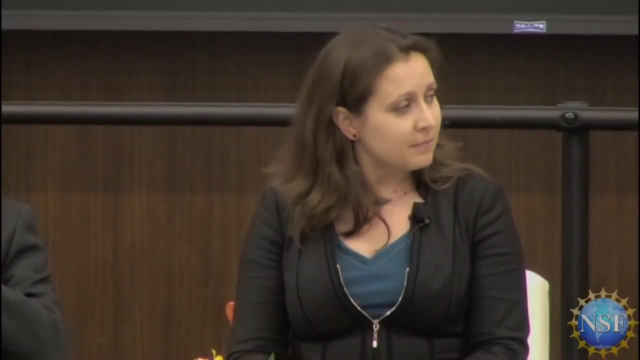 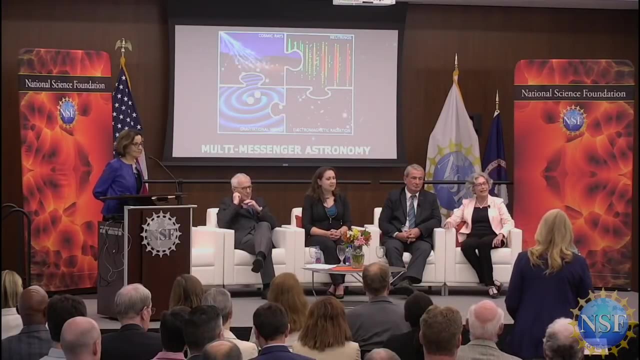 May I just add a sentence. I mean, this is actually very exciting. It's not clear cut science. We are learning about the blazes as we go. They don't you know. it's not as it was predicted. It's not as we had expected. 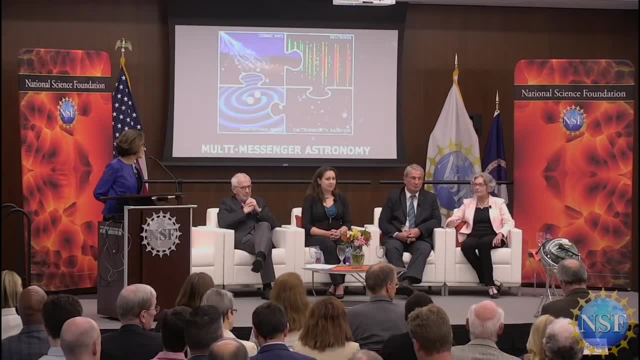 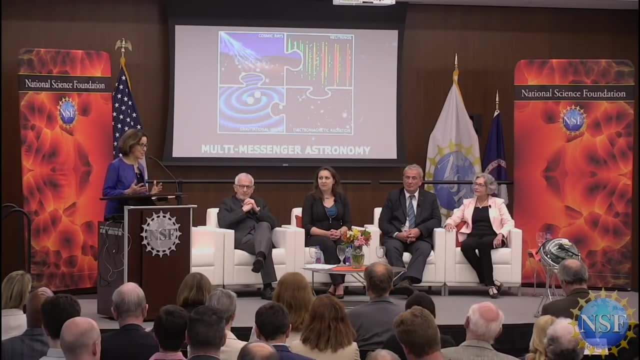 There's more things going on And we are learning new things. So this is just the beginning, just as, Dr Cormier, The physics of jets- just so you don't think that that's all been figured out is- really has a lot of mysteries in it. 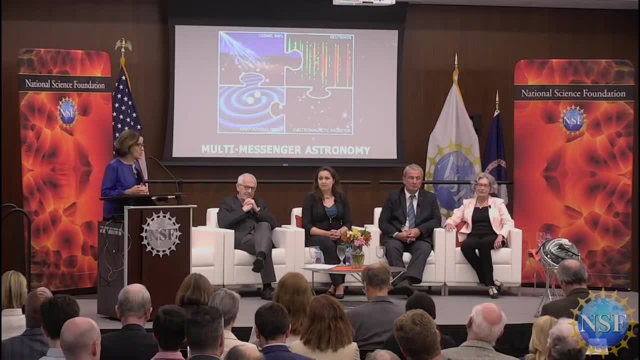 And this is another piece, as August just said, of the puzzle of how do particles get accelerated to these tremendously high energies in these kinds of environments And, as I said in my opening remarks, this is so much higher energy than what we can produce. 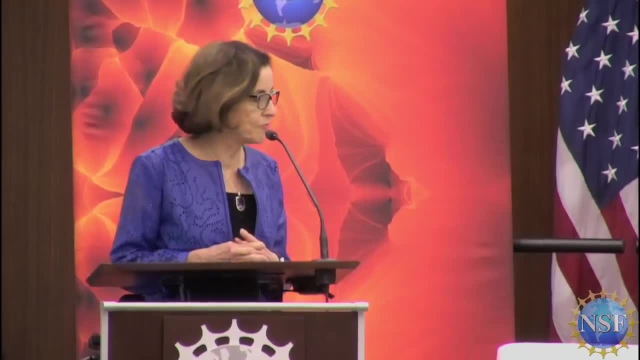 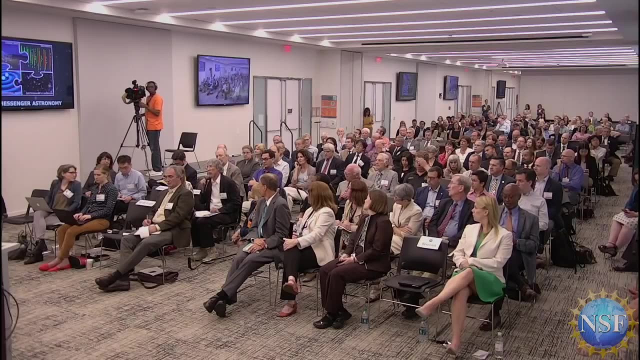 This is so much higher energy than what we can produce on Earth and our best accelerators. Another question: Yeah hi, Arthur Friedman, the Yucca reporter. So I'm wondering: are the neutrinos traveling at the speed of light? 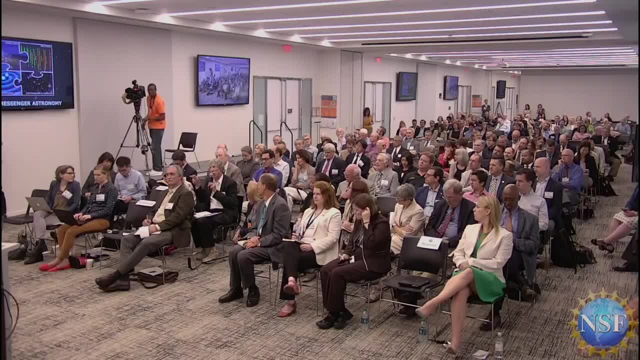 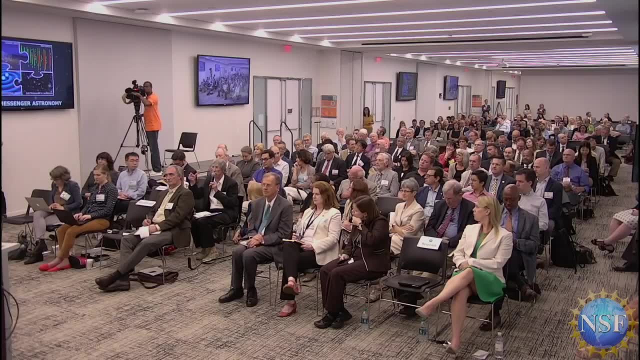 And the other part of the question is: if they were in a gravitational wave, would the gravitational wave accelerate them even faster Or are they already at the maximum speed? I was just trying to understand the interaction if they were a part of a gravitational wave. 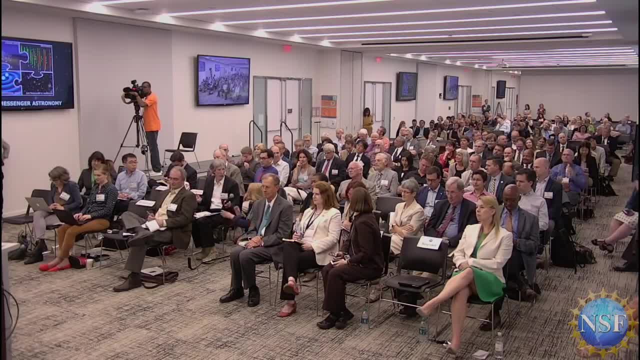 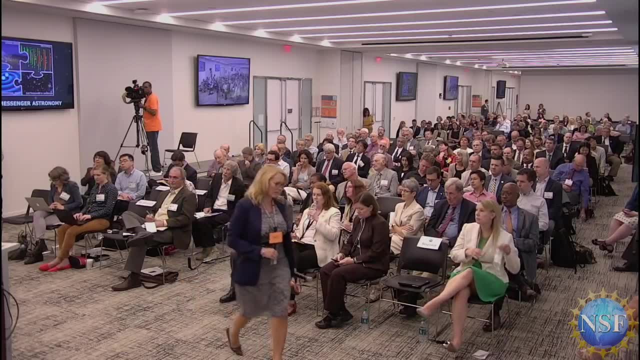 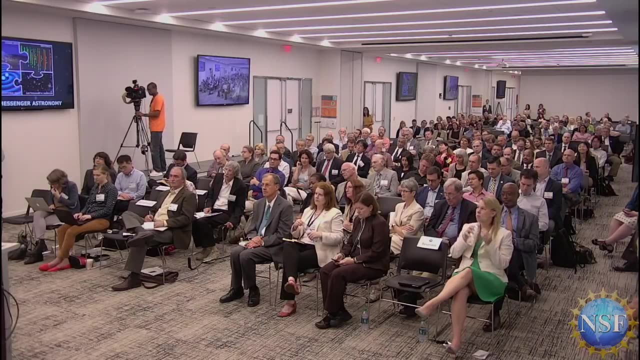 But undetected so far, Francis? No, I mean when we say they travel at the speed of light. of course it was a major discovery in 98 that neutrinos actually have a small mass. But this mass is so small compared to the energies. 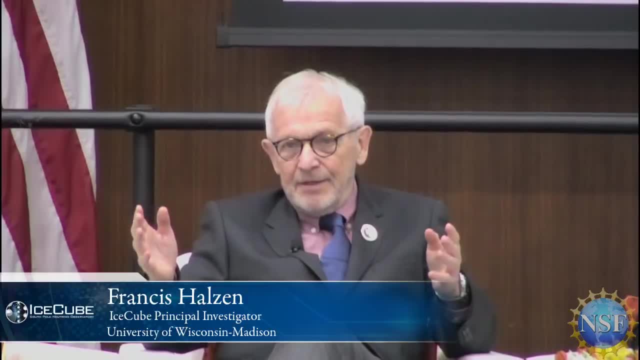 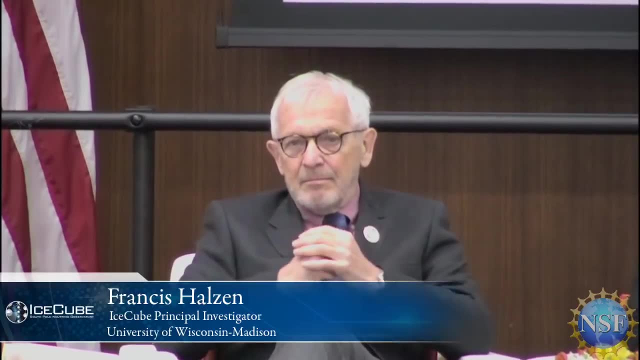 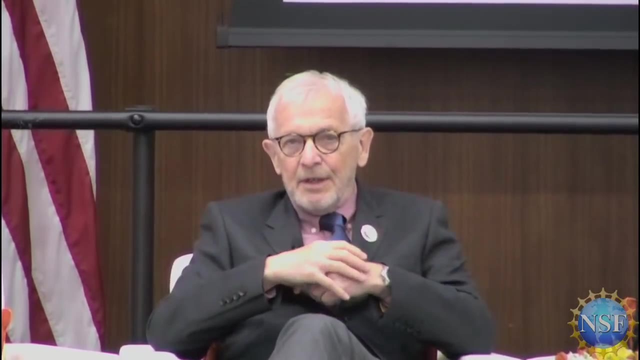 IceCube is observing. it's totally irrelevant. So neutrinos are basically like photons, And so there's no difference. I don't know if this answers your question. I'll give you an example of an event where we would see neutrinos in gravitational waves. 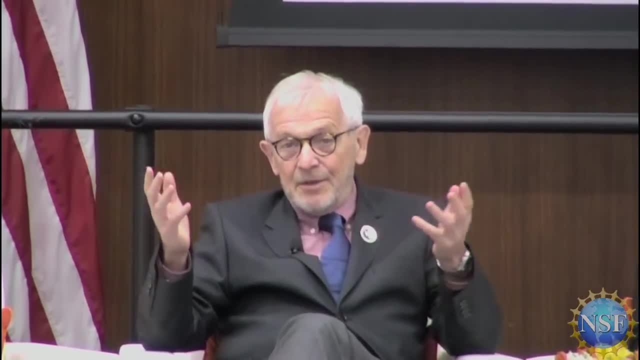 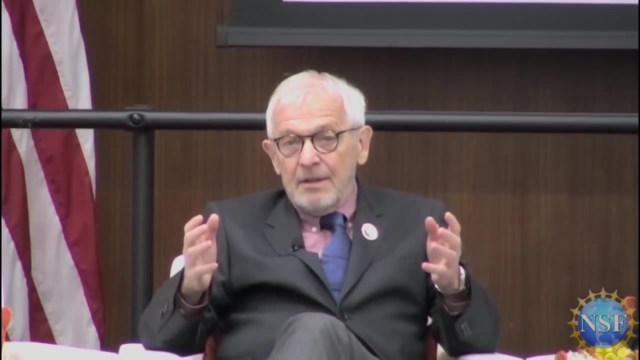 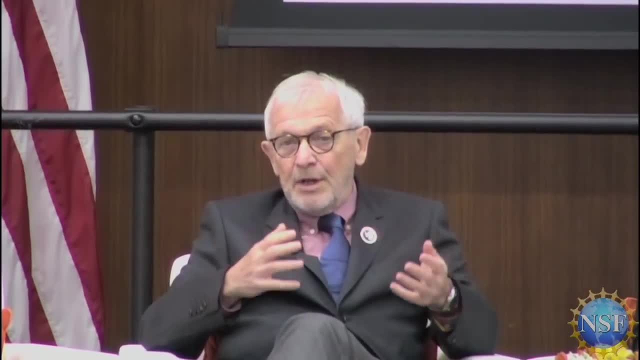 And I think that's what we're trying to do. And I think that's what we're trying to do, And we know that we can see neutrinos. So that's one case: The neutron star merger, which is still on the screen. 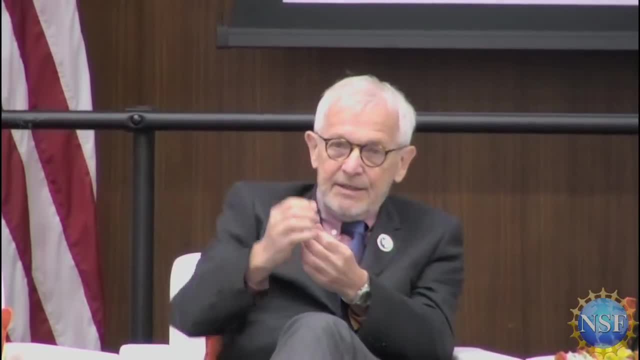 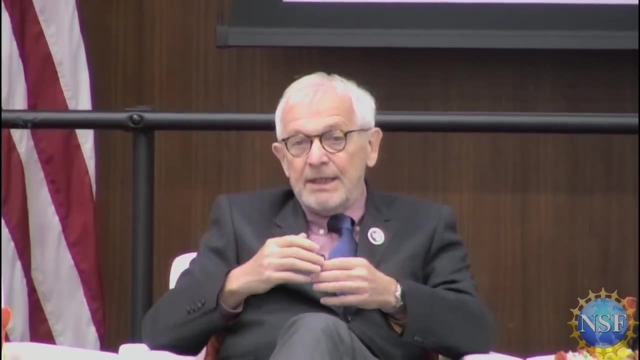 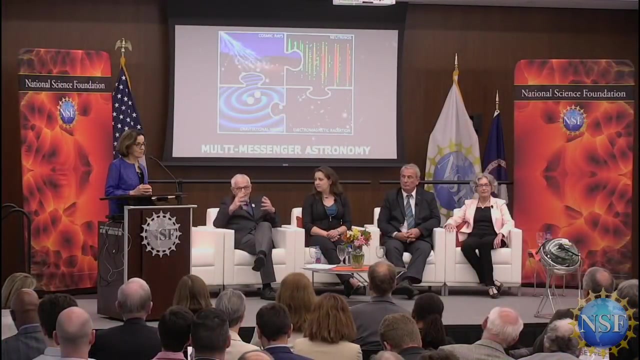 actually makes jets. when they spiral in, A jet is formed which is very similar actually in concept to what we are talking about here, And presumably this source emits neutrinos in some similar way, Some similar mechanism than the blazars. 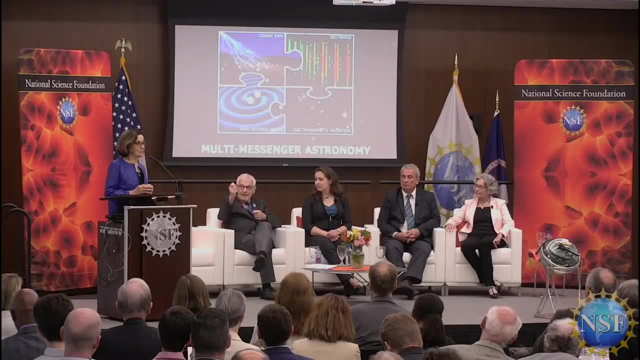 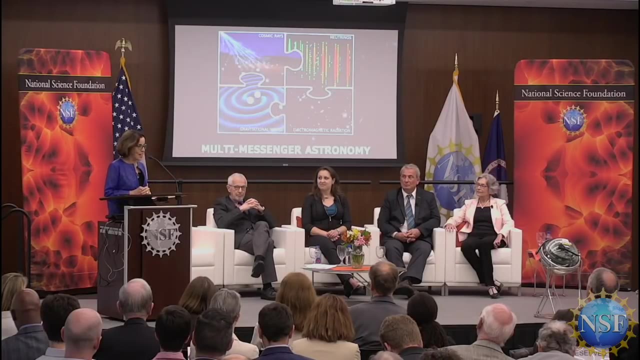 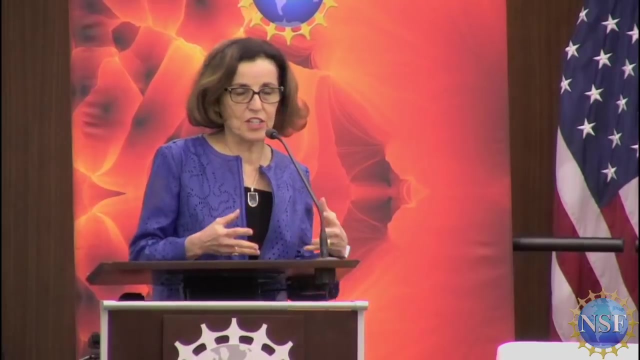 And of course the jet in that event was seen in gamma rays. So Razmik showed an illustration of the first cosmic neutrino detection of supernova 1987A, And we didn't have gravitational wave detectors at that time. So it's all just coming together as the technology increases. 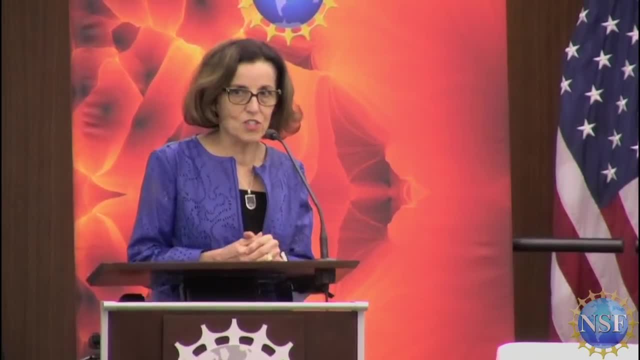 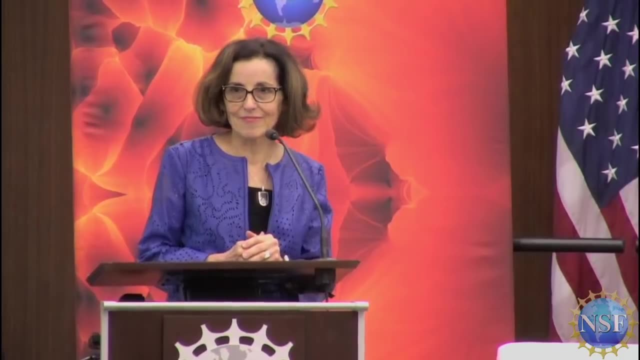 and we have more opportunities. So it's all just coming together as the technology increases and we have more opportunities to do these multi-messenger observations. Another question, please. So you're all ready to take an exam on this? You know what's up. 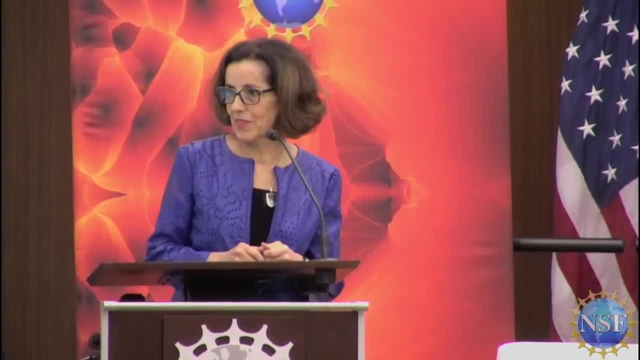 I have a question from the web. From the web, OK. In light of the breakthrough results from small-scale high-impact experiments like Q-Week and EDGEs, why does NSF invest in expensive projects like IceCube when they're not actually working? 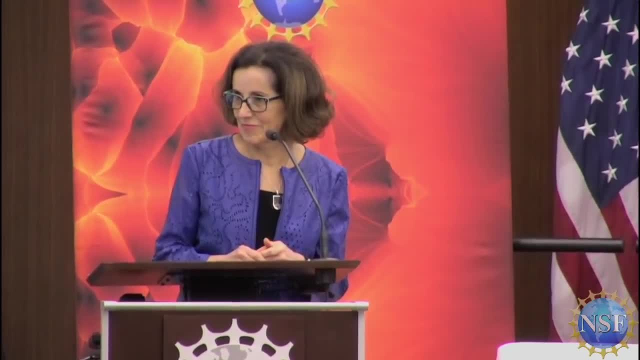 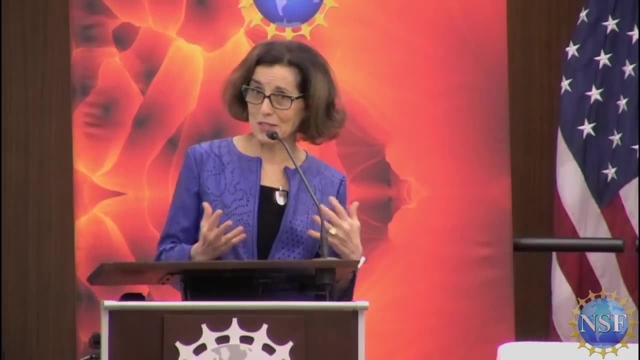 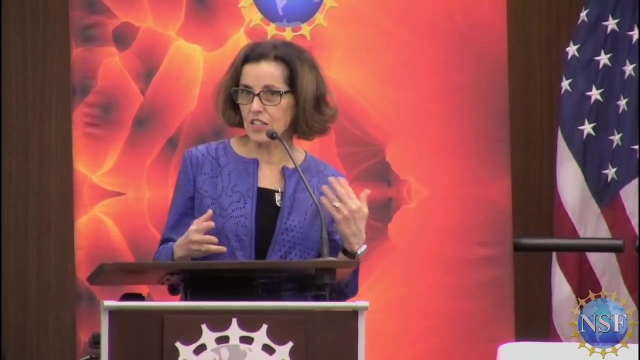 When the funds could support a wide range of smaller yet still impactful efforts. Well, I hope we're investing in both small tabletop experiments and these very large kind of experiments because they can detect different phenomena. But let me ask our observers here their thoughts. 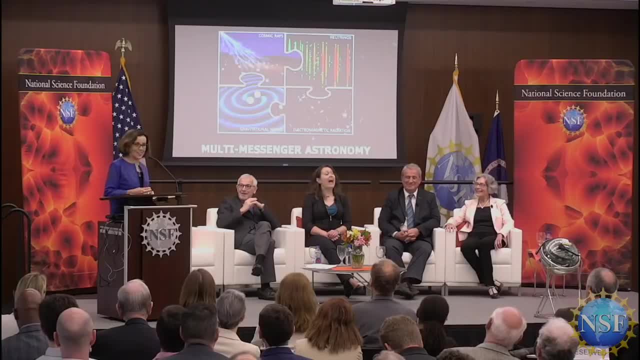 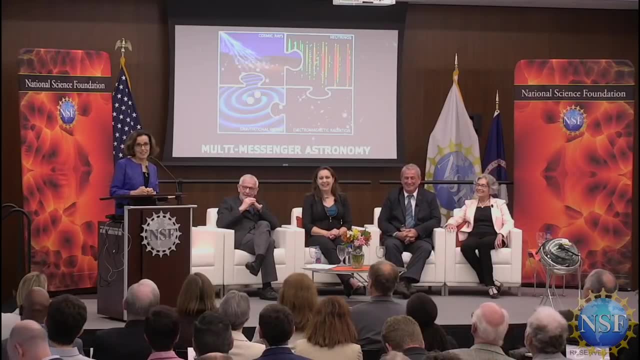 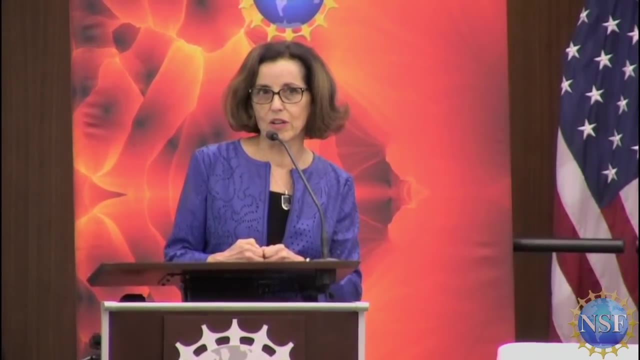 about this question. I think this is your job, OK. All right, OK, So you have a question for the audience. The creativity that is out there is just immense. We recently had a call for information on what people were thinking about doing. 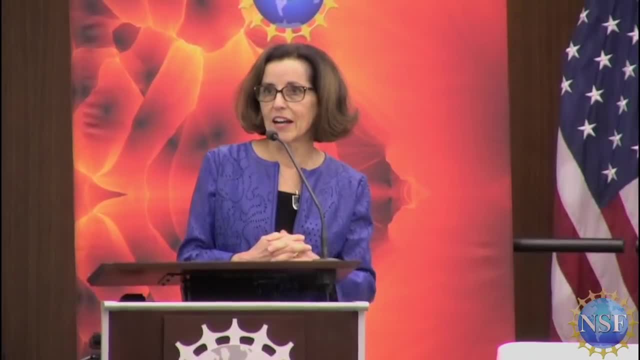 in the smaller line of experiments and we got $10 billion worth of responses to that question of all kinds of imaginative experiments that can be done. So we, just as a group, we have come here as a country, need, need, the will, the imagination to go after that and to to. 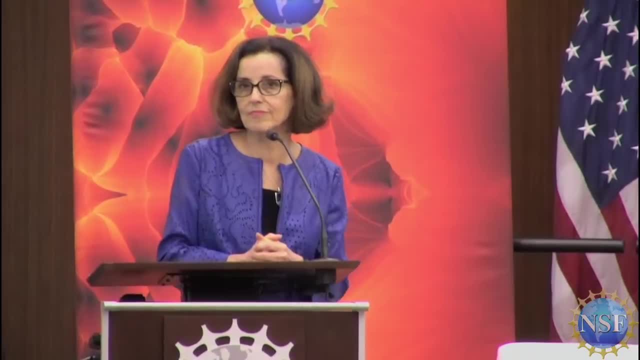 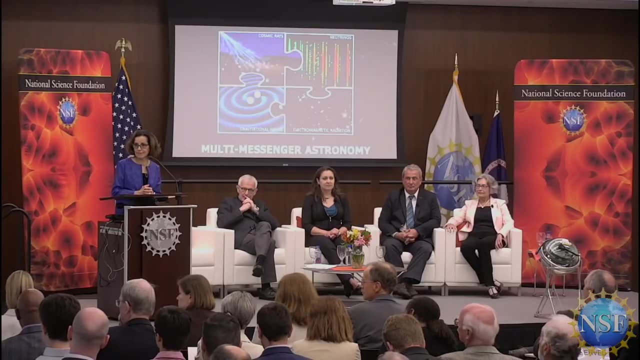 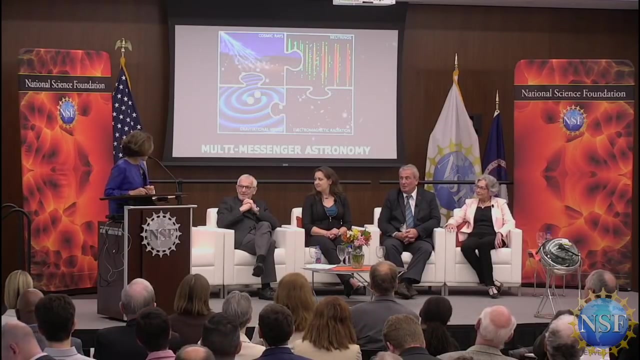 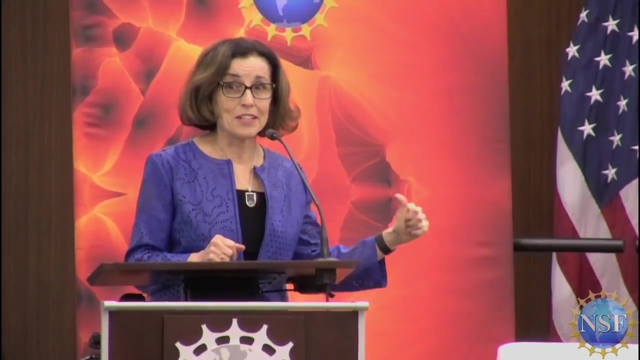 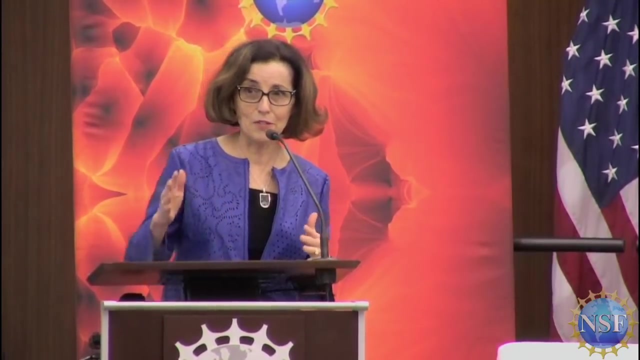 invest in the creativity that's out there. another question: quite simply, why does this research matter? okay, mysteries matter, right? so a lot of us probably started out wanting to be detectives when we were very young, and I know that's what I wanted to be, because mysteries captivate all. how many of you? 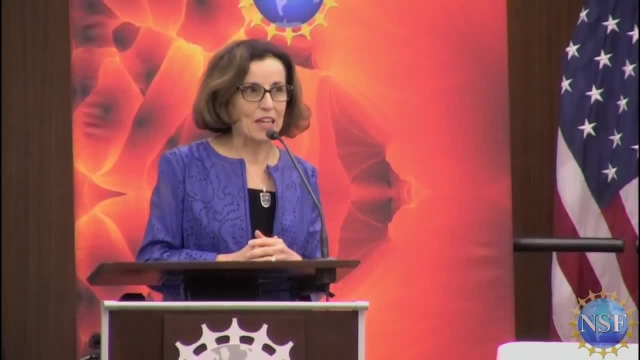 watch mysteries on shows and that's- and this is when you get to mysteries of the cosmos on a grand scale. that's really magic and- and as we've been all talking about our experimenters here- that this is one of the most. this is a mystery that's a hundred and six years old, about 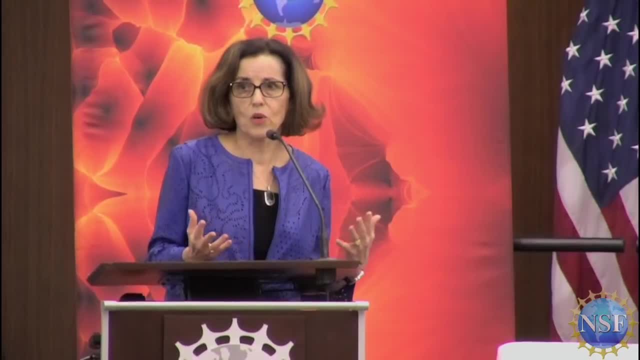 what's the origin of high energy cosmic rays, where? where do they come from? it's just, these are inconceivably high energies, as we've been saying produced, higher energies than we can even produce in these extremely wonderful big accelerators here on earth. and going after those mysteries, whether it's dark, 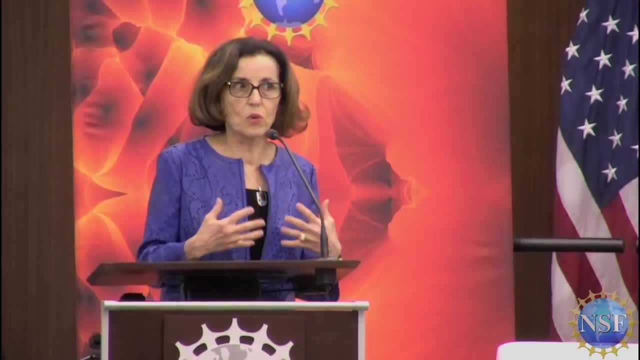 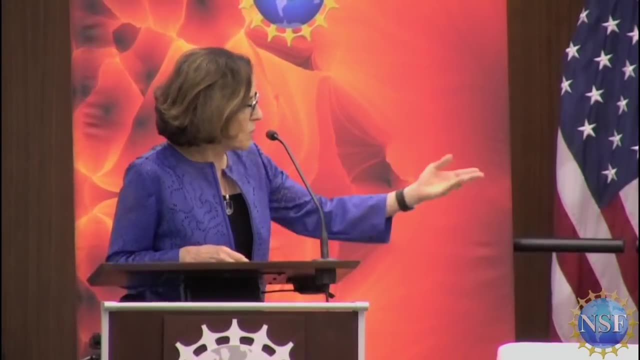 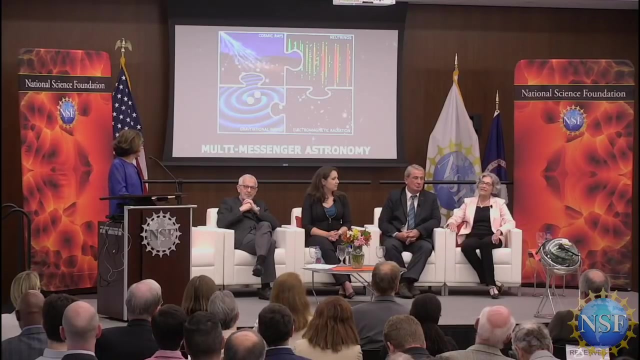 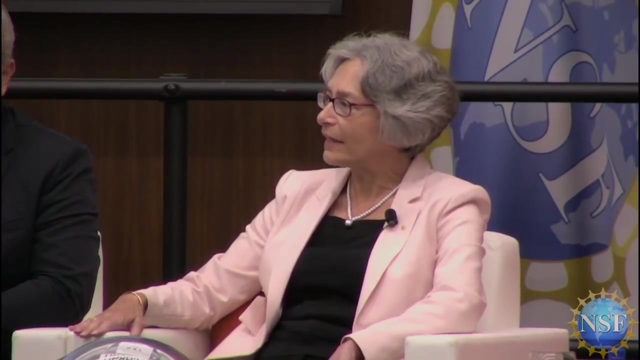 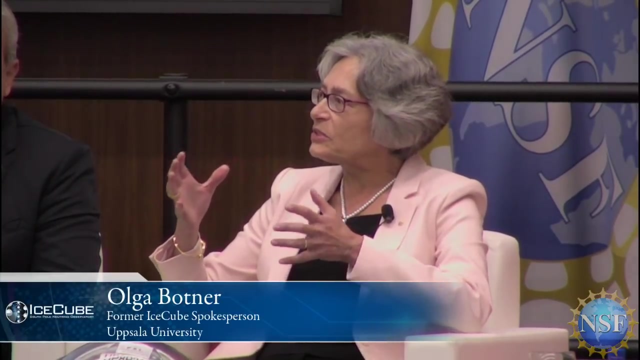 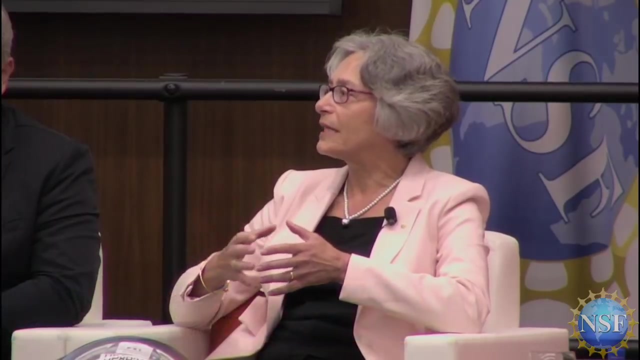 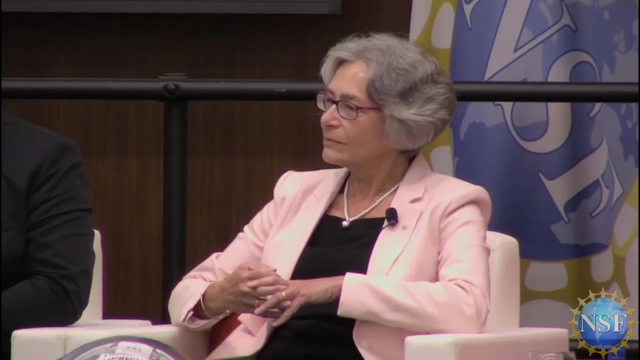 matter. dark energy, the origin of cosmic rays, is what really science is all about is in covering the the mysteries of nature, but use understanding to build the welfare of our societies. I think is a very, very important point behind the science we do. I'd also add: I think it's twofold. 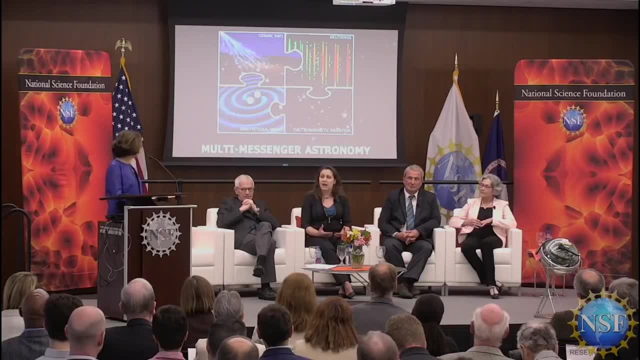 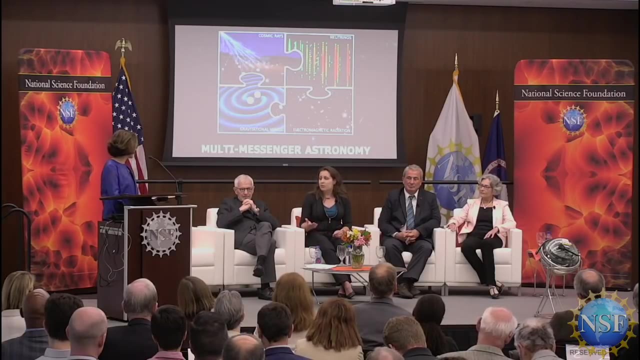 because humans are naturally very curious and we need to ask these questions. but in the pursuit of answering these questions, we develop new technologies. that has applications that we can only begin to understand through their development. when the electron was first discovered, we had no idea we could use it for. 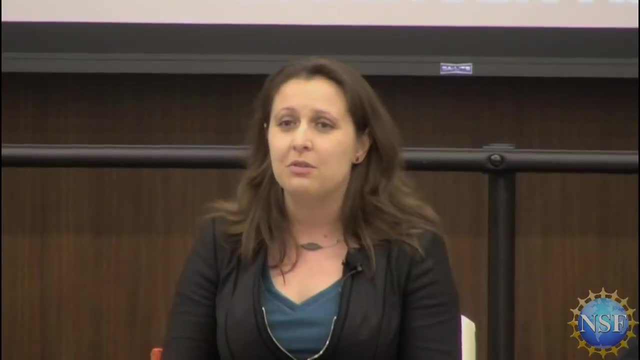 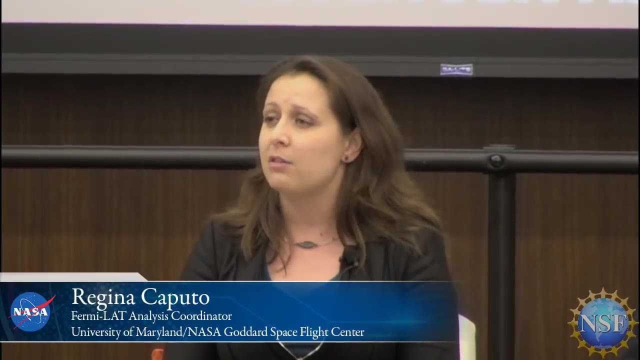 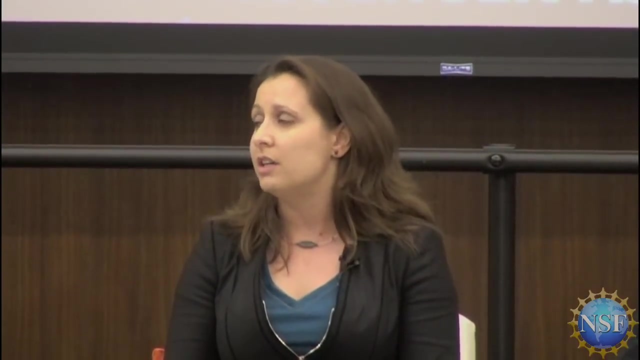 electricity, and that's you know what power is everything that we do. and so I think this even touches back on that initial question of why invest all this money when you could invest smaller amounts. and it's because sometimes the biggest breakthroughs require us to invest a lot in technology to to answer. 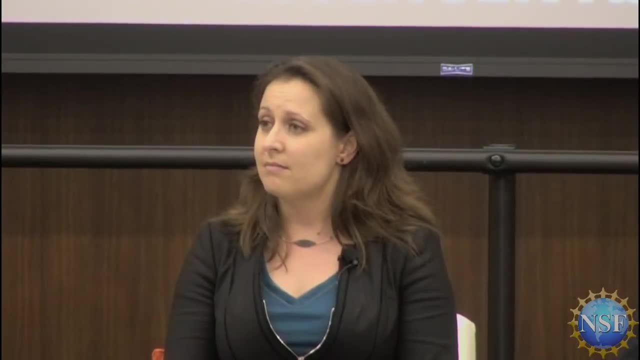 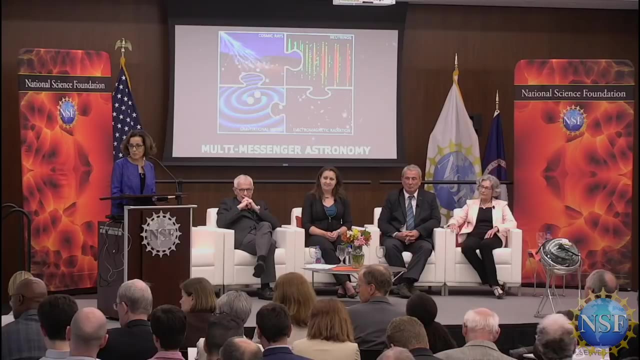 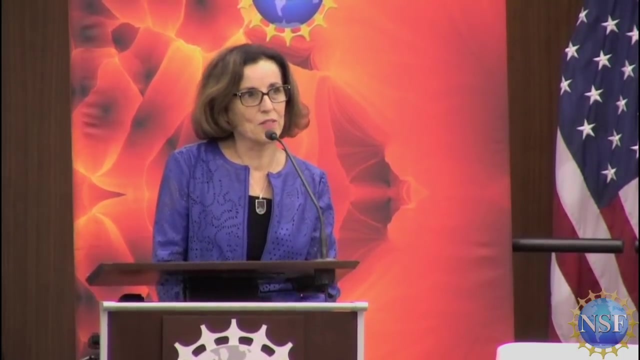 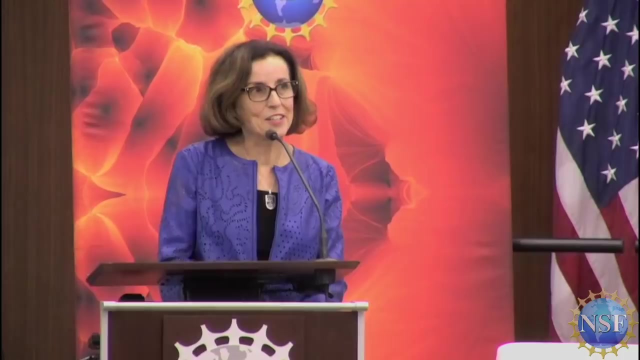 the biggest questions. last question: what does this discovery mean for the future of astrophysics, Multimessenger astrophysics and NSF support for facilities and research? I think this last slide that we have up here is just a perfect way of saying we haven't yet done the ultimate multi messenger detection of using, of bringing. 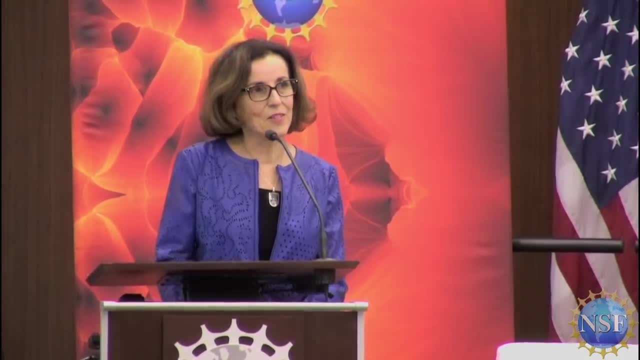 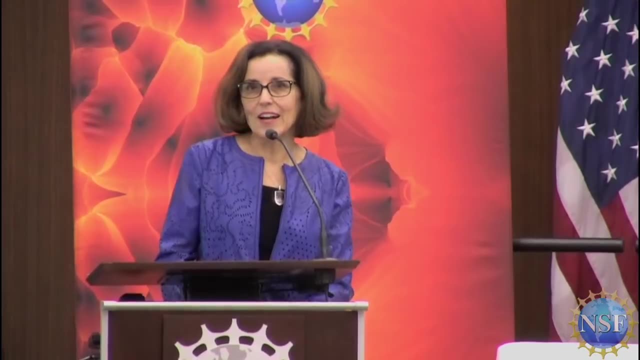 together gravitational background analysis to connect in the future for astrophysics Right gravitational waves and particles and electromagnetic radiation. So we have- we have- exciting work there. The the things that we are discovering, like with the LIGO observations, these some huge black holes and binary systems. 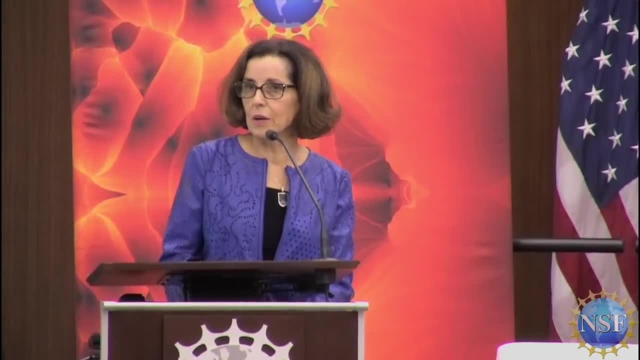 Neutron stars merging, things that were imagined but not witnessed, and so we have a Tremendous amount that we don't yet know about the universe, not only things like blaze, ours- We knew existed and we knew that there were all sorts of mysteries connected with them We hadn't made. 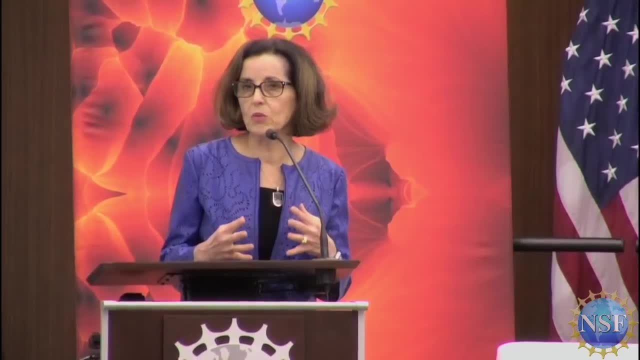 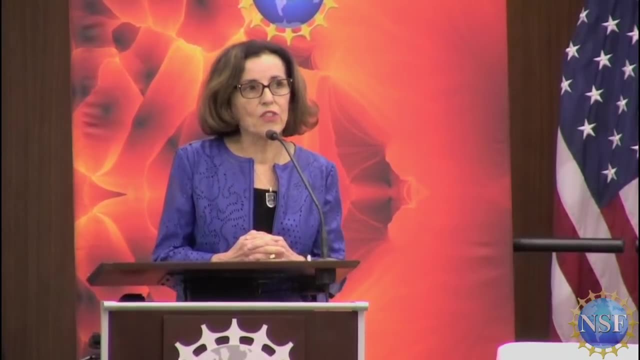 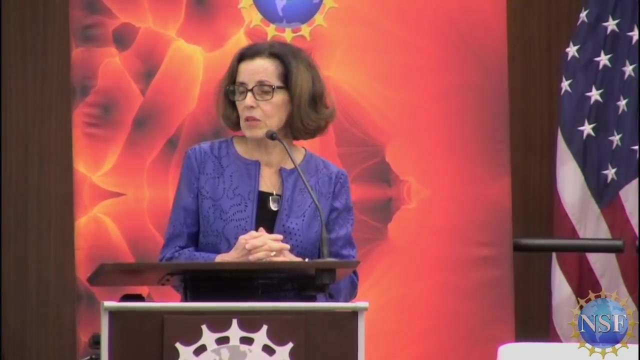 Confirmed the association yet with the cosmic rays and the high-end, High-energy neutrinos, and that's now been done in this announced today. But there are many other things that we out there that we have no idea That that even Existed, as the LIGO observation showed, and so we have just much, much more to discover about our universe and our place in. 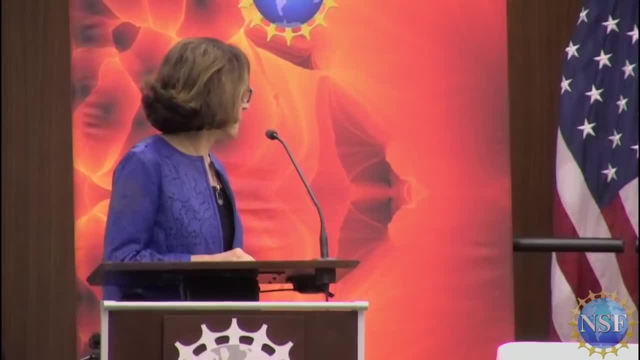 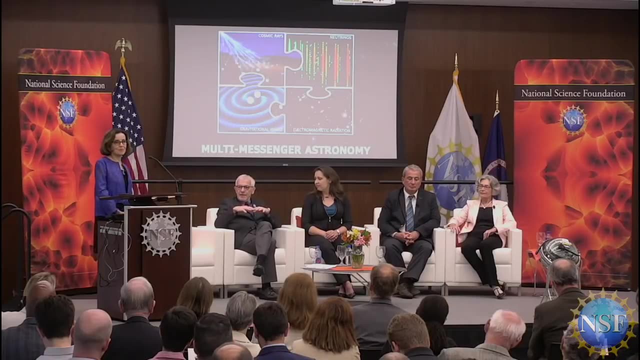 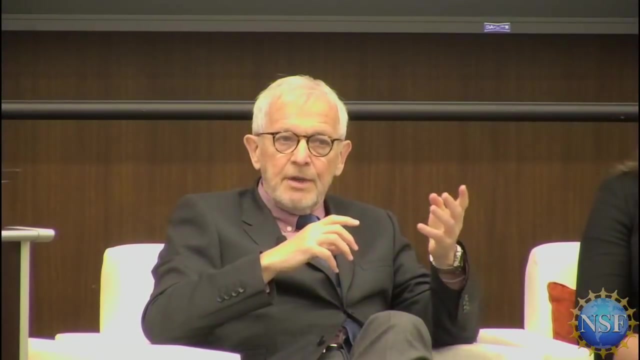 it Again, Francis. Yeah, I, there's something that is rather difficult to explain, But what? and that hasn't been mentioned today. But we learned something from the diffuse flux of neutrinos that were discovered in 2013. in fact, that flux we Detected is very large. 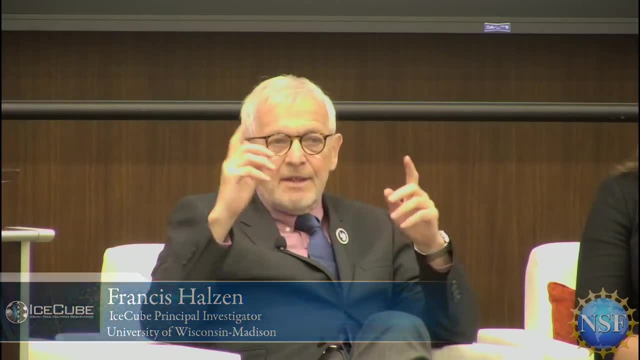 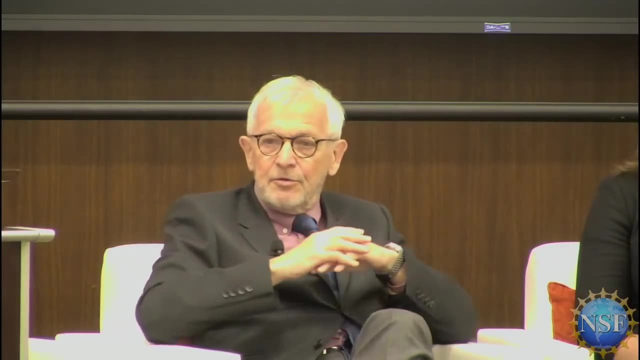 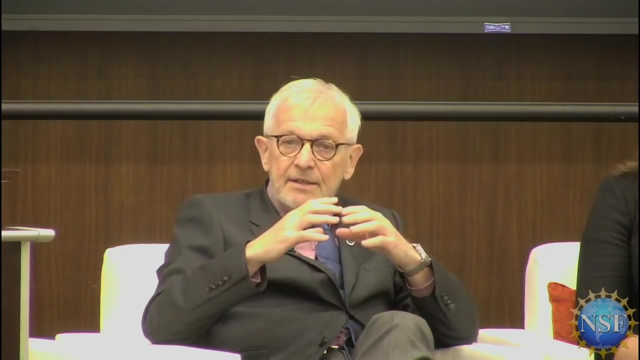 Which is difficult to imagine when you realize it's like one event per month or so. But if you look at the energy density, remember for every neutrino that goes through there are 100,000. We don't go through for the one we catch. So you look at the energy density in the, not in the high-energy universe in neutrinos. 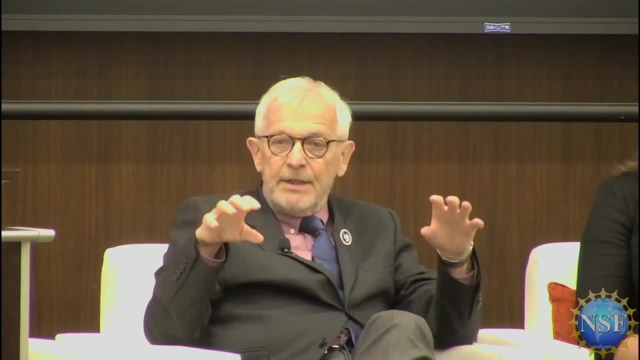 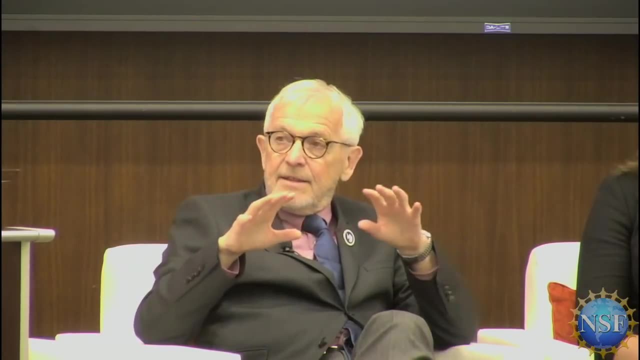 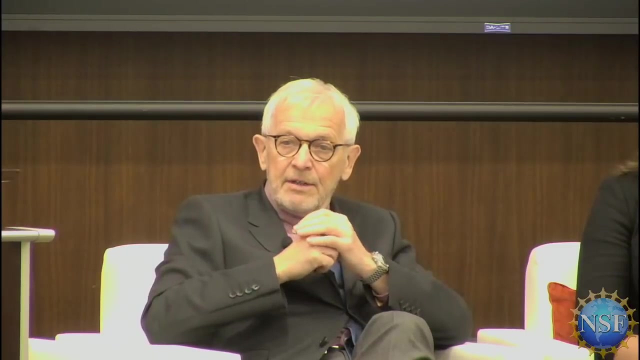 it's roughly the same within a factor as the one in gamma rays and these neutrinos come from proton sources and these neutrinos come from proton sources. so I think this is going to make an impact and a serious rethinking of The way we understand the non thermal universe. 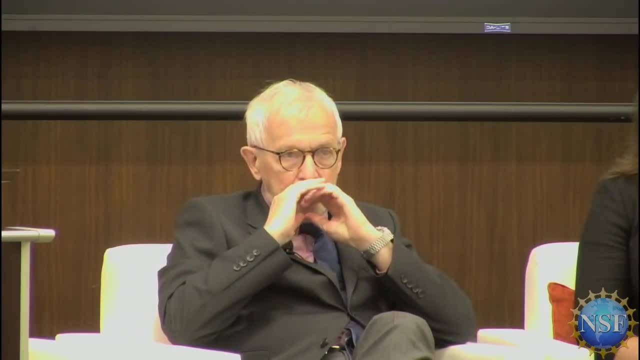 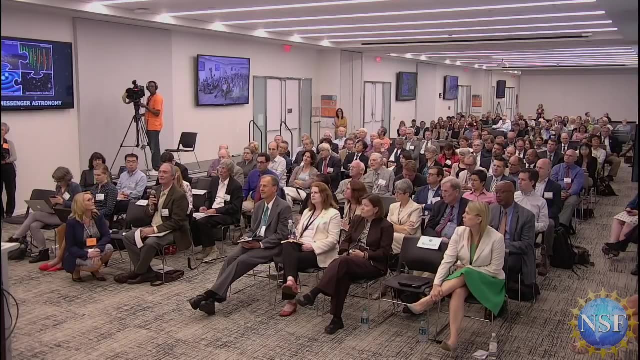 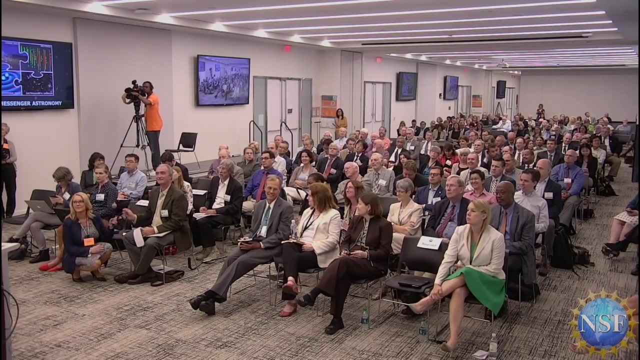 Wait one second for the microphone. Hi, I'm Denis Ollier, a freelance science writer. Are there any other potential messengers out there besides the four that you have up in that package? I guess ones we haven't discovered yet, But nothing in theory, right. 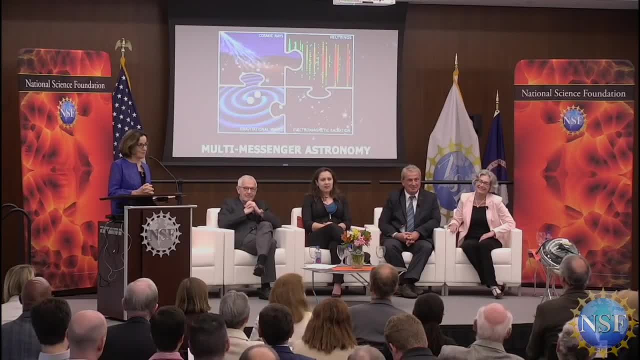 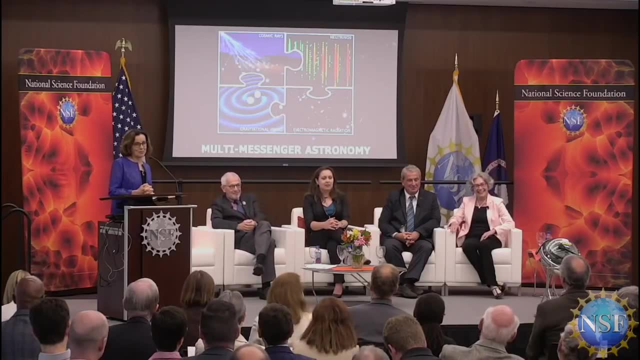 Nothing in current theory right. Dark I mean. I guess the audience is we're pulling the audience now. No, I mean discovering the particle nature of dark matter. I mean that would certainly be another way that we can investigate the universe.